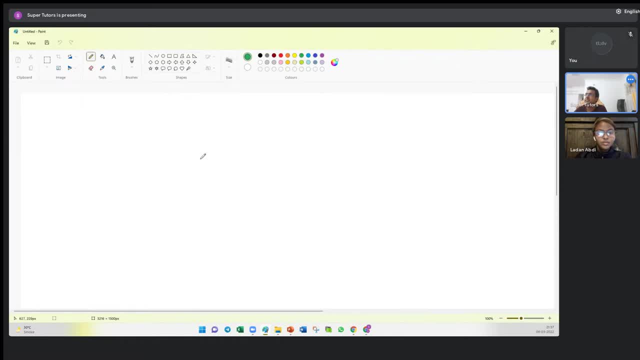 it like this: It's just mu like this, right. So all you do is you write a small u and then you have a little tail on the left, And this refers to population Mean right, Population, mean population average. So if you see on the slide, mu is. 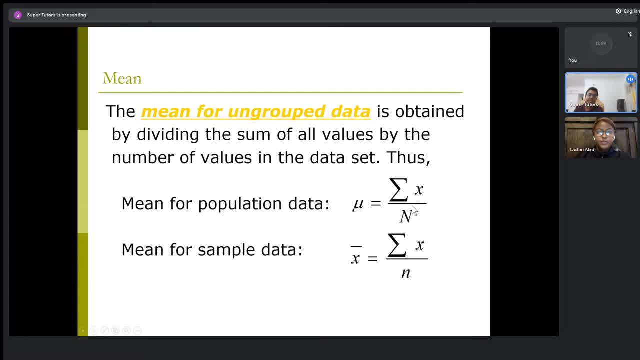 calculated as summation of X divided by capital N. Since you've done chapter one, I would assume that you are comfortable with the summation notation now, right? So summation of X would basically mean all the population parameters just added together and you divide by the. 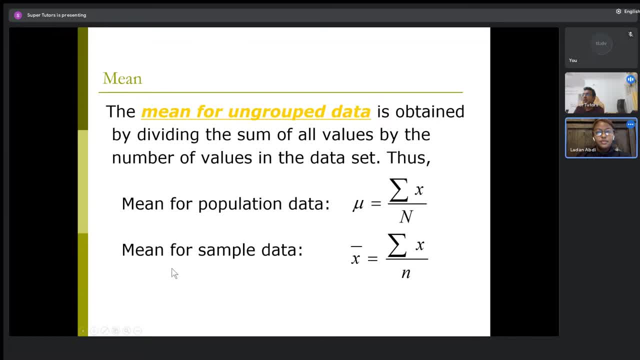 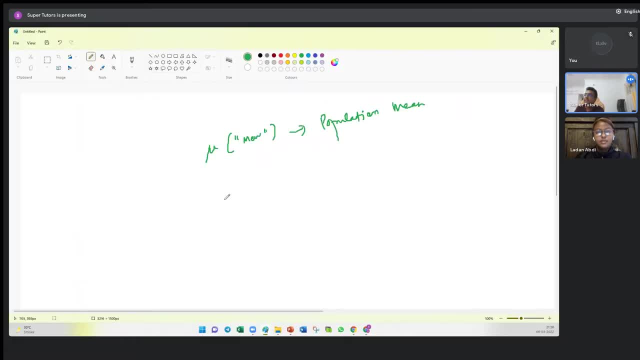 total population size. Simple right Now. mean for sample data essentially is represented by another variable which is called X bar. So it is a little x, lowercase x with a little bar on top- X bar. This is how you read it And basically refers to sample mean Does. 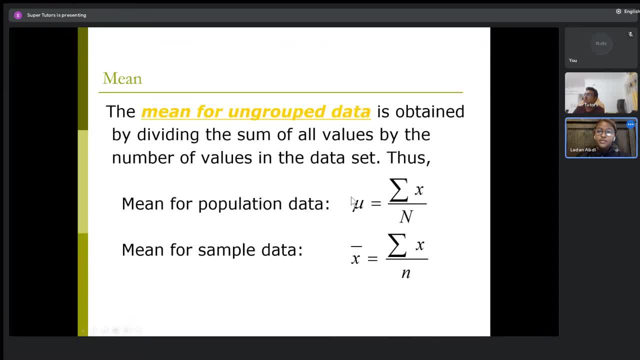 that make sense? Yeah, Right, Yeah, So it is the same formula, essentially: summation of X divided by small n, So capital N for population, because population is generally bigger. Small n for the sample Sample is normally smaller. Sample is smaller, So it's. 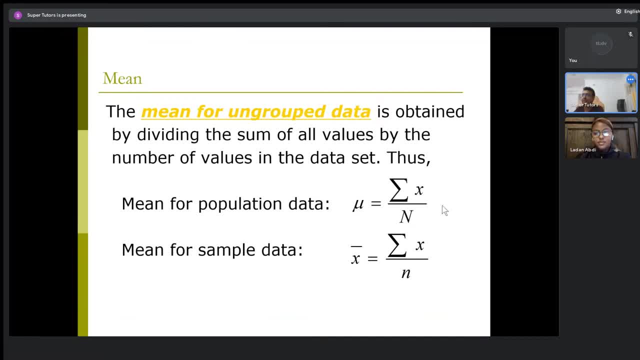 a little x, lowercase x, with a little bar on top X bar. This is how you read it And basically refers to sample mean. Does that make sense? Yeah Right, Yeah, So it is the same formula for sample size. So it's very intuitive if you think about it. So let's. 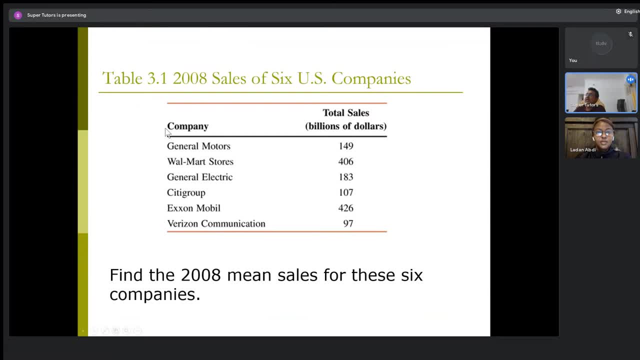 do a quick maths problem, a very simple one, for you. We have the 2008 sales of six American companies: General Motors, Walmart and so on. You have to simply find 2008 mean sales for these six companies. Can you do that? Yeah, just add them all up and divide it by. 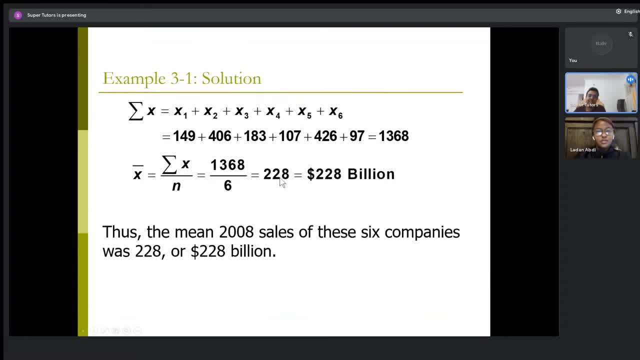 six? Yeah, absolutely, So I trust that you will get the calculation right. It's very straightforward: summation of x and you add all of these up and then x bar is summation of x over n. now question for you here is: why am i saying this is x bar and not mu? because it's sample, and how do you know? 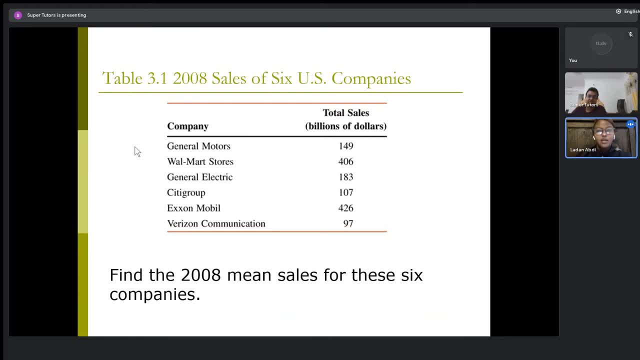 this is a sample, uh, because it's at six, not all companies, yeah, six american companies, and then, of course, there can be like hundreds of american companies, right, so we don't, we can't really say it's a population. similarly, how would you know if it's a population? what would it say? what would 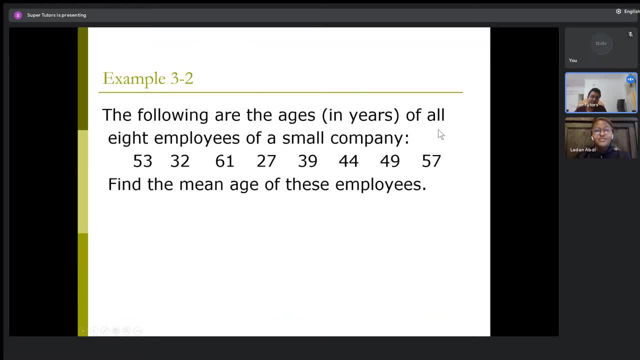 the question. yeah, it would say something like this. so that is the next example for you. so if it says: following are the ages of all eight employees of a small company, this is the population of all employees. so you have to really, you know, impute it from the language of the question. 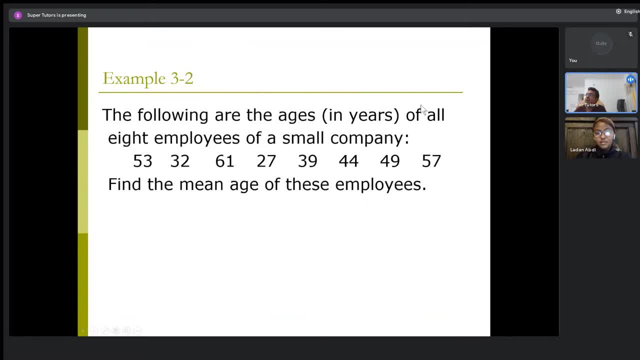 from the wordings of the question, right? so if it uses words like all, it's typically the population and if it doesn't- and you know, looking at the numbers also, you feel that there can be many others in this population. this is just a small subset of what this can be. 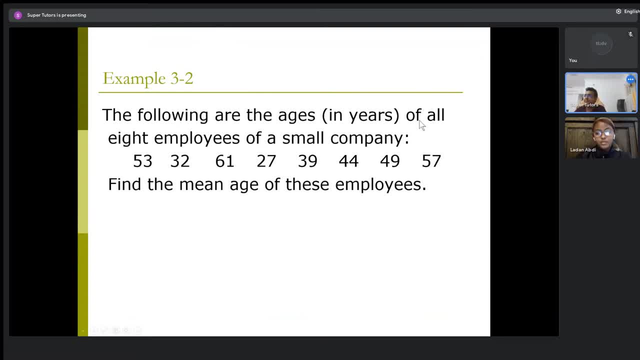 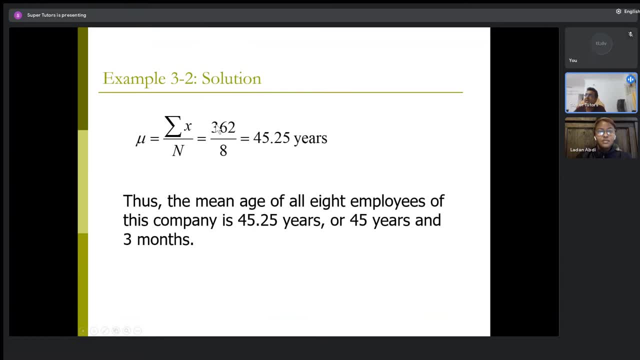 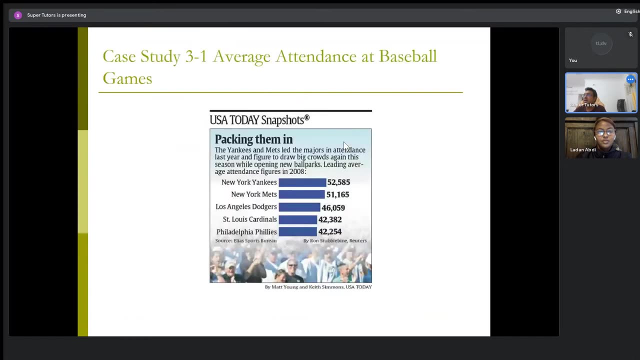 then you typically refer to it as some: okay, make sense. yeah, so mean age of all employees, so mu, and of course the formula is same, so you don't need to really bother about that. 360 divided by it, which is 45.25. okay, now we come to the second kind of metric, which is referred to as median. 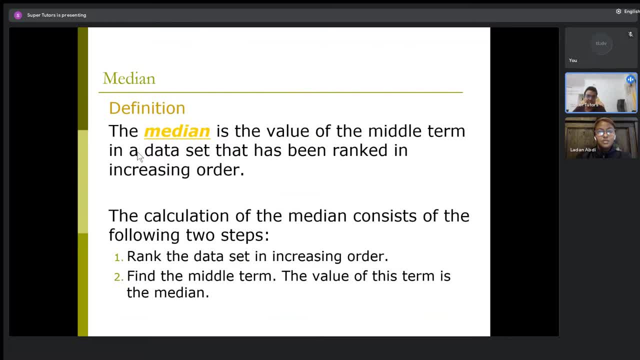 now, this might be new to you if you don't have a background in mathematics, but it's fairly straightforward, i assure you. it is basically the value of the middle term in a data set which is ranked in increasing order, right? so how do we find the median? two, very two simple steps we have highlighted on the slide. 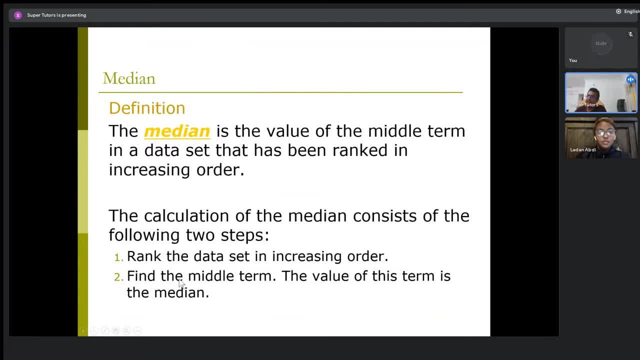 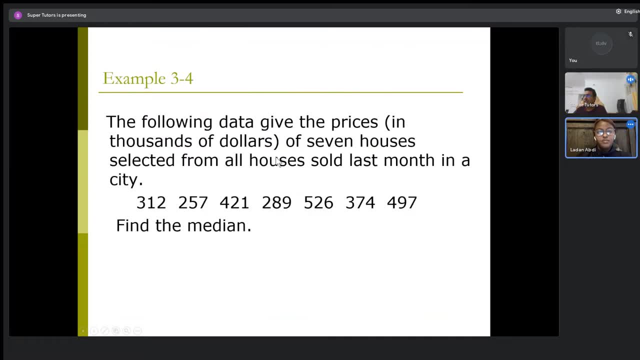 rank the data set in increasing order and then you find the middle term. the value of this term is the median. it is as simple as that. yeah, okay, right, yeah. so let's say, i have seven house, right, and i have the price of seven houses in thousands of dollars. so, for example, 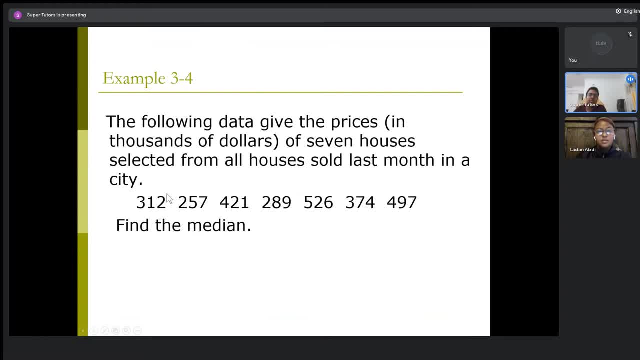 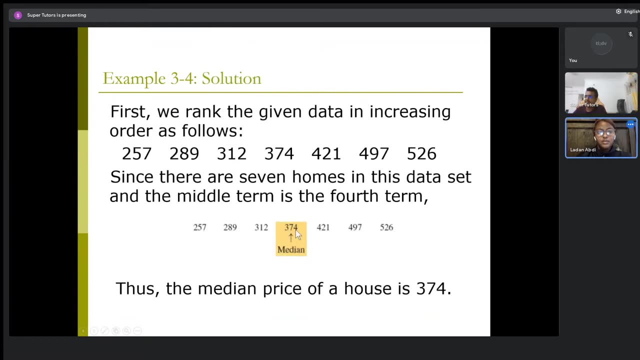 this is the price of the first house: three hundred and twelfth thousand dollars. i have the second house, 257 000, and so on. question is: find the median. how will we do it? we will increase in order. yeah, so if you see this is in random order, right, i have a bigger number, then a smaller number, so in a particular order. i hurry woi, so in a particular Потому. that's quickly. 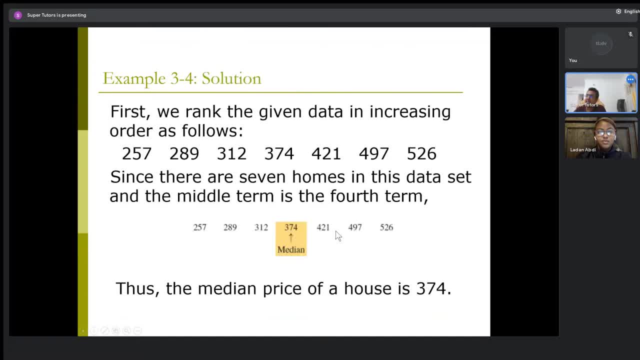 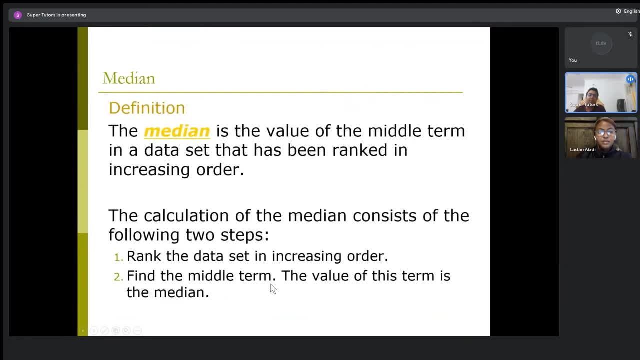 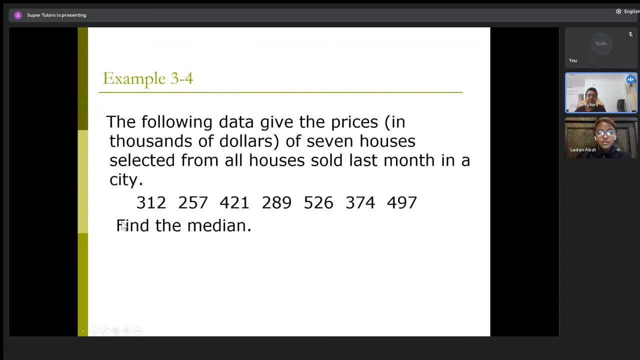 and then a even bigger number, and so on. so i arrange it like this, in increasing order. this is an increasing order, if you see. yeah, and then what's the second step? simply find the middle term. now, if i have seven terms, which one will be the middle term? think and answer. 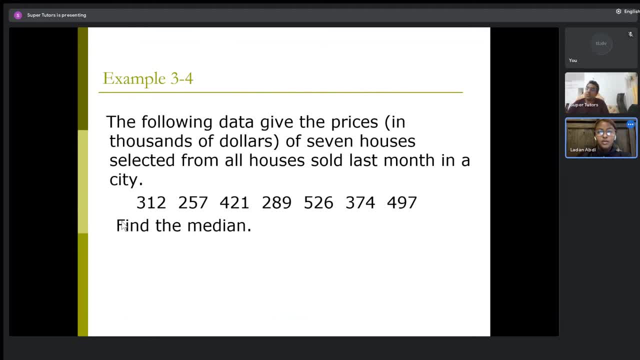 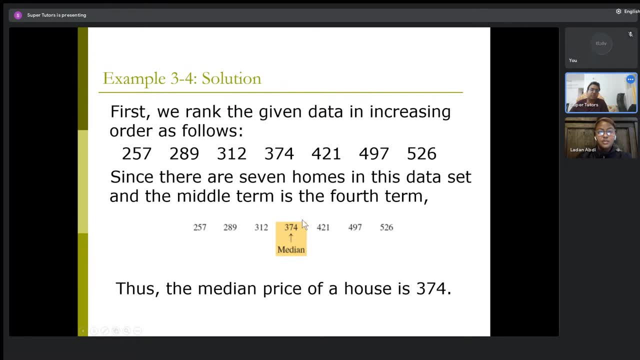 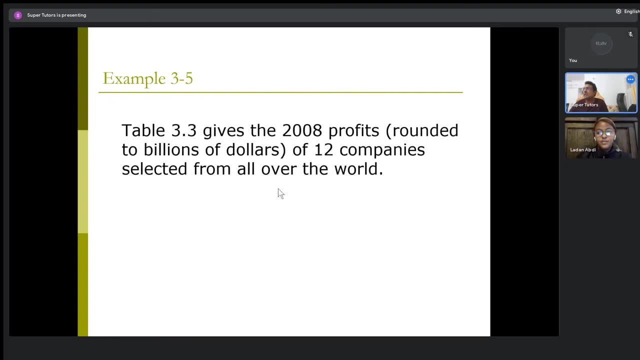 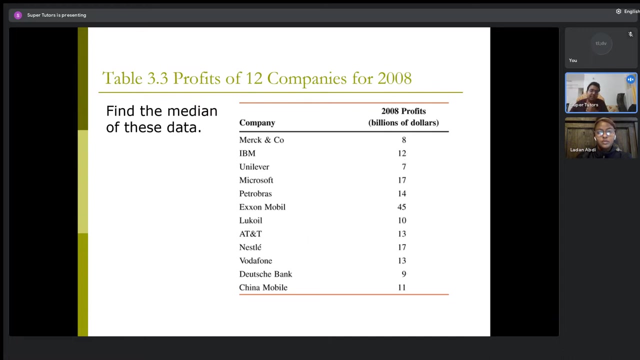 uh, one, two, three, the fourth, one, fourth term, absolutely correct. so all i would do is i would arrange it first and then grab the fourth term, which becomes my median. okay, is it straightforward? yeah, now the problem arises when i have an even number of numbers, because if you look at any sort of a combination of even numbers, let's say, if i have seven, nine, 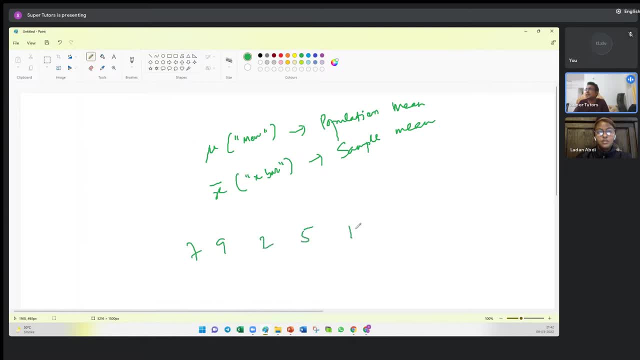 two, five, uh, eleven and let's say ten. so how many numbers do you see on my screen? six numbers. now, when there is an even number of numbers, which is six, in this case, there is no single middle term, but there are two middle terms, if you see. 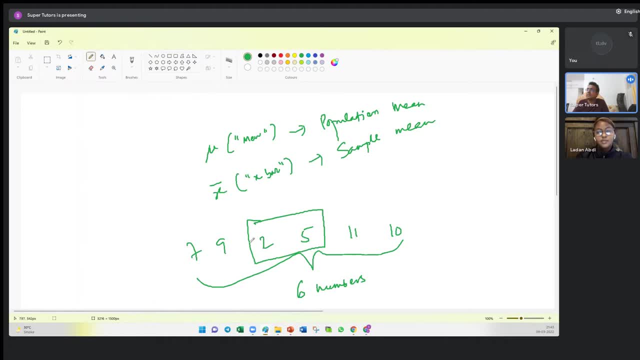 right, because i have two numbers here. i have two numbers here and two in the middle. if you have an odd number, like in our example, then of course the seventh for seven terms. for example, you have one middle term, so you just grab that. but the question is, what do you do when there's 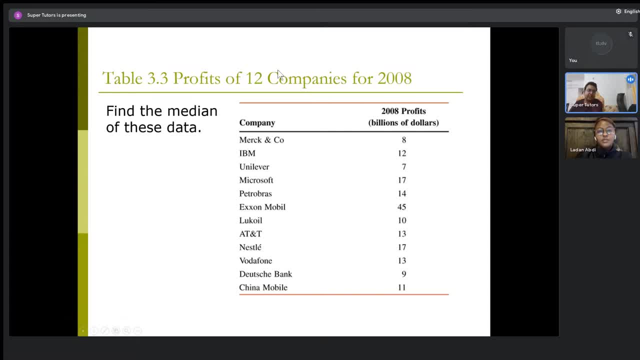 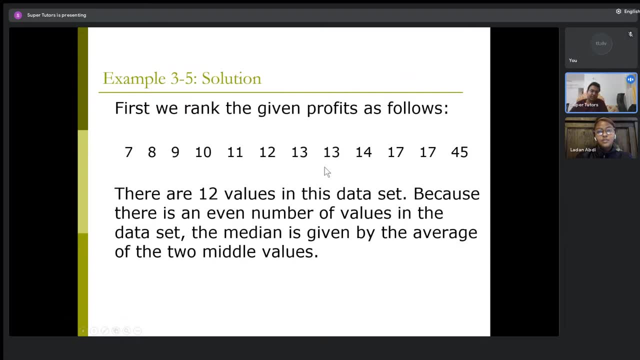 an even number of numbers. so i have 12 companies here. 12 is an even number, yeah right. so again i will have two middle terms. so what do you do in such cases? fairly straightforward, you first step is the same. you first rank them in increasing order, like this, and then you grab the middle two. 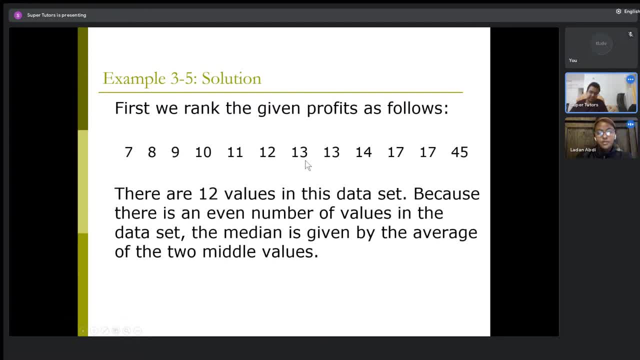 terms and take the average right. so for 12 values, if you think about it, the six middle terms are the sixth and the seventh value will be the middle two terms. yeah, because sixth will be after five terms and after seventh term there will be another five terms. so you grab the middle two, 12 and 13. 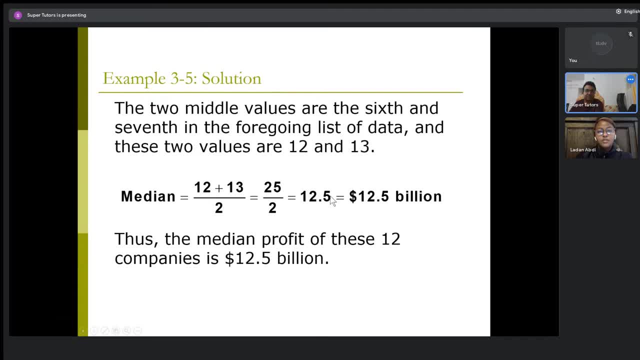 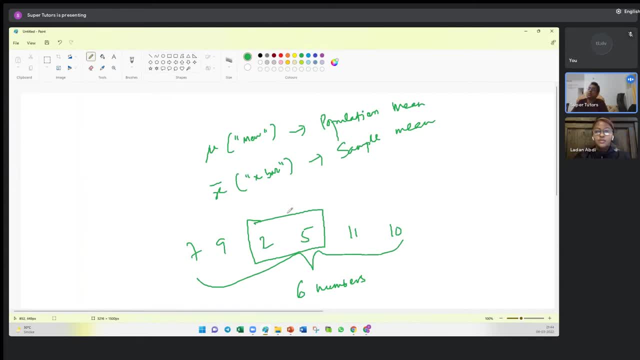 take the average and that's your median boiler. okay, right, yeah, yeah, but how do we quickly determine which are the two middle terms? so for that you can use a simple way to remember it: it is n by 2th term plus n by 2 plus 1th term, and this whole thing divided by 2, the average of these. 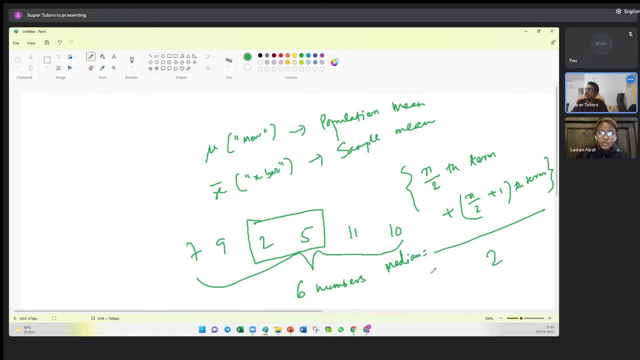 three are these two. so this is your median, where n is nothing but total number of terms. so if n is six, like six term terms, on this example, the n by 2th term would mean 6 divided by 2th term, which is third term, if that makes sense. 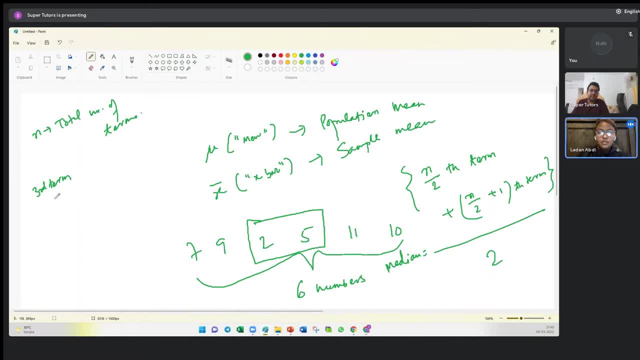 six by two is six. uh, six by two is three. yeah, and what did i say is the other term, n by two plus one x term. so if n by two is three and three plus one, is how much? four, four, so third term plus plus fourth term divided by two. so you take the average of these two. 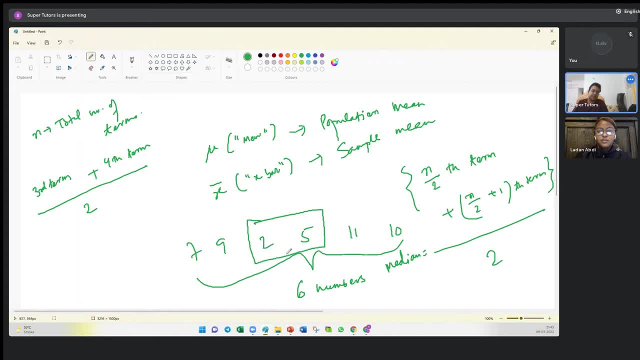 just for you to quickly find out which are the middle two terms, because i can use the other method as well. right, the other method is the same thing. i'm just like giving you a more concrete formula here, just to quickly identify the middle two terms. okay, because- and over two, if you have like 12 terms here. 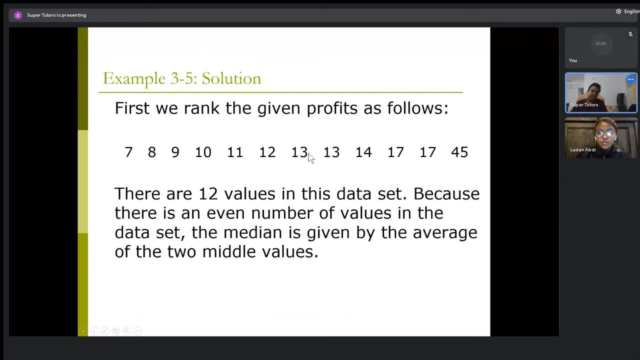 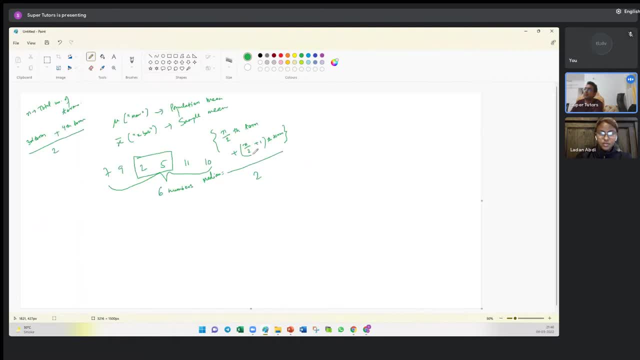 you will take a minute to figure out that these are the two middle terms. but if you have the formula n by two plus n by uh and the average of the n by two plus one x term, so for 12, how much is 12 divided by two? 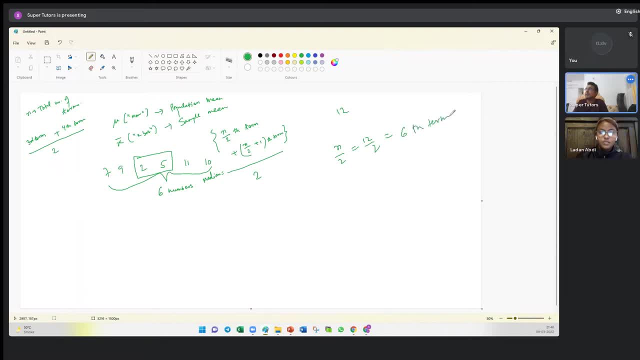 six, six, so six term, and n by two plus one x term. so how much is six plus one? seven, seven, seven. so you see how it becomes easy to find that which terms am i looking for? because when you have like 100 terms or, let's say, 104 terms, right then sit in your exam and 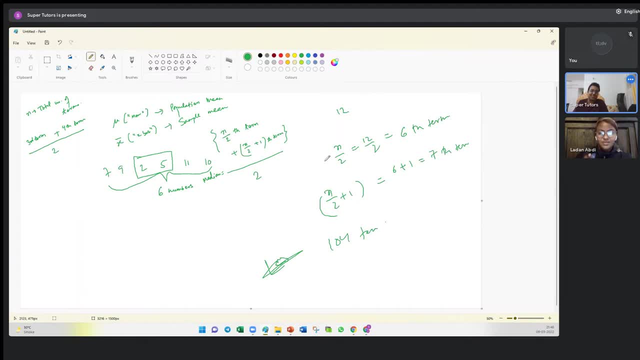 count as to which are the middle two terms or will you be smart and use this formula? yeah, formula make sense. yes, so it's n over two, yeah, and over two x term. if you look at the formula here, if my, if you want, i can zoom in, so you have to basically take the. 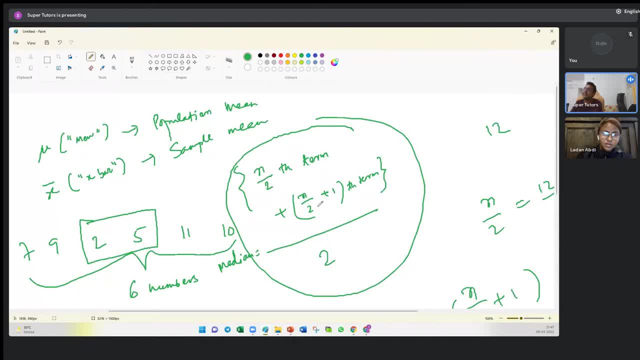 average of the n by 2th term and the and the next term. basically so n by 2 plus one x term, that's your median when n is even. if that makes sense, don't need to jot down anything. you will have the recording so you can like. 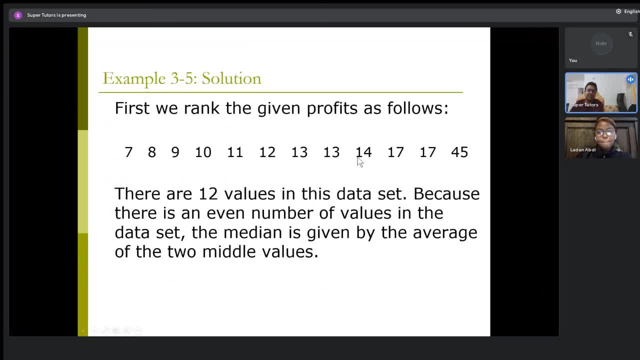 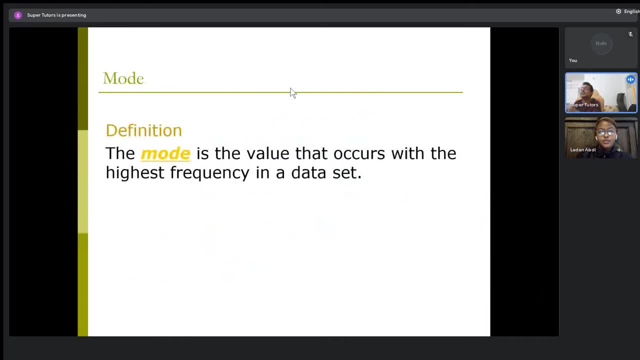 you know? look at the discussion again. is it clear? is it fairly straightforward? yes, yeah. now the third measure of central tendency is called mode. so mode is basically a value that occurs with the highest frequency in a data set, the most frequently occurring value. so that is what we refer to as the 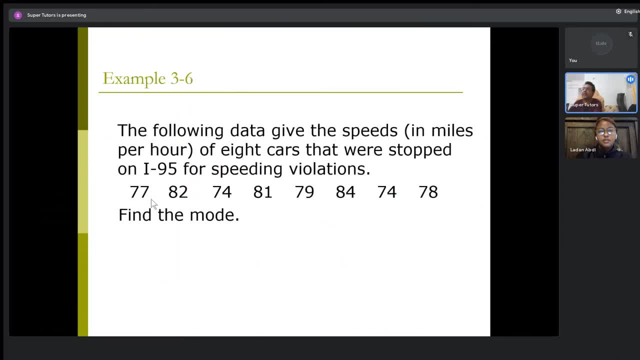 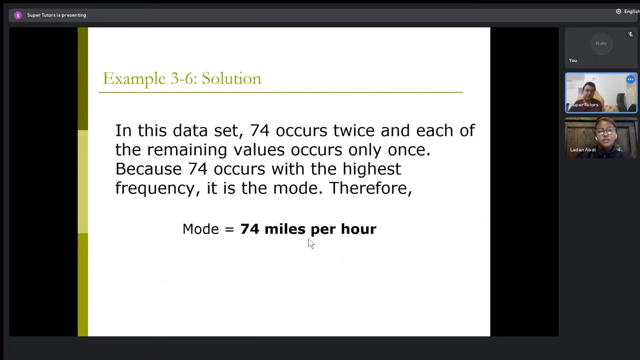 code. so here, which value do you find is recurring the most? uh, 74, absolutely, because everything else is very, very unique. you have 178, 184, 181, 179 and so on, but you have 74 repeating twice, so the mode is 74, if that makes sense. 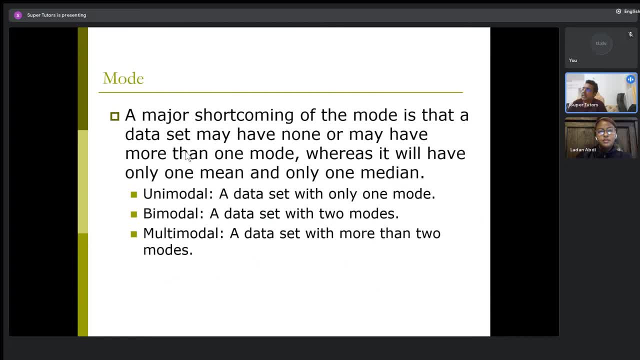 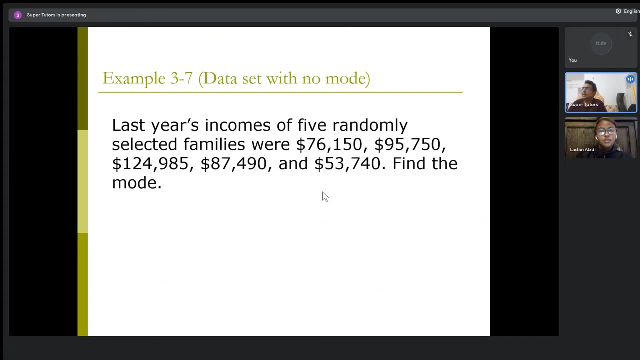 now you can say that a data set is having only one mode and it's called a unimodal data set. a data set with two modes is called bimodal and a data set with more than two modes is called multi model. right, yes, so can you find the mode here? 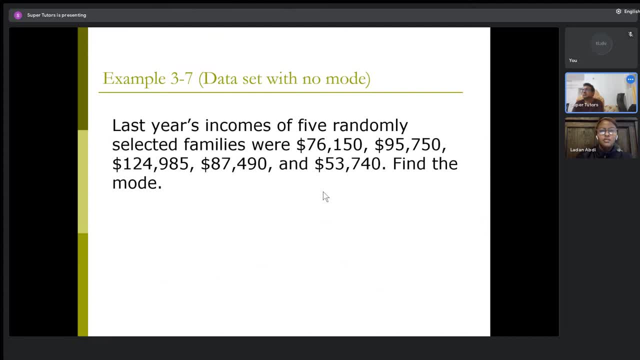 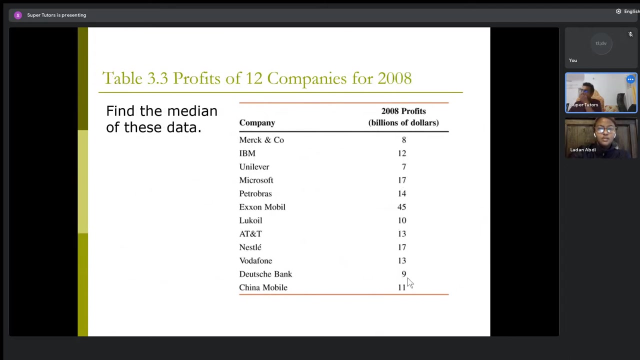 I don't see why. I don't see why? um, I don't see one. yeah, absolutely perfect. there is no mode, as you rightly mentioned, because all the values are unique. how about the previous example about the mean? can you find the mode here? which are the most frequently occurring values or value? 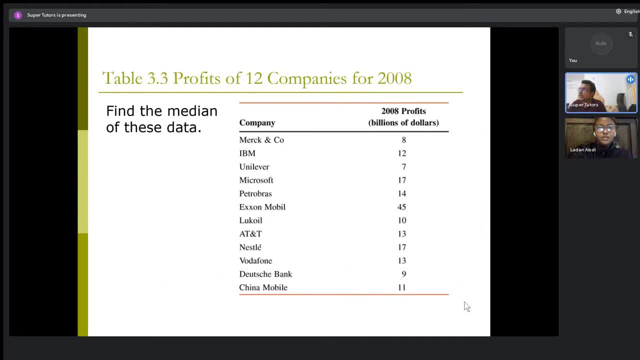 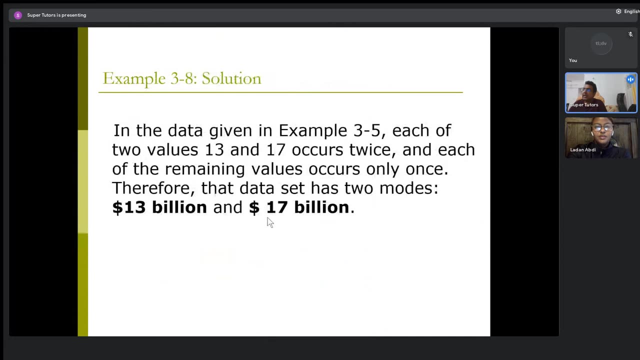 None. So, if you look at it, there are two 13s. Oh yeah, here yeah, two, And there are two 17s as well. Oh, okay, yeah. So basically there are two modes here: 13 and 17.. 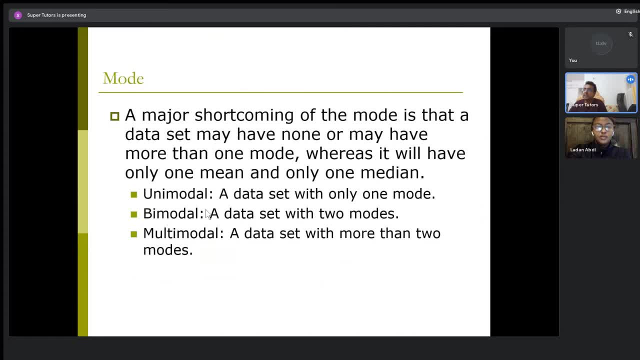 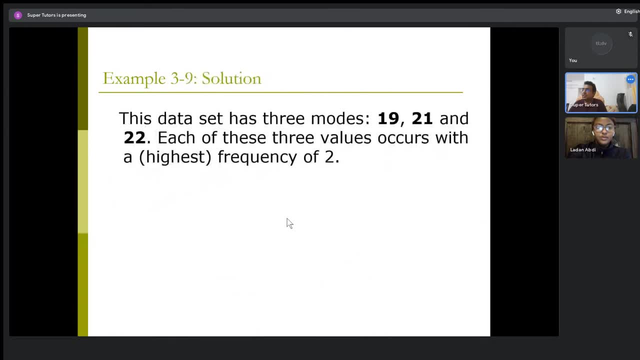 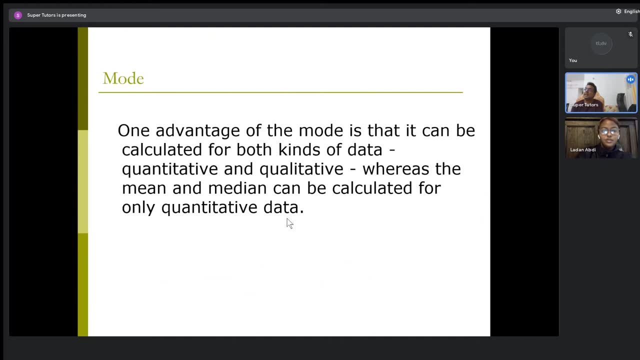 And since there are two modes, there are two numbers which are both mode. this is a bimodal data. bimodal data set right. So mode is clear. Is it fairly straightforward as well? Yes, Now, one beautiful advantage of mode is that. 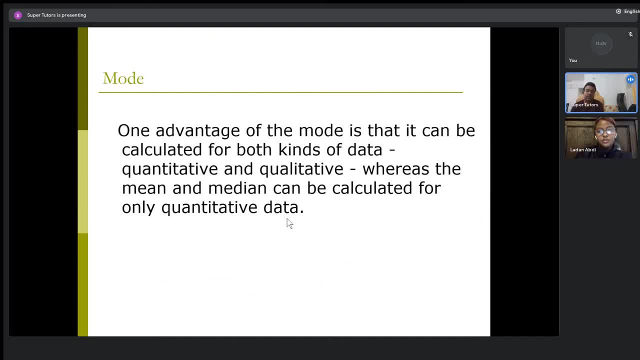 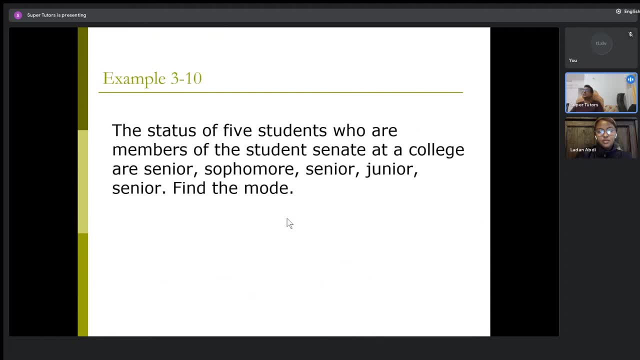 it can be calculated for both kinds of data, quantitative as well as qualitative. So when you talk about qualitative data, this is how the data will look like. There are no numbers involved. It's just a qualitative data with a qualitative understanding of data. 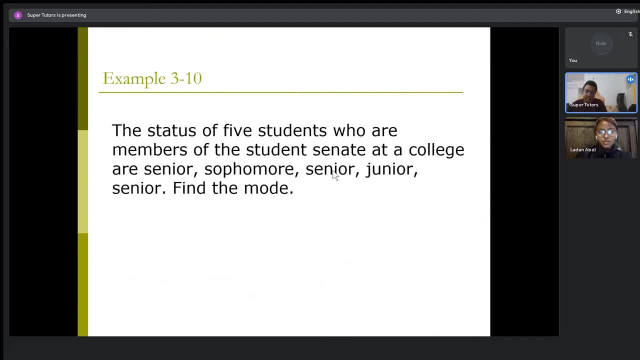 Now, what's the mode here? Any ideas? I've seen here Absolutely, because senior is repeated multiple times whereas the others are not. So this is one big advantage of using mode, that it can be calculated for this kind of data also. 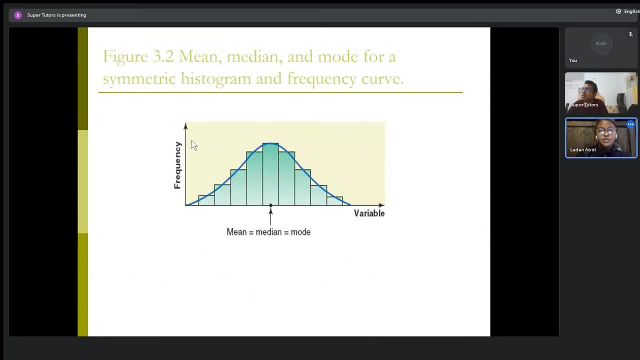 Oh yeah, okay, Yes Now. relationship between mean, median and mode. So for a symmetric histogram which looks like this: the three are equal to each other And the three are equal to this value of the variable, the central value. 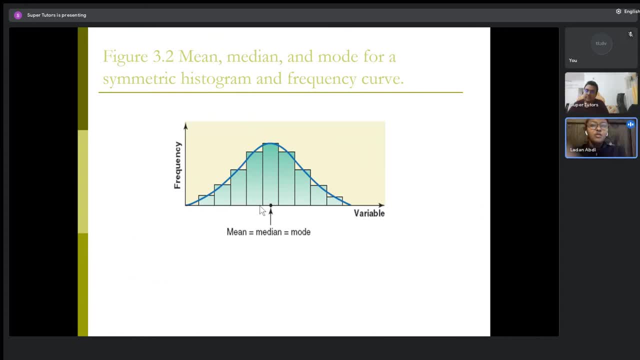 Oh, okay, I read the book and I was a little bit confused about how they're all equal. Yeah, because it's symmetric. That's the reason that they're equal. Okay, Simple. Now, when you have something which is skewed, 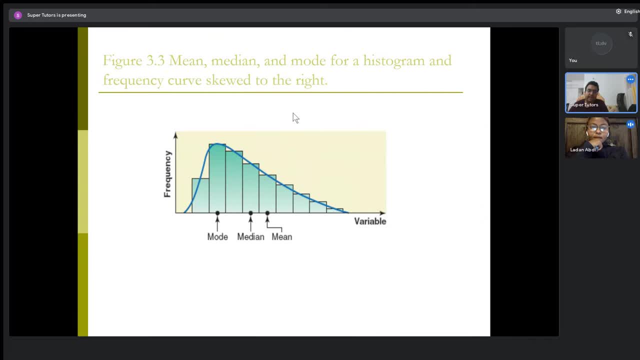 can you tell me whether this is skewed to the right or the left? The right Absolutely, because you have smaller bars on this side, as we learned earlier right. So in this case, the mean is actually greater than the median, which in turn is greater than the mode. 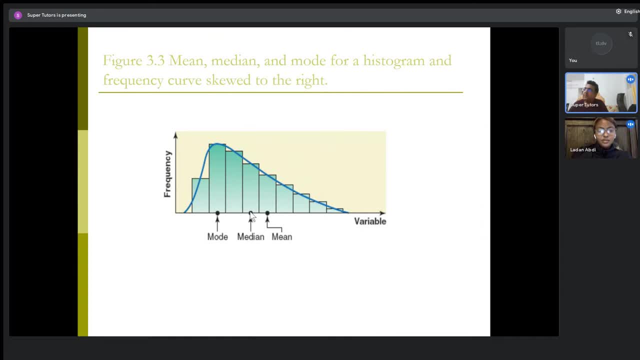 If you see, the mode is the leftmost, then comes the median, then comes the mean. If it's the other way around, if it's a left, then it's a right. If it's the other way around, if it's a left, then it's a right. 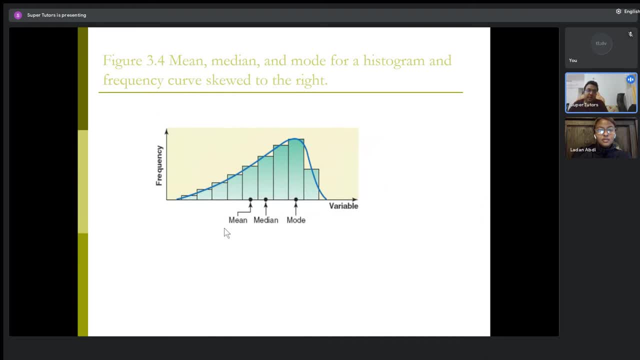 If it's skewed, then the relationship is also reverse. Now the mean is the smallest, the median is in the center and the mode is the largest. That's always the case. That's always the case for something which is skewed to the left. 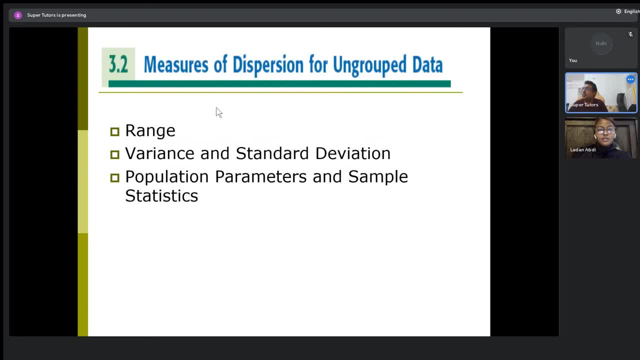 Okay, Right, Measures of dispersion. Now we have three different metrics- range, variance and standard deviation- for measuring dispersion. Till now, we were focusing on measures of central tendency. Centrally, how does the data look? So mean is like a central measure. 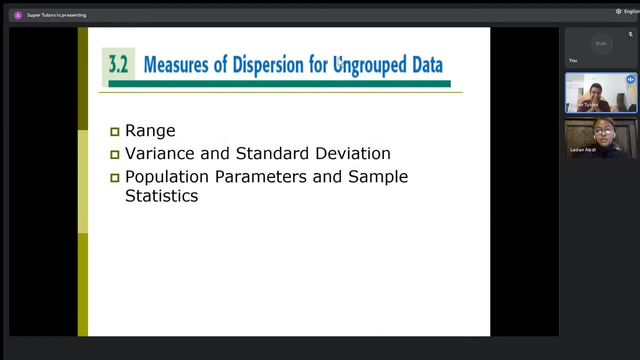 the average of all numbers And then the standard deviation tells you how far are the values spread around the mean, the other values, right? So the first one is the simplest and is the least used these days. It's not very important these days. 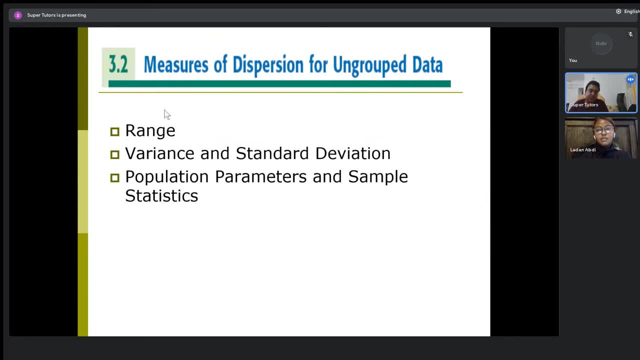 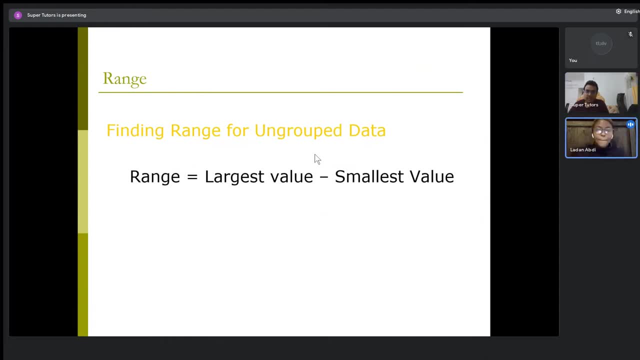 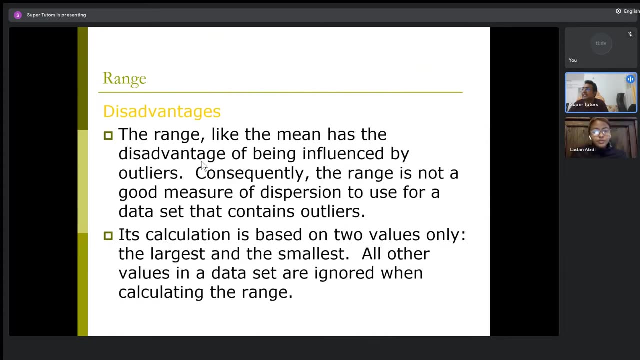 in our normal industrial standards It's called the range, And the range is very simple: It is the largest value in the data set minus the smallest value. That's it Okay, But the problem with range is it has the disadvantage of being influenced by outliers. 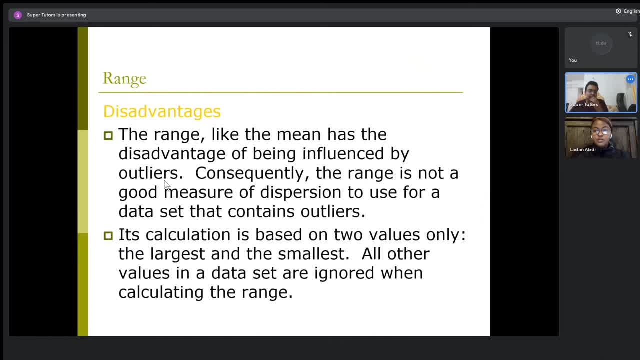 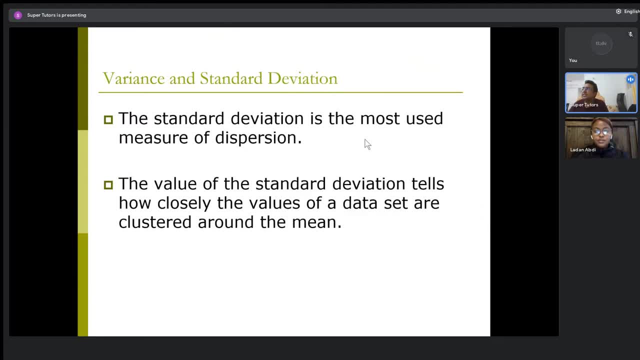 So if there are two big or two small values, then the range will be influenced by that, But does not give you a good picture of what the rest of the data looks like. So what we look at is essentially called a standard deviation, As you see on the slide, standard deviation. 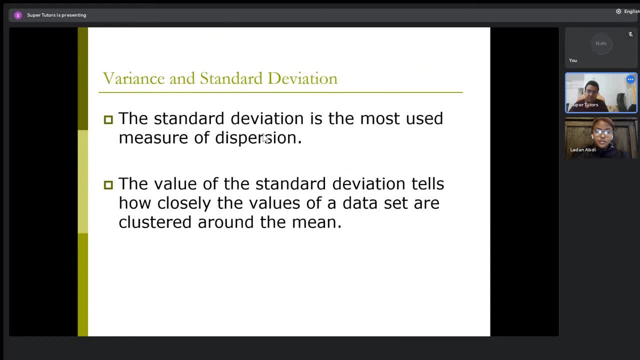 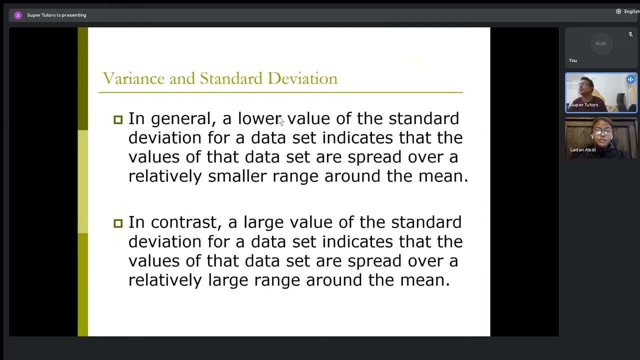 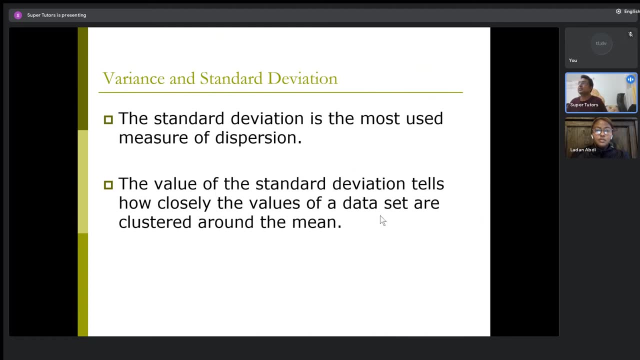 is the most used measure of dispersion. So, of course, lower value of the standard deviation. Yeah, So value of the standard deviation, as I was just saying, tells how closely the values of data are clustered around the mean. If the standard deviation is low, 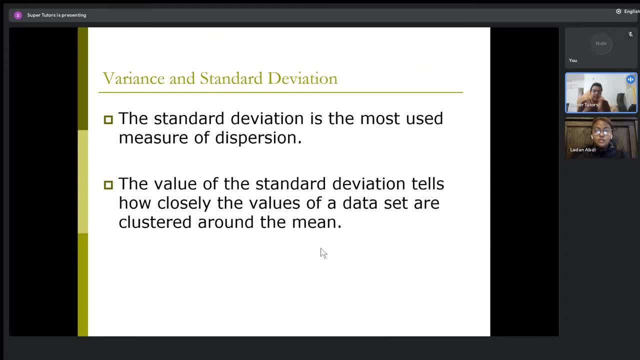 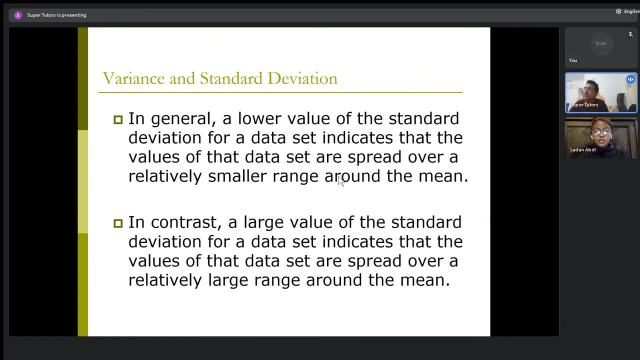 then the distribution is tighter around the mean. The values are very close to the mean, the other values. If the standard deviation is too high, the values are farther apart from the. as simple as that. okay. lower value of standard deviation indicates that the values of the data set are spread over a relatively small range. 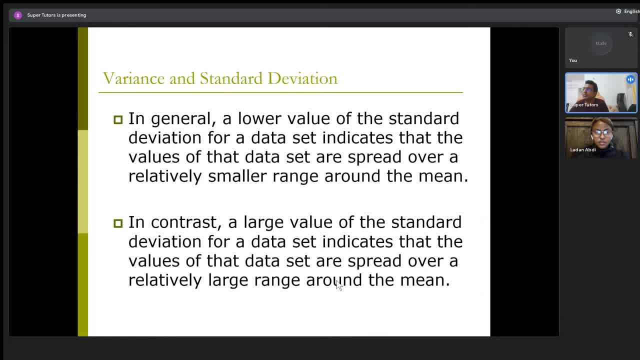 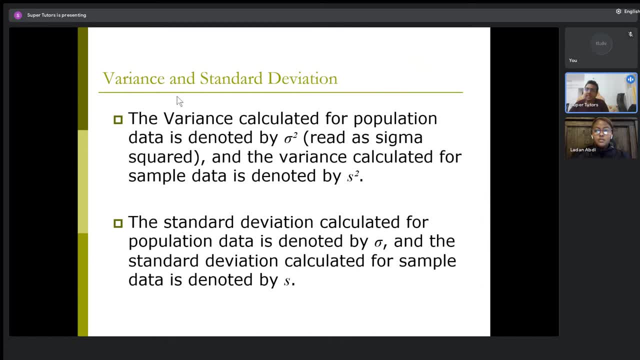 and a large value of standard deviation indicates that the values are spread out over a large range. as we just noted, now there is something called variance. variance is nothing but the square of the standard deviation. so the standard deviation is two units, the variance is four. if the standard 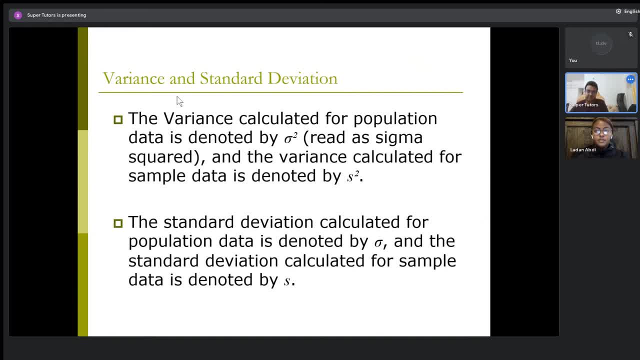 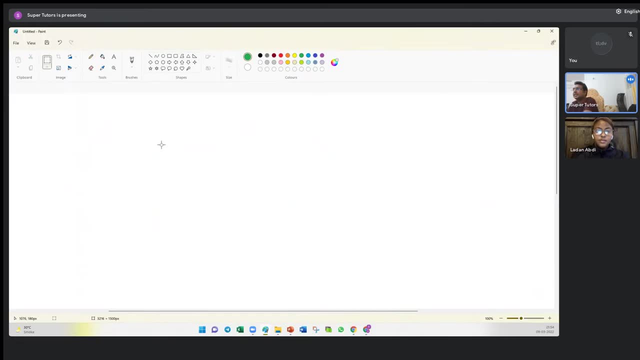 deviation is five, the variance is 25, the square of that right. so standard deviation is normally represented by this symbol, which is called sigma right. so again, since we always uh differentiate between the population and the sample for the population, the standard deviation is referred to as this symbol. it's a little circle with the extended 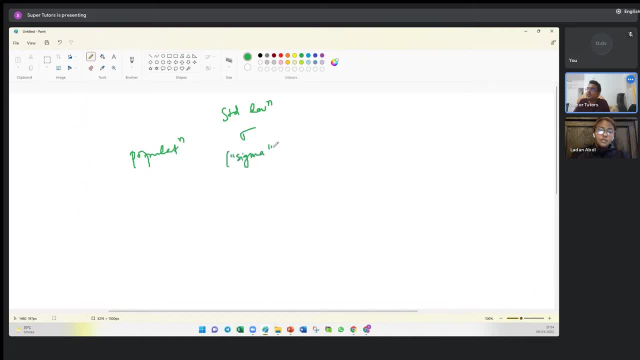 tail on the top and this symbol is read as sigma for the sample. this is given as s just s, a small s right? yes, that's just s. similarly for the mean, just for you to draw a parallel in your head. this is mu for the population. for the sample, it is x bar, if that makes sense. yes, so of course, as i said, 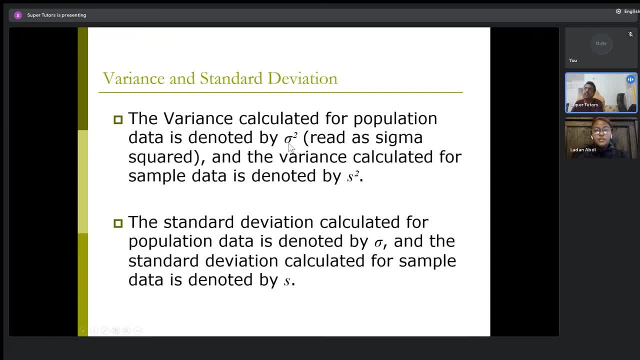 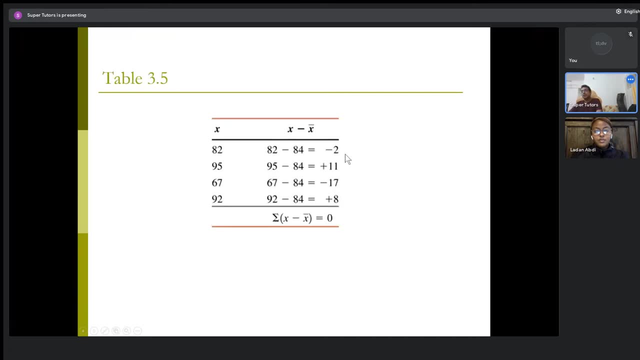 if i square up sigma, i will get the variance. so the symbol is sigma squared, just sigma, with the square symbol on top, and similarly, for the sample variance i will just have s square. does that make sense? yes, yeah. now how do i calculate the variance and standard deviation? 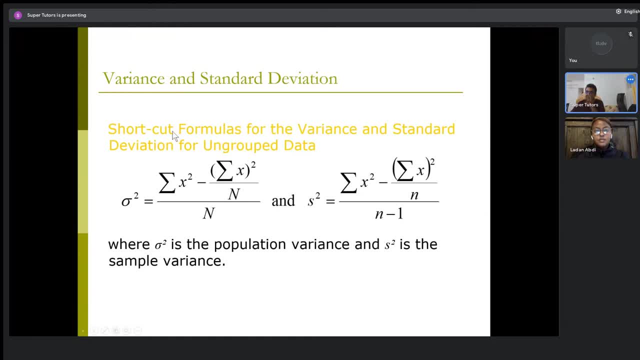 for groups. so in the example we have an x bar for the sample variance and the standard deviation for ungroup data. so we have certain horrible looking formula that you see on my slide which unfortunately we'll have to use in our exam if you have ungrouped data. but the good news is that 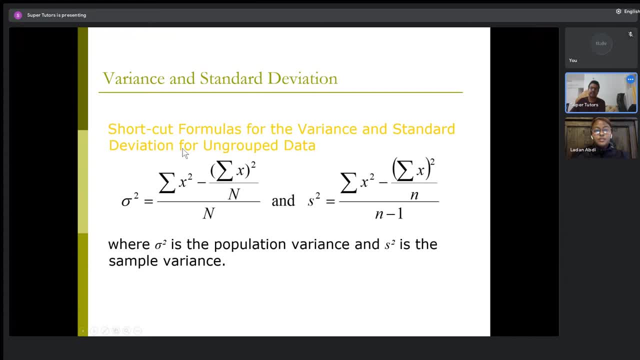 this formula will be a part of your cheat sheet so you need not worry about anything. so sigma square is the population variance and s square is the sample variance. summation of x square minus summation of x whole square divided by capital n: the whole thing divided by capital n and s square is summation of x square minus summation of x whole square. 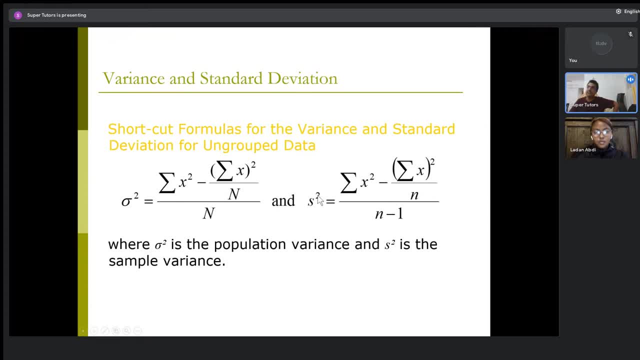 divided by n, the whole thing divided by n minus 1. now this is where we use different formula for the sample and the population variance, and you have to be extremely, extremely careful, okay, right, so for the sample variance, when you're calculating it, the ultimate denominator here is n minus 1. 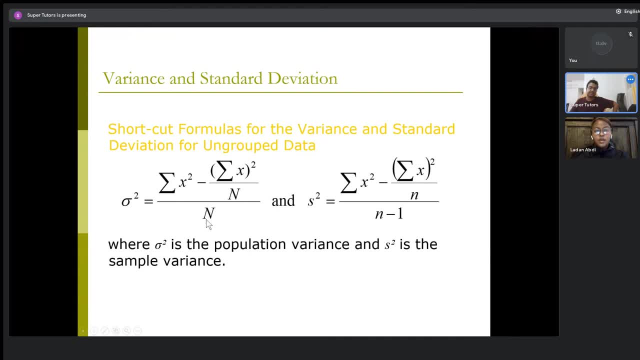 for the population. it's capital n okay, but on the top it's fairly similar. if you've seen this whole thing, and this whole thing is fairly similar, right? yes, is it all sinking in? yeah, yeah, this is good. so far questions anywhere till now? no, perfect, perfect. 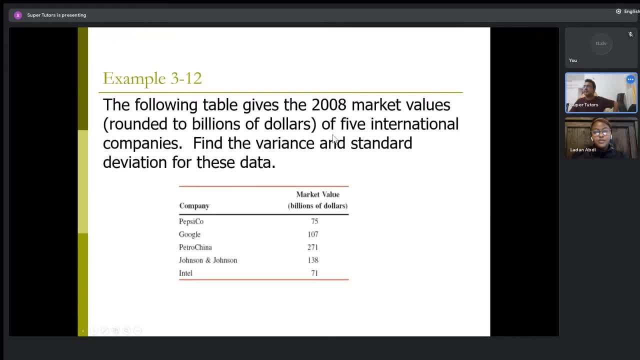 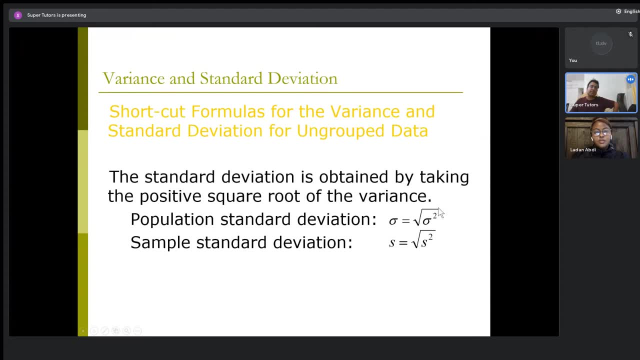 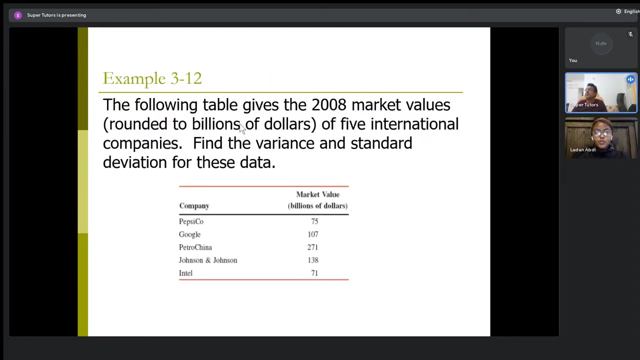 and, of course, if you have to impute or calculate the standard deviation from the variance, you simply take a square root of that. so population standard deviation is nothing but square root of sigma square, and sample standard deviation is square root of s square. that's it, okay. so the following table gives the 2008 market values of: 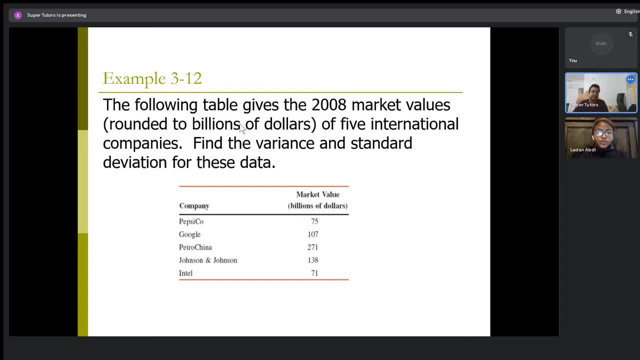 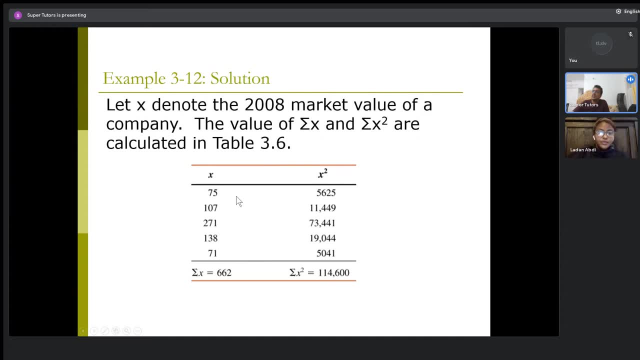 five international companies find the variance and standard deviation for this data. so how will we approach this? the same kind of approach. we will have our x's as these market values. this is my variable and since i need x square and the summation of x square for the formula, i will add a separate column for x square and calculate all the squares of these. 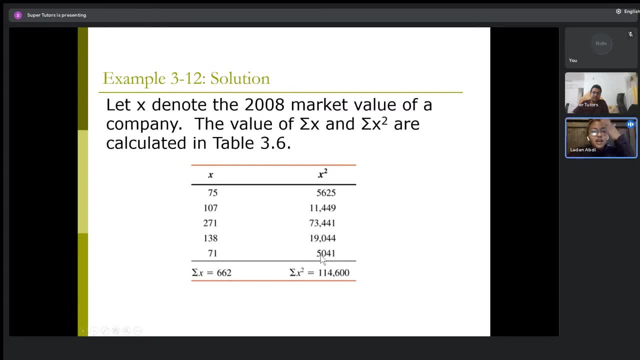 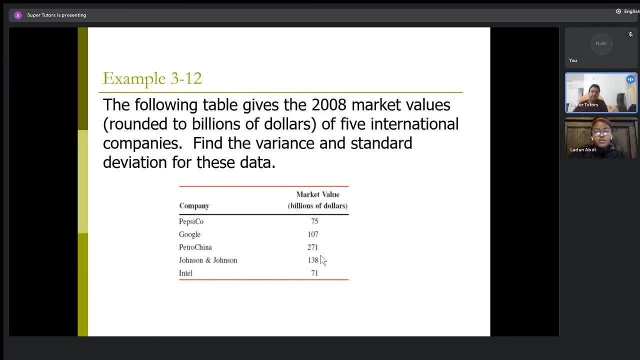 numbers fairly straightforward. yeah, is this group data or ungrouped data? you tell me group data. right, it's ungrouped data. if you've brushed up your chapter two, you would know that group data basically means where you have ranges for the class. so upper limit, lower limit, upper boundary, lower boundary, groupings- this is ungrouped data. 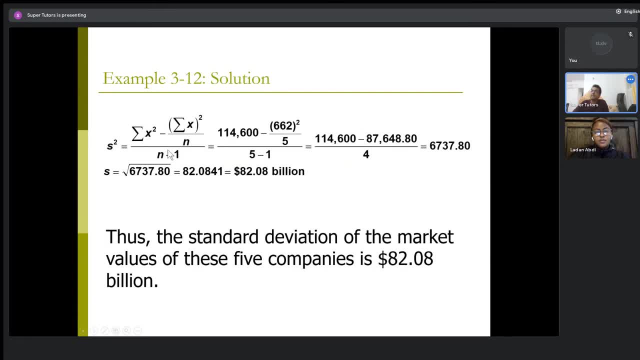 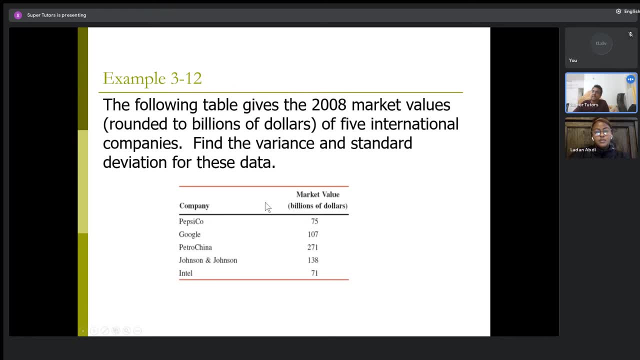 yeah. so how do we calculate it? the final answer very simple. now, this says: 2008 market values of five international companies. is it a sample or is it a population as a sample? and how do you know that? because it says, uh, five international companies, yeah. so there can be like five million international companies, we don't care. 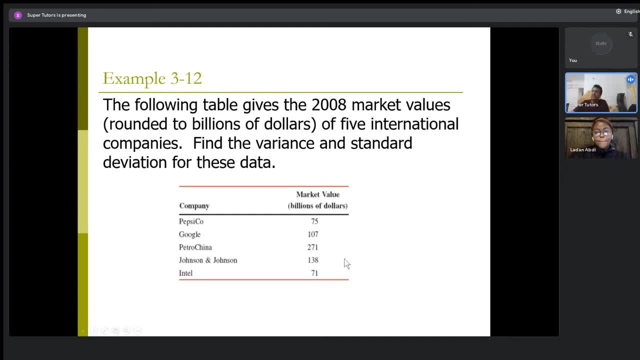 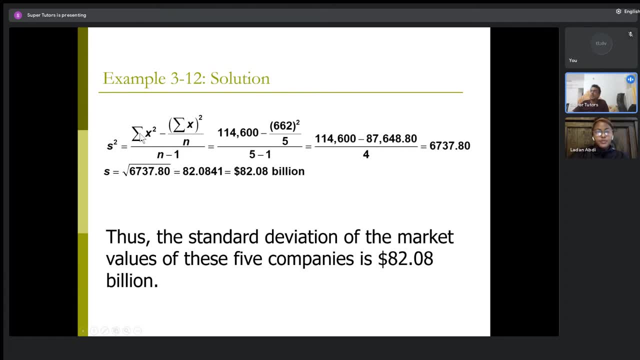 but definitely more than five right common sense. so it's a sample for a sample. you have n minus one as the final denominator, the summation of x square minus summation of x whole square divided by small n, and then you go on doing some calculations and you get this number as your. 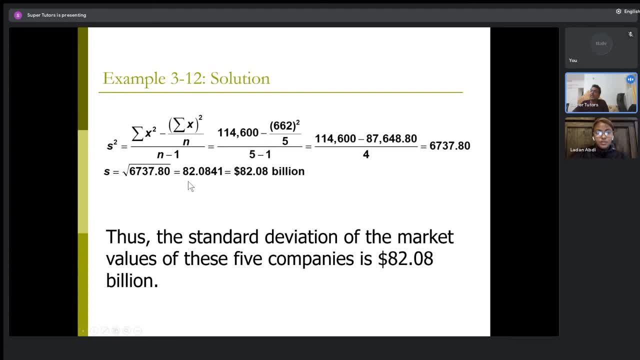 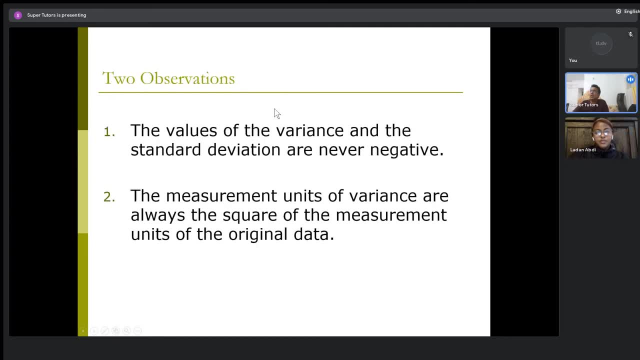 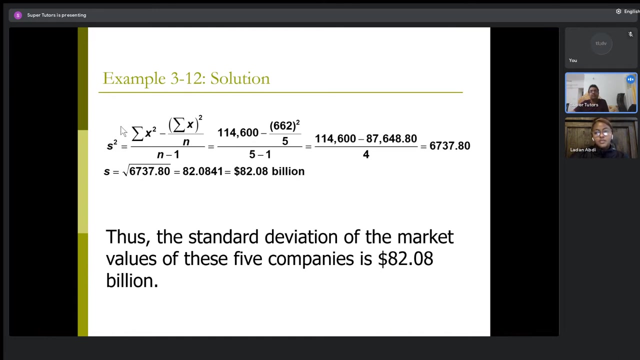 variance s square, then simply take the square root of that. you find your standard deviation. now, one thing to note here is these: both of these, like variance and standard deviation, can never be negative. and why is that? because you are squaring up something. when you square up something, it will always be b positive. 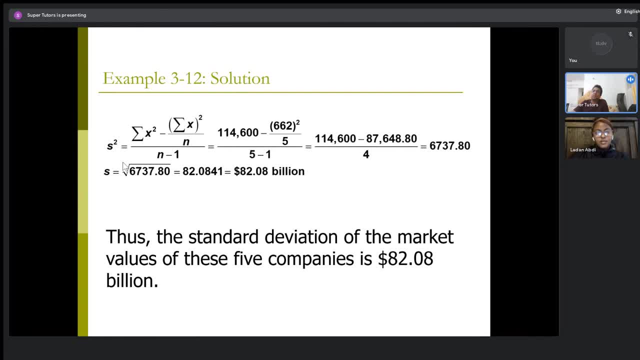 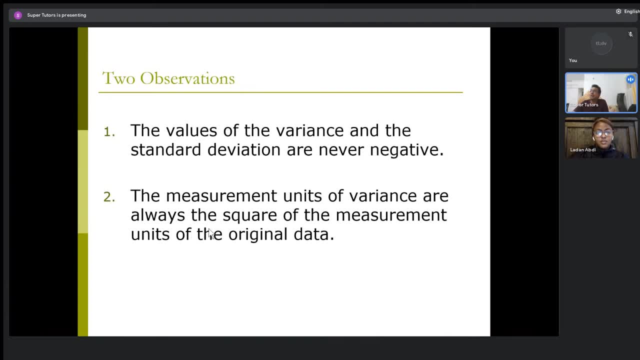 okay, and when you take the positive square root of that, that number will obviously be positive because there are two octaves in it, so that if it's a positive square root of one and you go to the other, Sal detail be positive. second thing is measurement. units of variance are always the square. 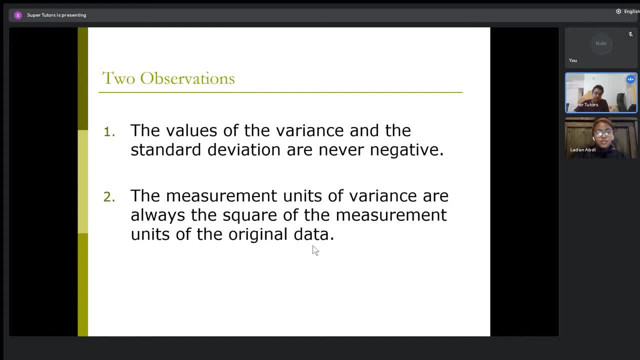 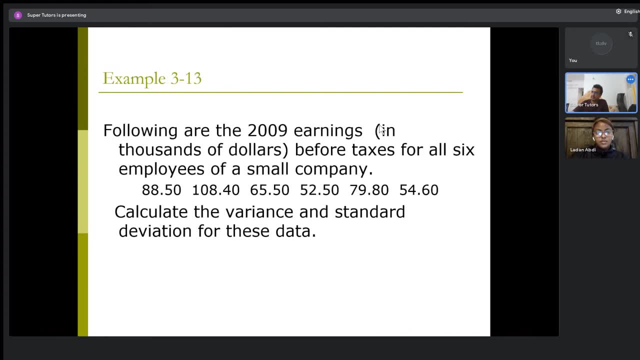 of the measurement units of the original data. so, like when we calculate area, its centimeter square, not centimeter right, the similar concept. okay, can you try this one end-to-end? give me the final answer, okay, mm-hmm. so jot down the data and then I'll bring up both the formula for you and you will tell me which one. 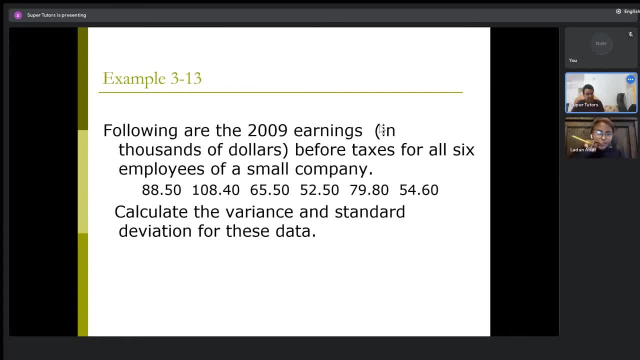 to use. once we agree on that, then you can just go ahead and do your calculations. yeah, okay, you, so this one is sample. it's a sample. yeah, what does it say? oh, okay, oh I, I, I missed the all, I just I just read the six. yeah, yeah, so all six means population. 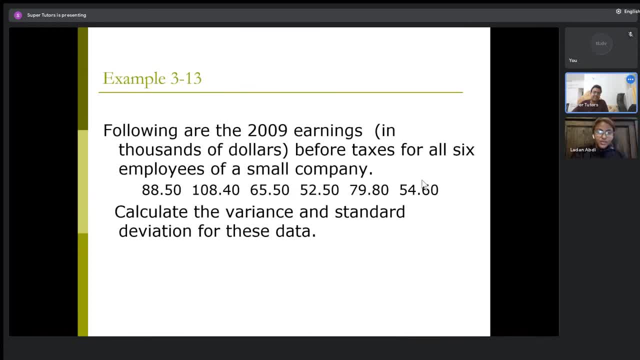 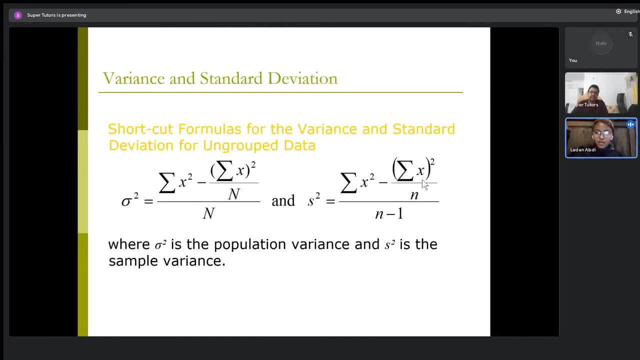 population? yeah right, so you will. you've jotted down these numbers. yeah, perfect. so which formula are we going to use from here? the, the little thing with the square. no, the first formula of the second formula. first one, first one. so let's try to use this and find the variance, and then we'll calculate the. 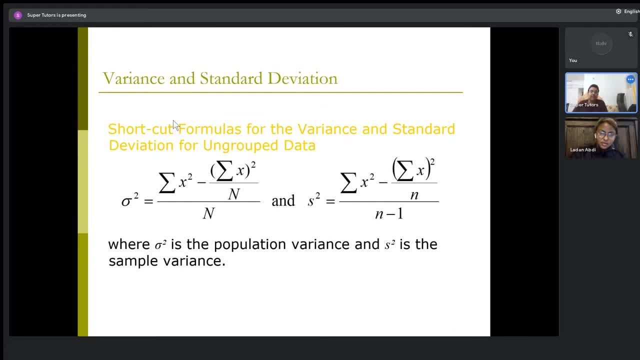 square root. so add one column for your x squares. be very, very careful with your calculations. do not commit silly mistakes. right, and then let's find the standard deviation. now i have to find all the x squares for this. yeah, absolutely. well, it's going to be longer, yeah, so i just want to. 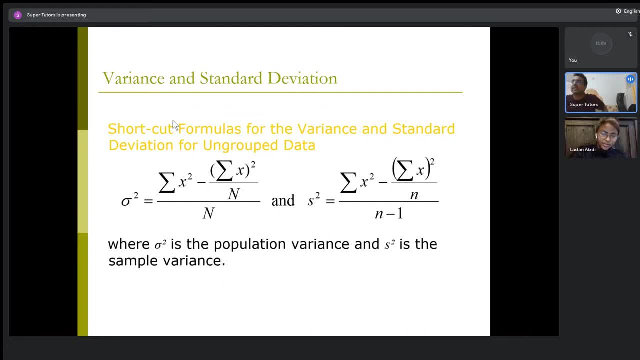 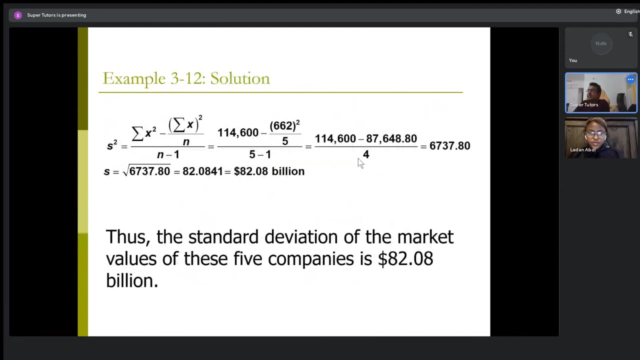 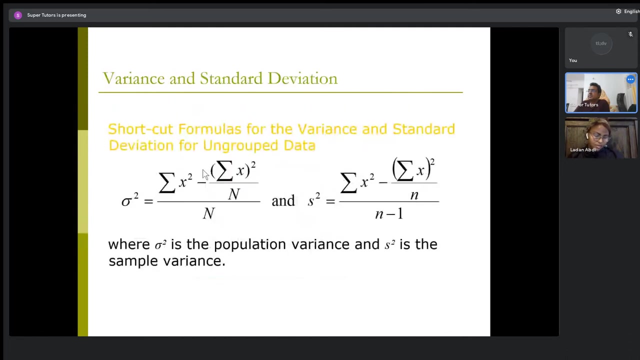 want you to do this problem end to end, so that you are comfortable with the calculations and you don't commit silly mistakes. right, yeah, so, Yeah, So where are we at? I just did the square. Now I have to add them all up. Okay, go on. 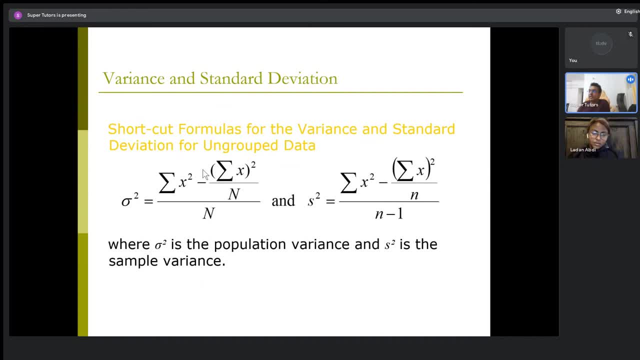 When you have the sum, just give me the sum before applying the full formula, so that I can just compare it to what I have on the slide Before squaring it or after squaring it, After adding the squares. Oh, okay, Yeah. 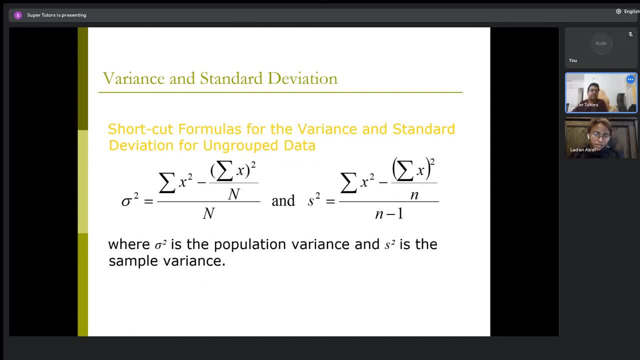 Okay, Just that simple. Yeah, it's not a big deal. Yeah, So I'll just go ahead and add the squares here. Okay, So I'm going to add the squares. Okay, Okay, Okay, Okay. Okay, That's a great idea. 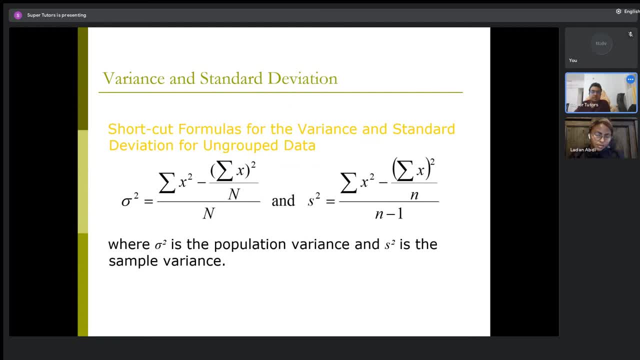 Okay, Thanks, Thanks, Thanks, Thanks. What else do we need? We can add, I don't know, whatever that we think we need. Yeah, Like it's a real piece of cake, I can't wait to add them. 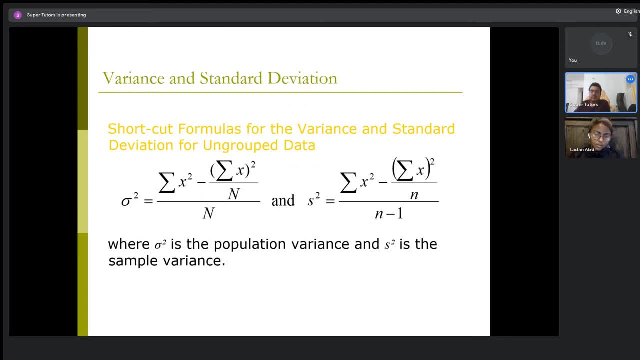 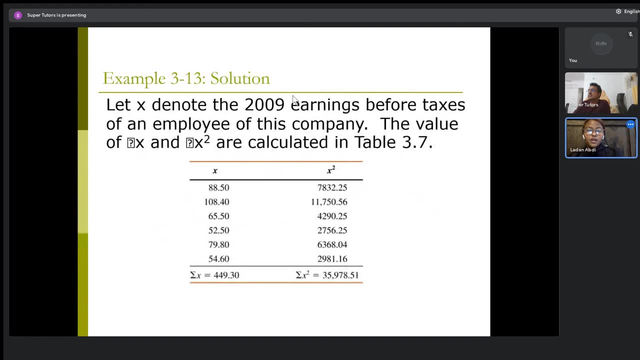 Okay, All right, We just going to pass it on to the next slide. Thank you, It's a good idea. oh, i have uh, 35, 978.46. yeah, that's fine, it's 0.51, but does not make a difference. 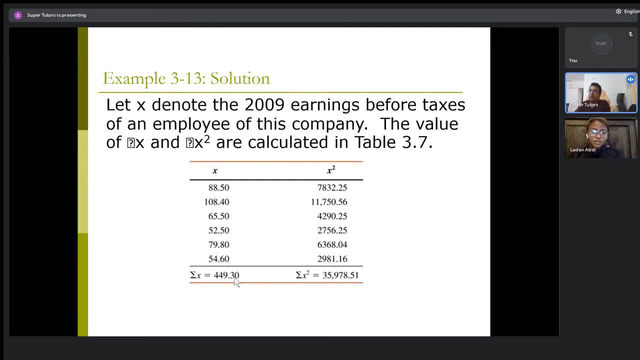 and uh. similarly, summation of x will come to 449.3. just jot down this value. you don't need to add up x- 449.3. you have the two numbers jotted down. yes, now just try to apply this formula, please. the first one. 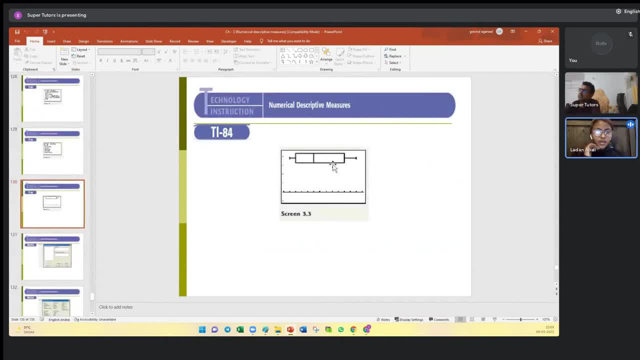 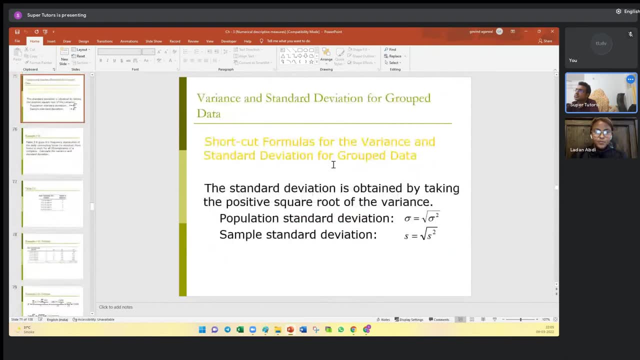 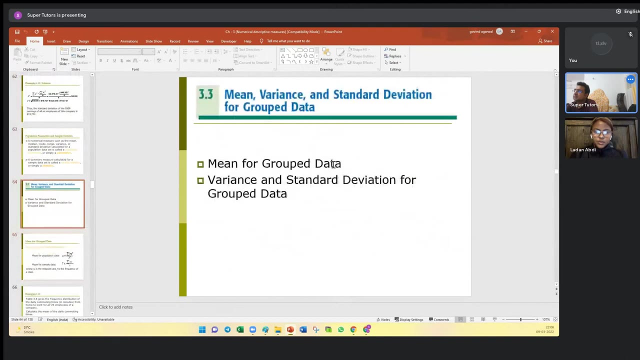 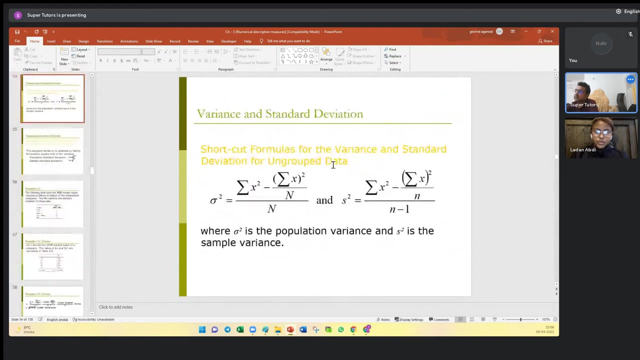 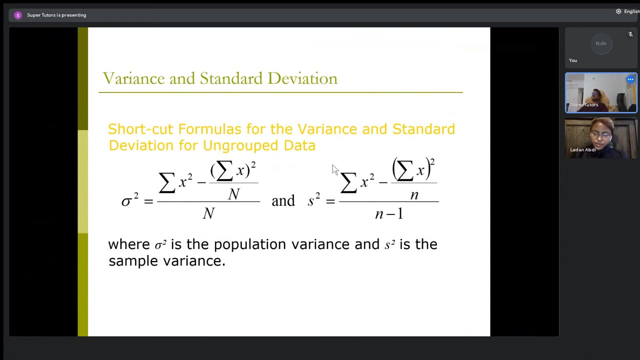 can i see the formula again? yeah, i'll just go back to it. give me one sec, okay. yeah, okay, got it. okay. what's the final answer? you have it. no, i didn't do it yet. yeah, go on, take your time. uh, um now, uh, uh, uh. 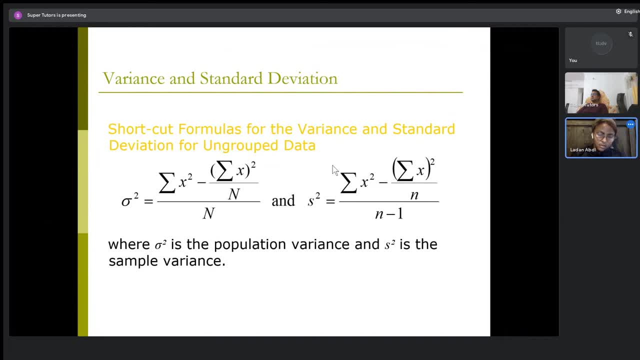 uh, uh, uh, uh, Thank you, Thank you. I'm subtracting and I'm going to divide. Okay, okay, Okay, I got 388.. 388.89.. Okay, let's take a look. Yeah, 388.90.. 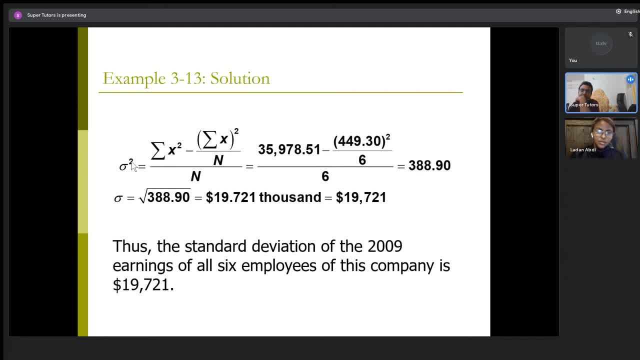 So that's the same thing for the variance sigma square right. I'm glad that you did not commit any silly mistakes here, which many students do So definitely you are among the better lot. That's a good thing, And sigma is square root of that number, of course. 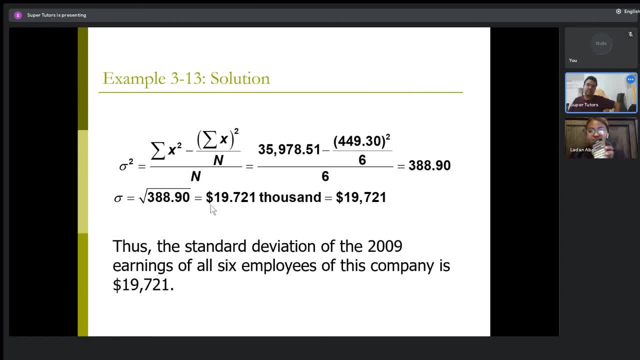 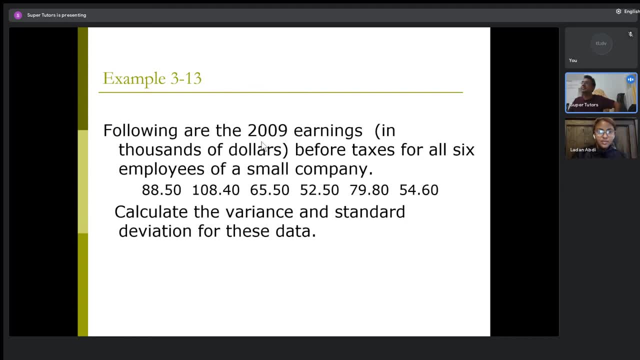 So it would come to 19.721.. Yeah, I got it. Perfect, perfect. Yeah, So that's the standard deviation And the data was in thousands. If you recall, we started and said that these are the 2019 earnings in thousands of dollars. 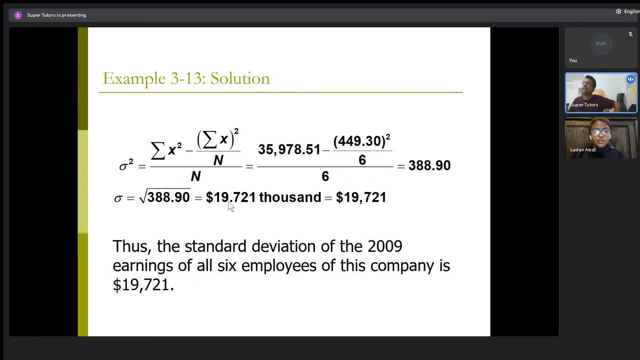 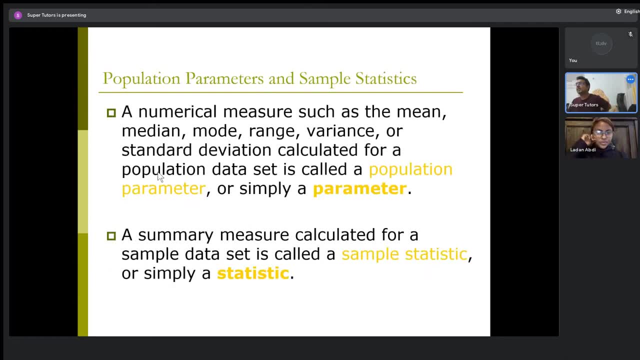 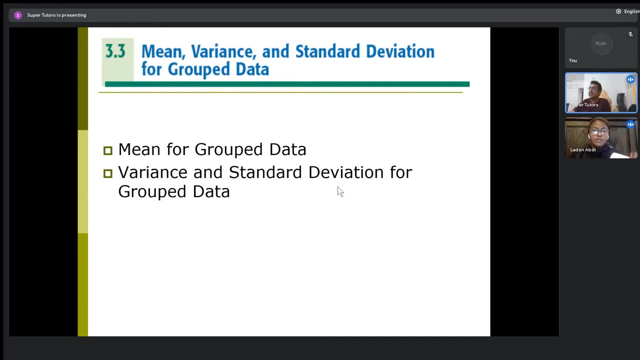 Yeah, okay. So 19.721 basically means 19.721,000.. So basically 19721, right, Yeah, Perfect. So we come to something called mean for group data now and the variance and standard deviation for that. Okay. 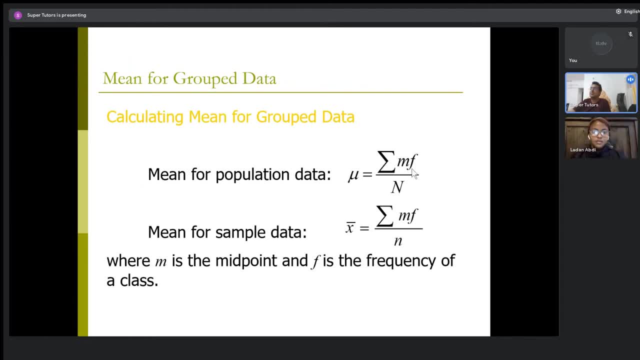 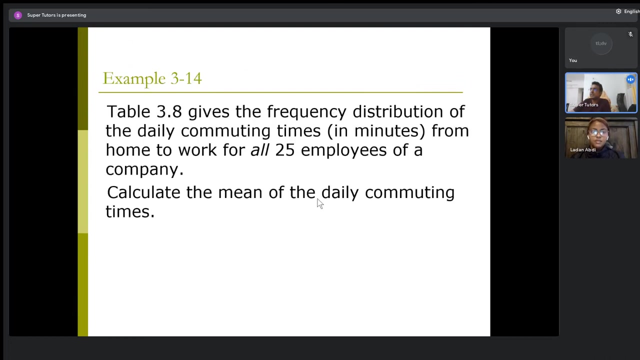 So mean for population data. So mean for population data is given by summation of MF over capital N. and of course, mean is a very simple guy. mean is a very simple formula. for the sample also, the formula is the same. X bar is summation of MF over small n. so M is the new thing that we're introducing here, that's the midpoint of every class and F is the frequency. so I have some data about the daily commute times for 25 employees. this is group data. now you recall it. 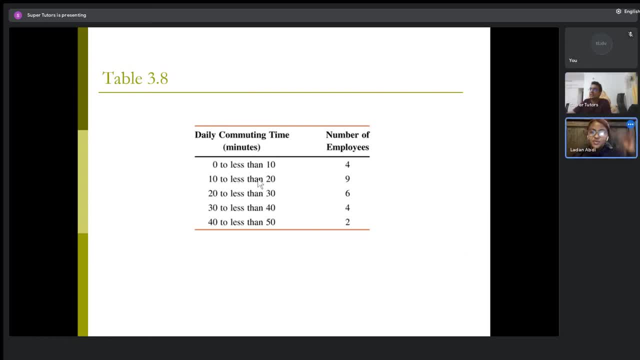 Okay, Now you recall from chapter two. Oh, yes, yes, yes, When you have classes in terms of ranges like this. Okay, Right, So we have daily commute times of 25 employees. The first set of employees commute between zero to 10 minutes every day. 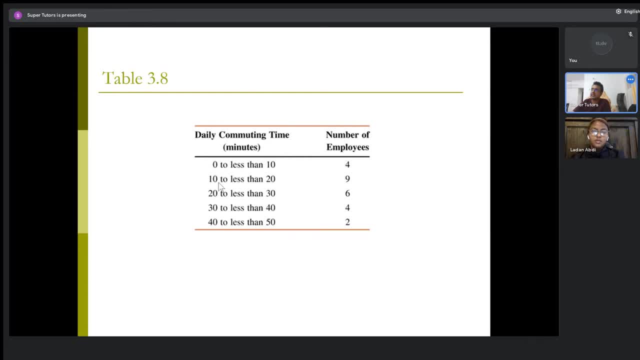 And how many employees do we have in that class? Four, Then nine employees commute, between 10 to 20, and so on, Nine, Okay. So if I have to find The mean of this data, I need the midpoint of every class. 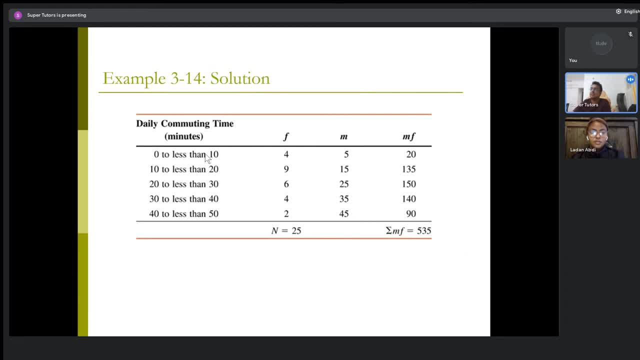 Midpoint is simply upper boundary plus upper boundary plus lower boundary divided by two. So zero to 10 comes to five, and then 10 plus 20 is how much? 15, 10 plus 20, 30 divided by two is 15.. So you get these midpoints, you already have the frequencies, so you have to find the summation of MF. 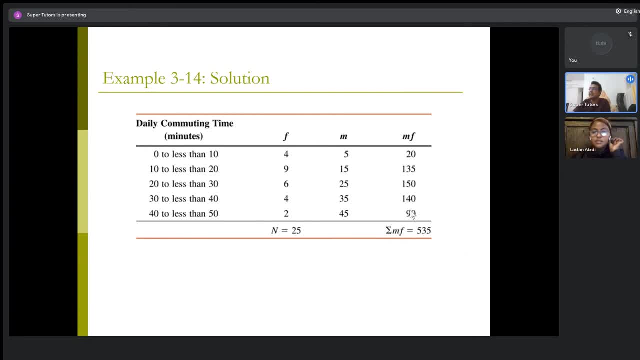 And we said in chapter one that whatever has a summation symbol next to it. you find that as a different column. So you find all the values of MF. Multiply each M with the F, Go on finding the products. Does that make sense? 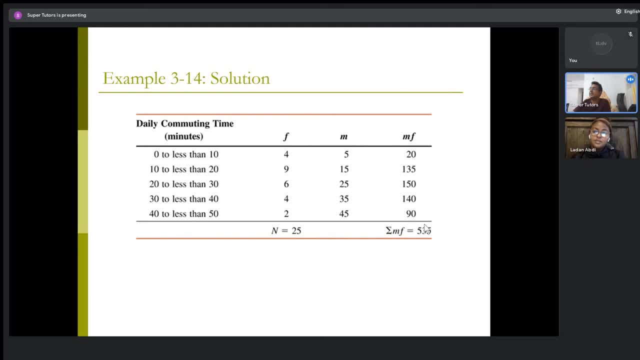 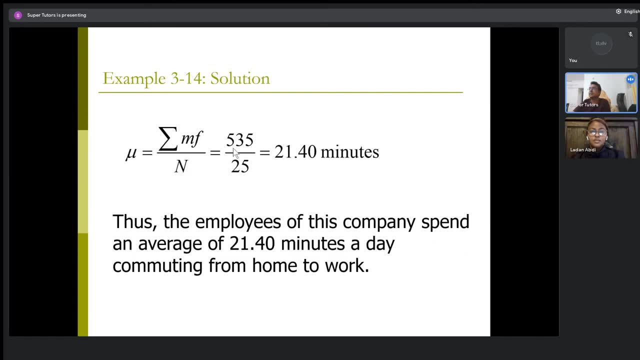 Yeah, Yeah, And then add these up, It gives you how much: 535.. Make sense, Yeah, So summation of MF over capital N is 535 divided by 25, which is 21.4.. 4 minutes. 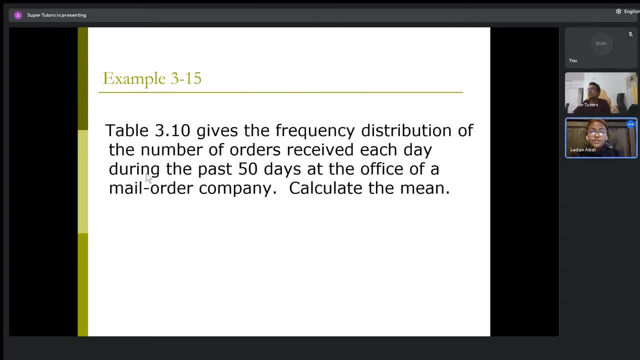 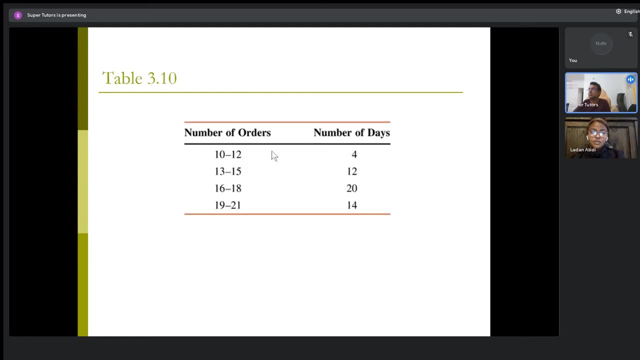 Yeah, Yeah. Table 3.1 gives the frequency distribution of the number of orders received Each day during the past 50 days at the office of a mail order company. calculate the mean. So similar process: we add an M 10 plus 12, 22 divided by two is 11.. 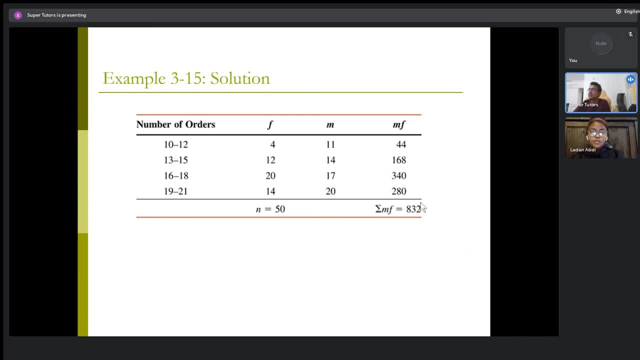 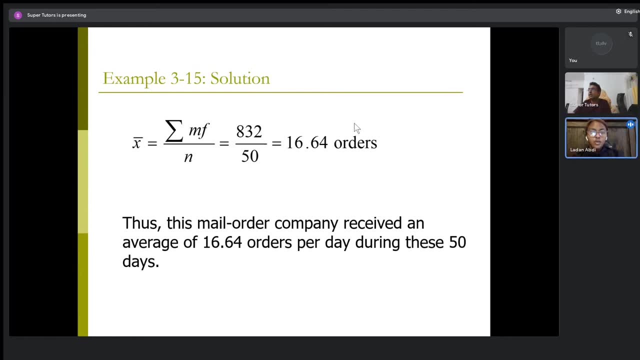 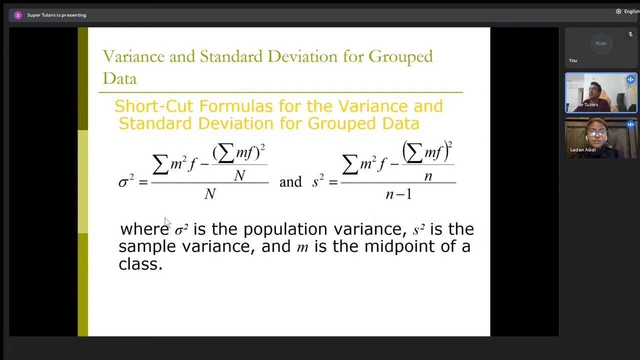 So on. find the midpoints, find the products, Sum them up and divide by 50. Sounds good, Fairly straightforward. Yeah, This is straight forward, Yeah. And if you have to find the variance and standard deviation for group data, the formula is again slightly complicated. 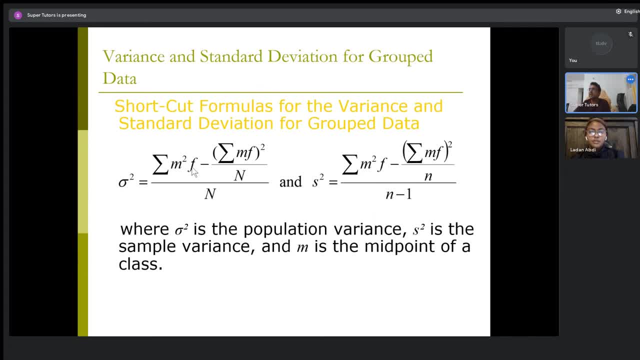 So for population variance, Sigma square, you have summation of M square F minus summation of MF, whole squared divided by N, divided by N. For sample variance, The numerator remains the same and denominator changes to N minus one. So this is the group data. 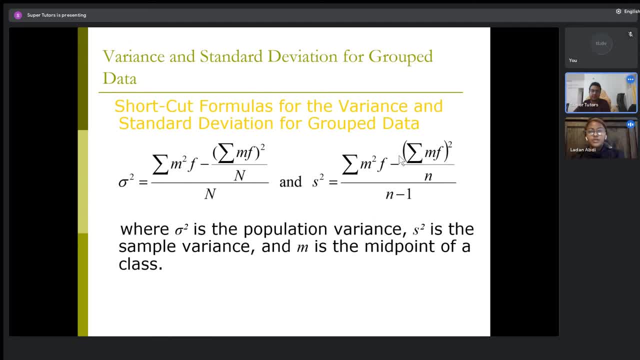 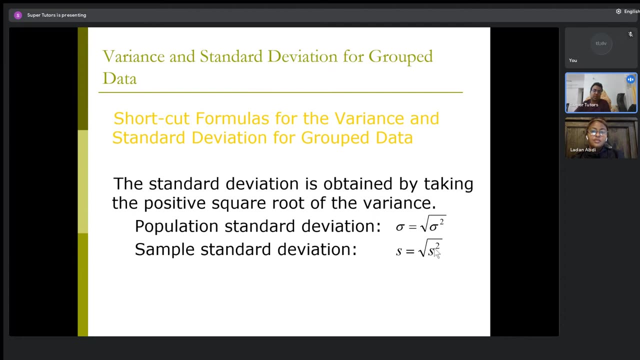 Sorry, This is for the group data. Yeah, absolutely Yeah, Group data similar to the previous set of data that we went to. We will set a formula. It's very similar And, of course, the standard deviation is again. of course, it's just the plane square root of whatever you find as the variance. 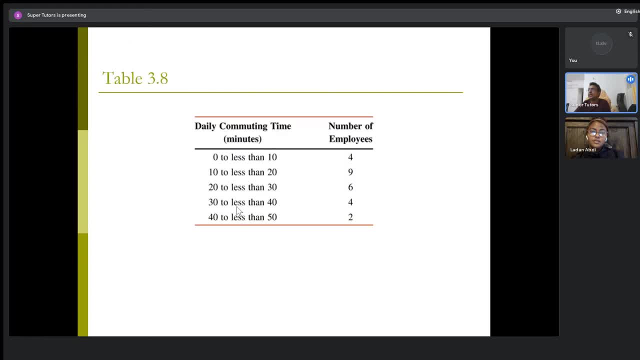 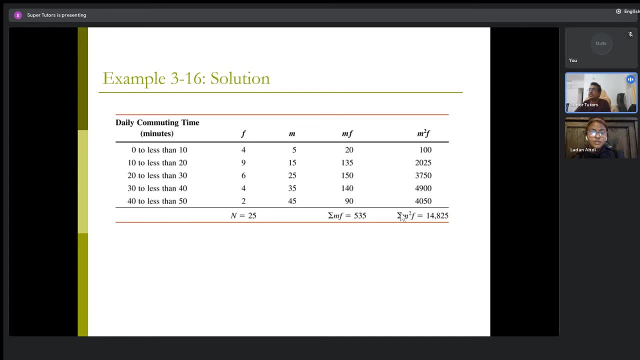 Mm, hmm, So same data. let's try to find the standard deviation now. So for the variance, I need summation of MF and summation of M square F. I will add two new columns, apart from the midpoint, which is another new column. 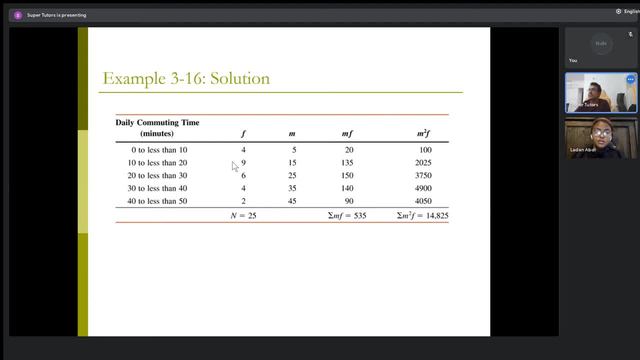 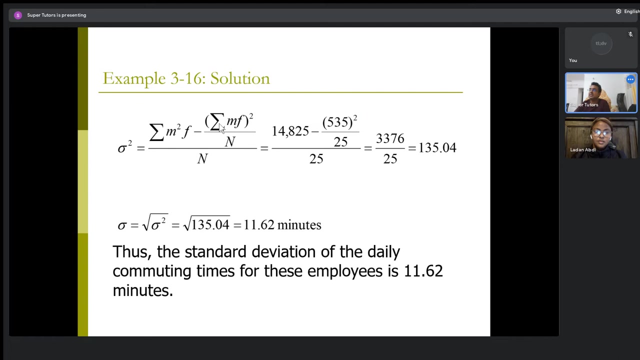 So midpoint, just the midpoints of all of these, MF, which is product of each M and F, M square F, which is the product of M square times F, Summation of M square F is this number. So sigma square is nothing but the summation of M square F minus summation of MF whole. 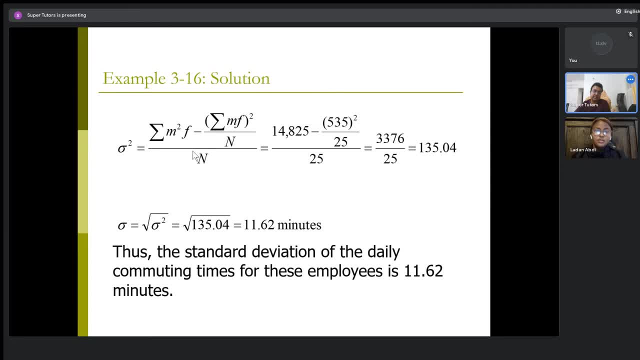 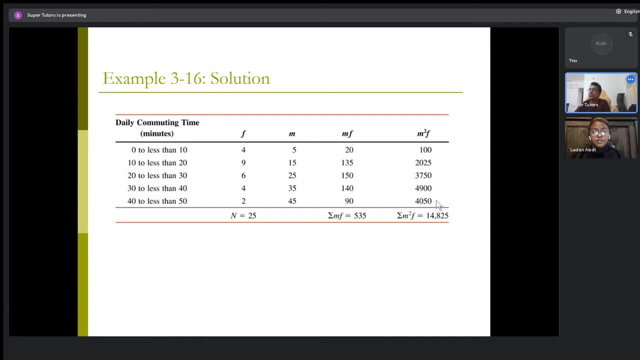 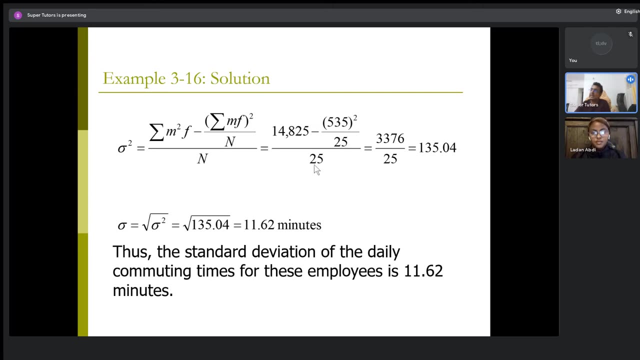 squared divided by N, the whole thing divided by capital N. Right Yeah? Summation of M square F is this number: 14825, minus summation of MF whole squared divided by N. So MF 535 whole squared divided by 25, and the whole thing again divided by 25.. 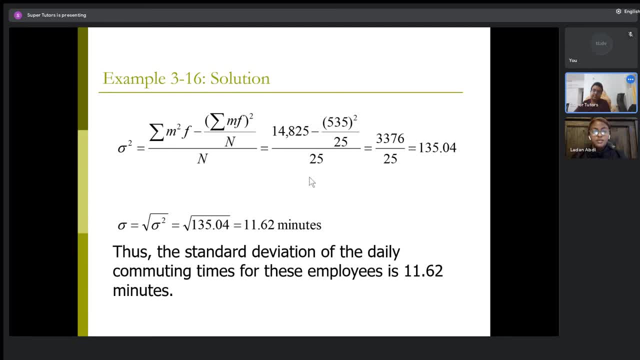 That makes sense. Yeah, Yes, So you will get how much? 135.04,, if that makes sense. Similarly, sigma is nothing but the square root of sigma square, and that comes to 11.62.. Just be very careful with the M square F, because that's where students make the most mistakes. 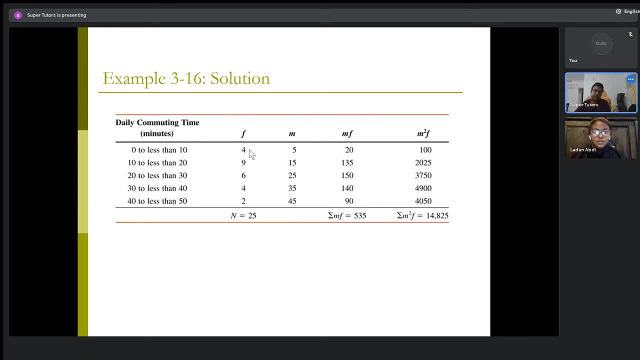 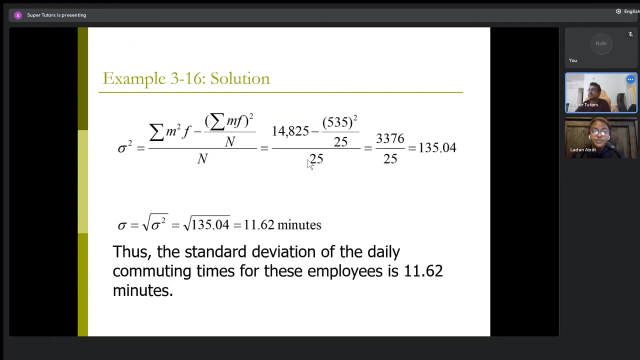 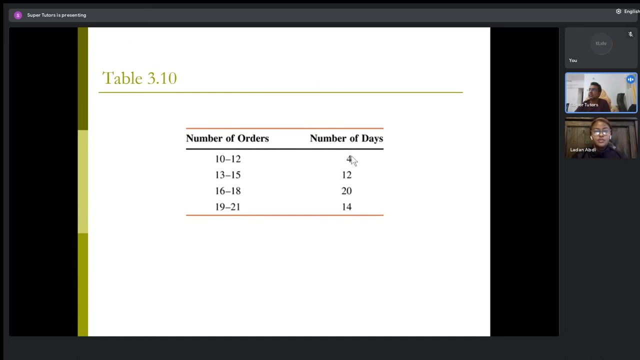 Yeah, So you have to multiply the square of M with F. Yeah, So 5 squared is 25, and that gets multiplied to 4, giving us 100.. Okay, Yeah, And so on, Right. So this example is again the same example for the standard deviation that we did for. 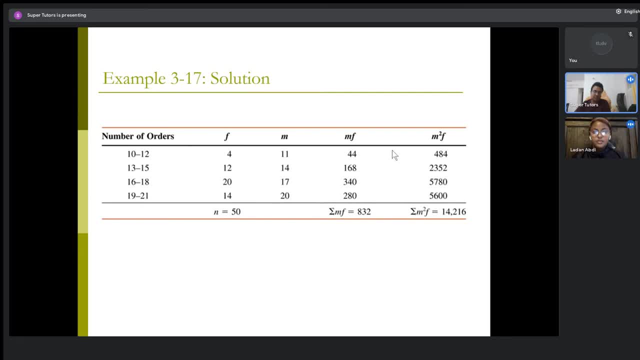 the mean Just skipping this in the interest of time. not like very different, It's the same thing. We come to a very important concept of Chebyshev's theorem. Chebyshev is the one I had issue with, Yeah. 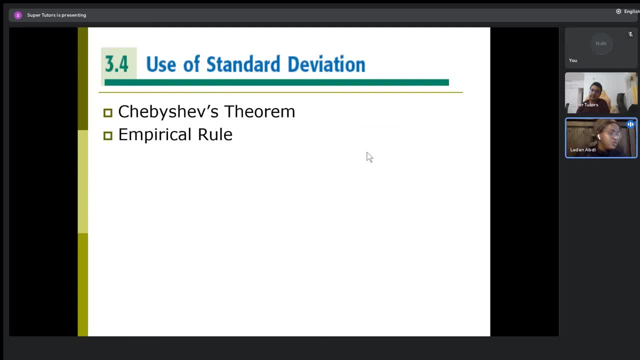 So Chebyshev's theorem, if you read the definition it will never make sense. Right, For any number greater than k, greater than 1, at least 1 minus 1 by k square of the data value lie within k standard deviation of the mean. blah, blah, blah. 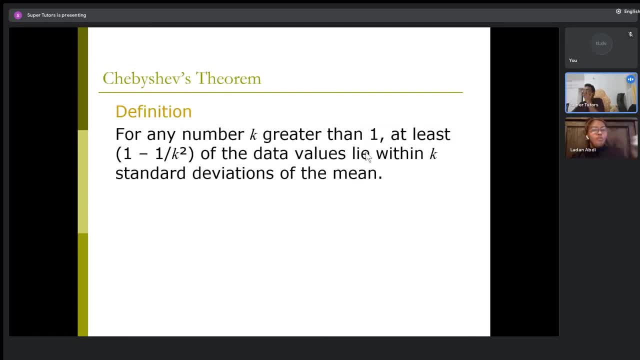 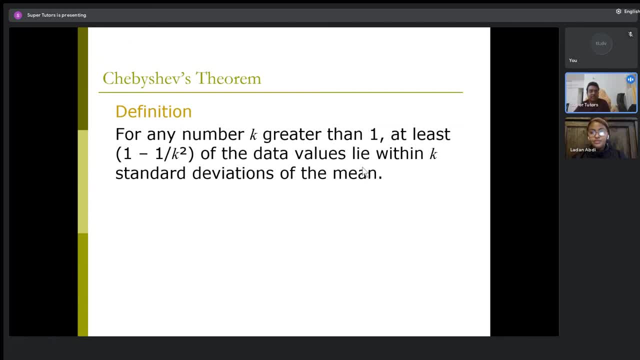 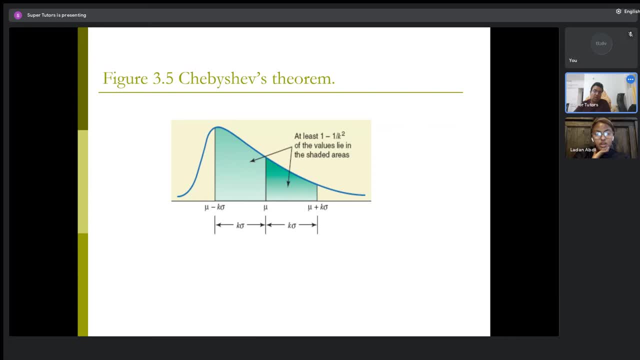 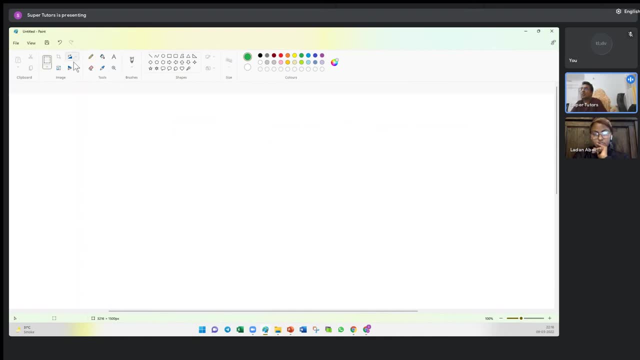 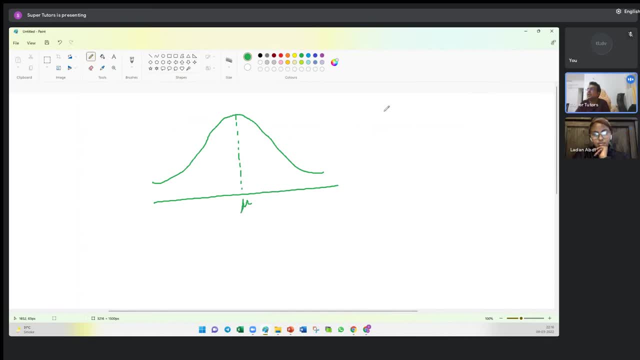 Yes, So I have something called standard deviation, which we know now sigma, And this is always a positive number. This is always positive. So if I add a multiple of this to mu, I would land here. I am adding something positive to mu. 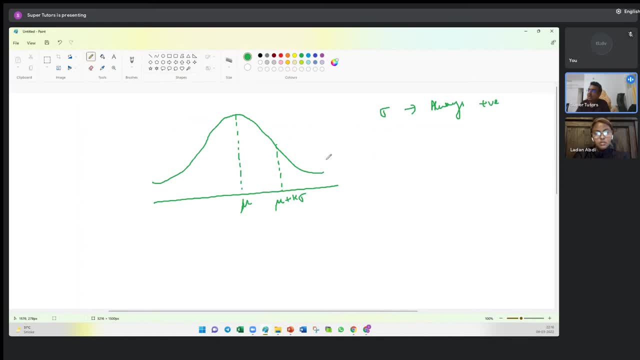 So I will land ahead of mu, if that makes sense. I am adding a kth multiple of standard deviation. k is just an integer. Okay, It is just a number. Right, You can say a positive integer. So mu plus k sigma will be somewhere here, if that makes sense. 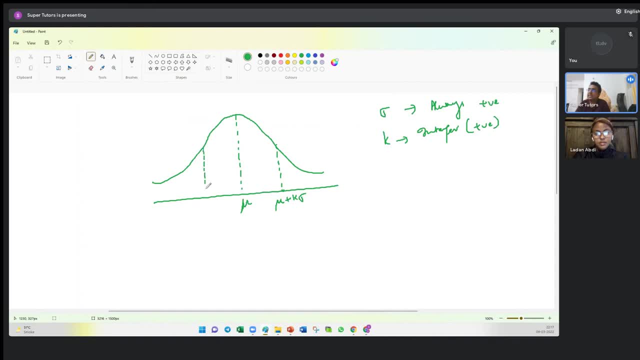 This point. Similarly, if I subtract the same thing from mu, I will go an equal distance back Mu minus k times. sigma Right, Yes, So all Chebyshev did in his entire life was to find what percentage is this? 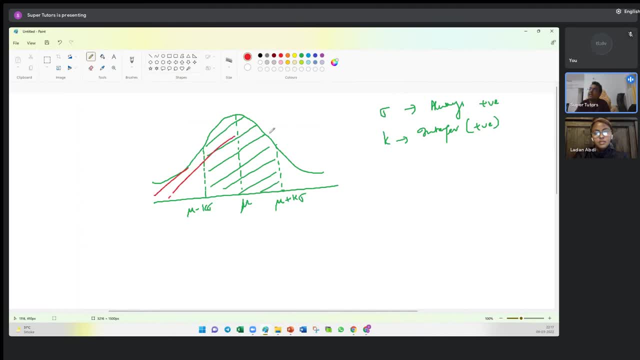 Green area of the total red area, the total area under the curve. what is the percentage of that green in the total red? Does that make sense? Mm-hmm. And he concluded that the green divided by the red is greater than or equal to 1 minus. 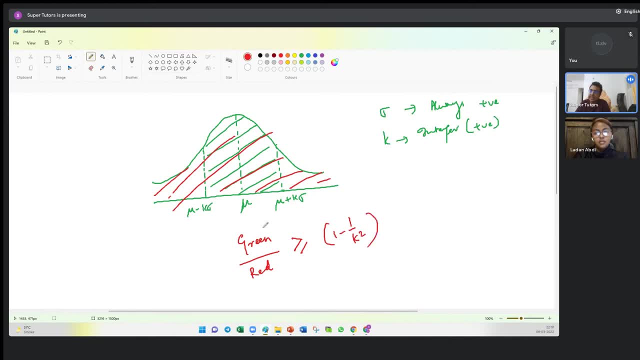 1 upon k square. That's the formula, So this ratio. he did not find an exact answer, Leydon Mm-hmm. He found that it is greater than or equal to this ratio, Mm-hmm Right. 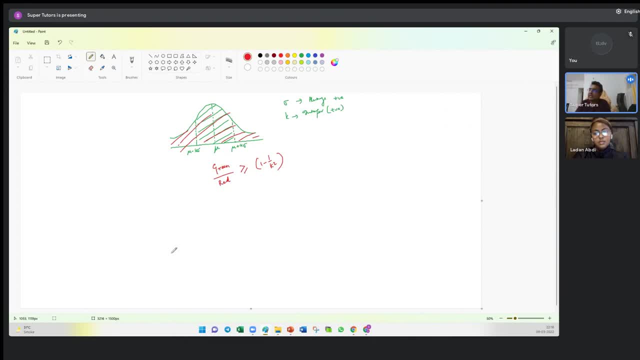 So let's take a quick example and it will become absolutely crystal clear to you: Mu let k equal to 2.. So mu plus 2 times sigma, Right, Mm-hmm? And mu minus 2 times. So mu plus 2 times sigma. 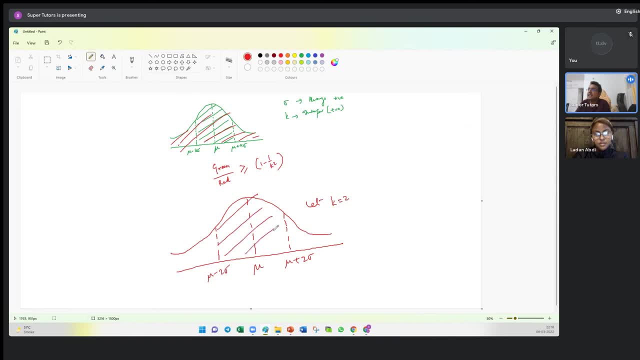 Yes, So then this area, red area upon total area, which is the total area under this curve, Mm-hmm, Right, Mm-hmm, Is greater than equal to 1 minus 1 upon 2 square. 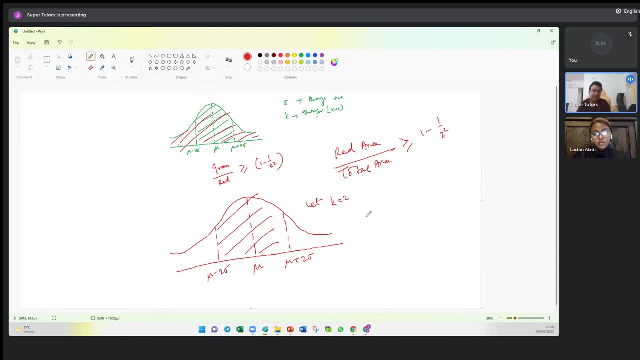 Does that make sense? Is it straightforward? And you got the 2.. Oh, because k Oh, yeah, Yeah, yeah, k is 2.. Yeah, Okay, So I'm simply just putting k as 2.. Mm-hmm. 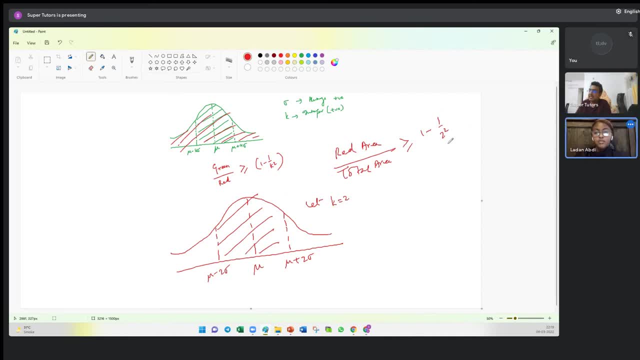 Yeah, Okay, I'm putting k as 2.. As simple as that. Oh, okay, Right. So in other words, can I write: this whole thing is greater than equal to 3 upon 4?. This is what you will get when you like finally solve this out. 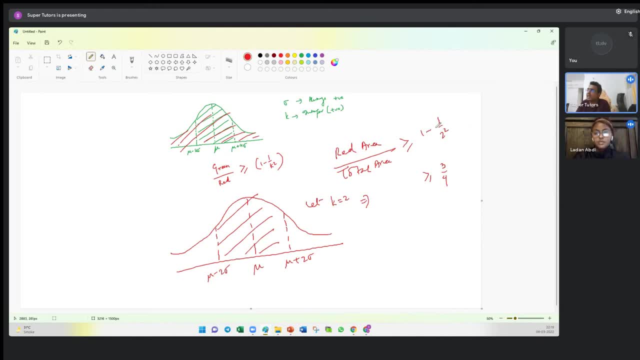 Yeah, So 1 upon 2 square is nothing but 1 upon 4.. And 1 minus 1 upon 4 is 3 upon 4.. Simple, Yeah, So that again is nothing but greater than 0.75, if you do the math here. 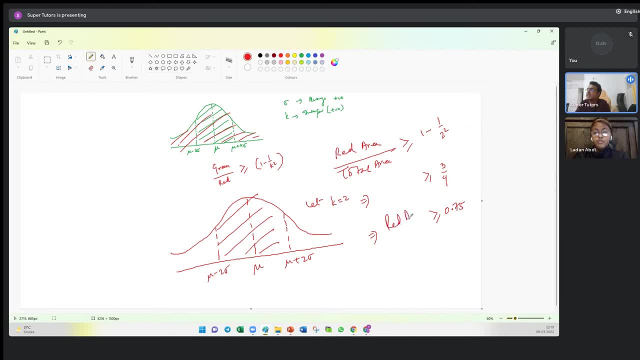 Yeah, So basically just saying that for a value of 2, this red area upon total area is greater than equal to 0.75, or 75%, right? So this is minimum 75% of the total area under the curve. 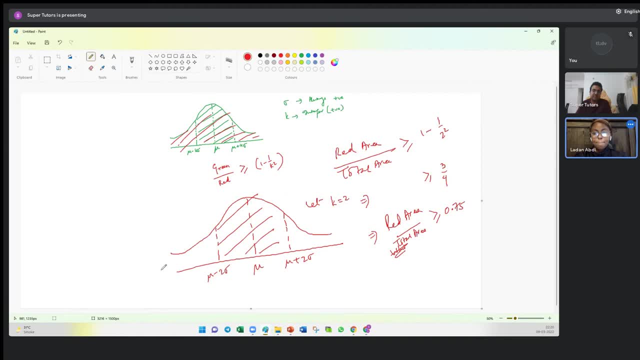 That's all Chabishev said. Okay, Does it clarify for you? Yeah, Yeah, Big time, Yeah, Perfect, So same thing. if I go on and, you know, put another value of k, it will be the same. 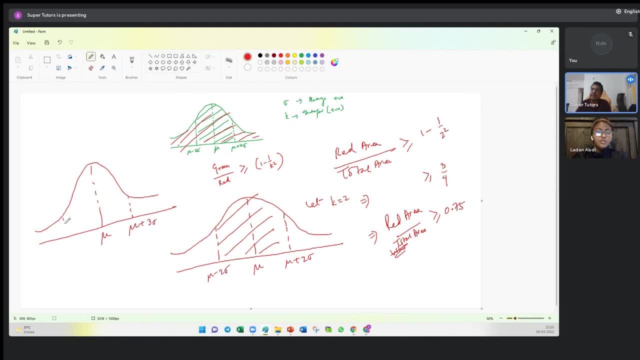 thing: If I say 3 sigma now, so k is 3 now right, And I ask you, what is the green area as a percentage of the total area, Then you will simply say, in this example, green area upon total area. 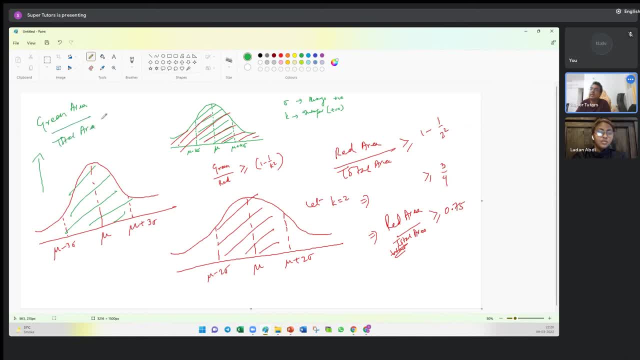 Green area upon total area is minimum or greater than equal to 1 minus 1 upon 3 square. Simple. So 1 minus 1 upon 9.. 8 upon 9.. And just do the math and tell me what this comes to. 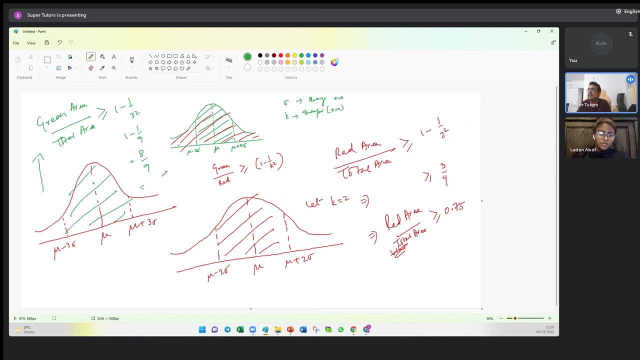 I think it's somewhere around 88.8.. 88.8.. Yeah, Yeah, 88.89.. Yeah, Or actually 0.88 or 88.88. Yeah, Yeah, Yeah, Yeah, Yeah Yeah. 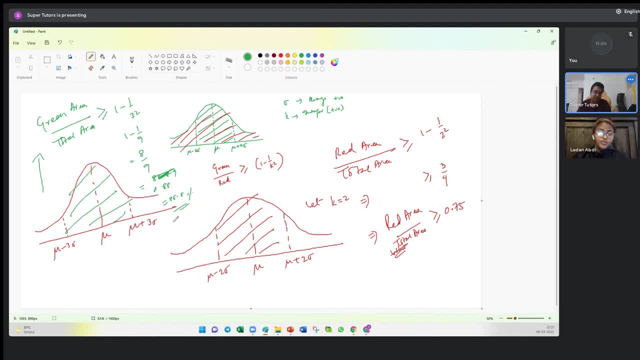 So this green area as a percentage of total area under the curve is around minimum 88.88%. It's actually greater than equal to 88.88%, Makes sense? Yeah, Very clear now, My goodness, That's what I like to hear. 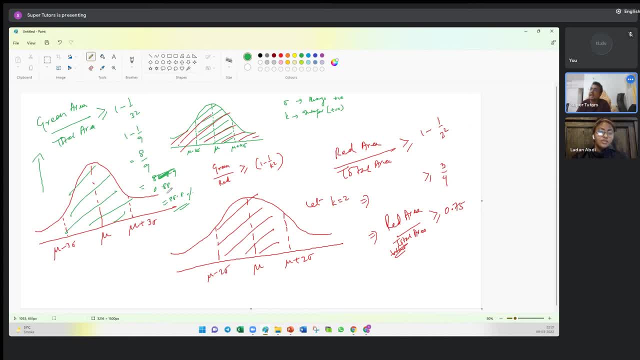 I can't believe I was having an issue. You made it look so easy. Yeah, Yeah, I'm happy to. I'm always happy to hear that. So thank you so much for listening. Thank you, Bye, Bye, Bye. 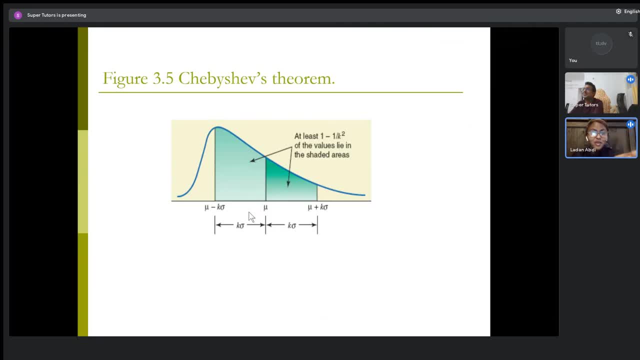 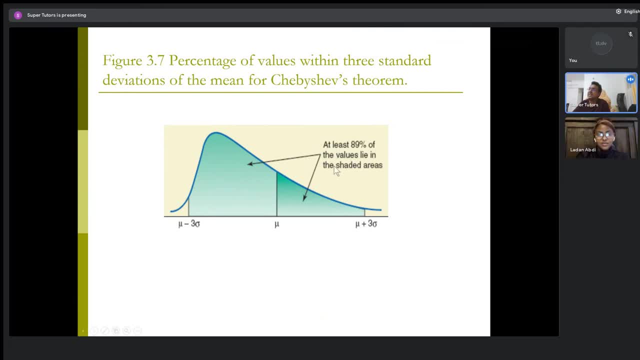 Is it fully clear now? Yeah, this one, yeah, it is Yeah. So if you look at this slide, we have said the same thing. At least 89% of the values lie in the shaded areas, So 89% of the total value under the curve is the shaded area. 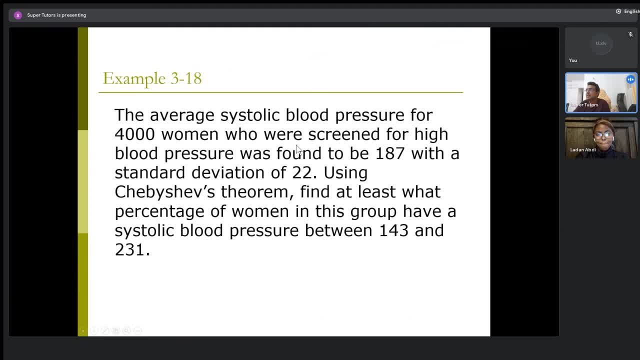 That's it, Right? Yes, So let's see another variation of a problem. using Chebyshev's theorem, The average systolic blood pressure for 4000 women who were screened for high blood pressure was found to be 187, with a standard deviation of 22.. 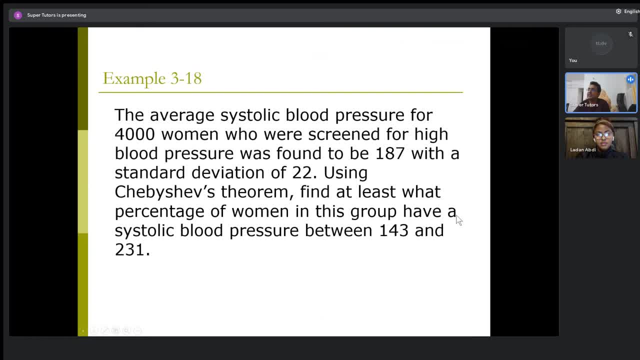 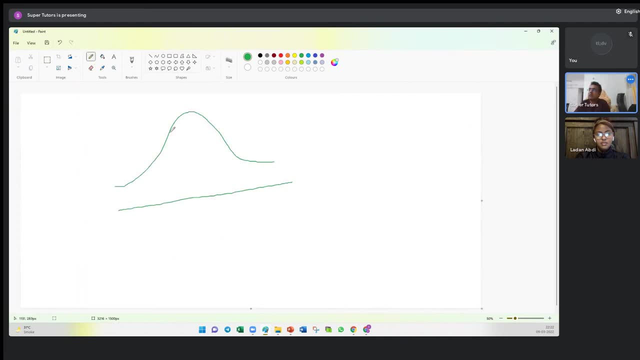 Using Chebyshev's theorem, find at least what percentage of women in this group have a systolic blood pressure between 143 and 231.. So let's see how we do it. What's the mean? This is always the mean. 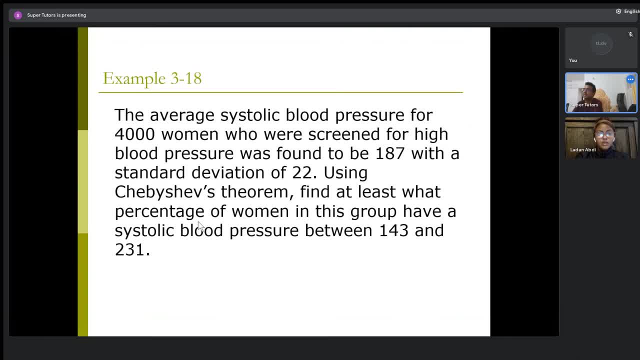 If you look at the problem, can you tell me what's the mean Average? so would it be 4000?? That's the number of women surveyed. The average was 187.. Oh, okay, The average blood pressure for 4000 women. 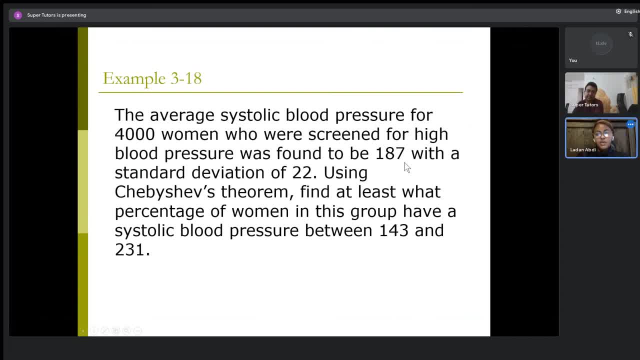 The average blood pressure for 4000 women who were screened was found to be 187.. Okay, 187.. So the mean is: how much 187.. 187.. Right, What's my standard deviation? 22. 22.. 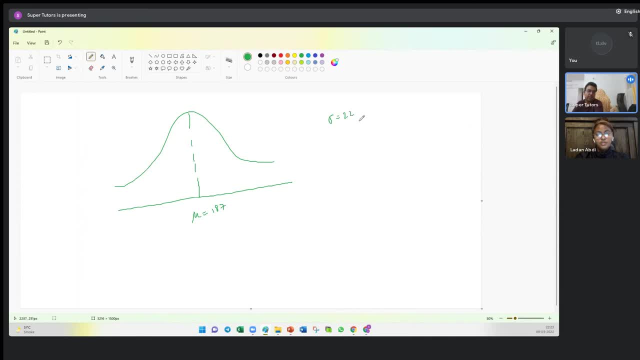 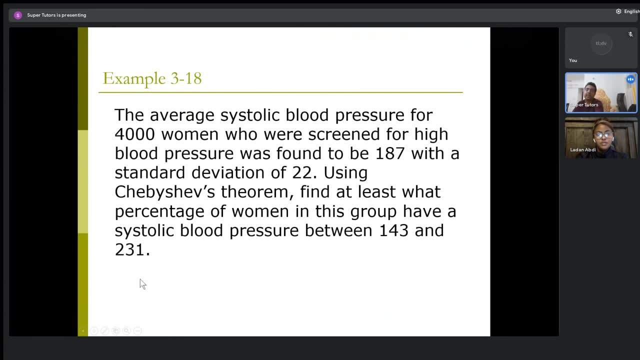 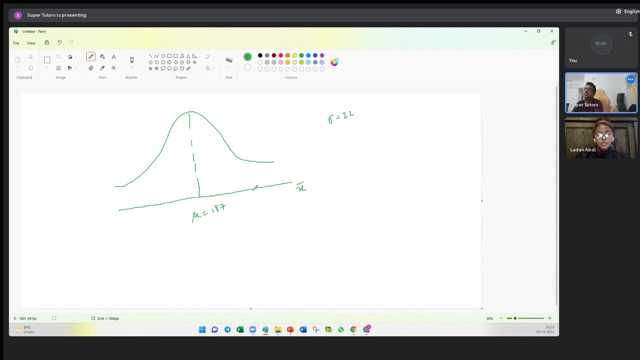 So I will just let it hanging in the air somewhere 22.. That's how we always treat standard deviation. initially. Now read the question: Find what percentage of women have blood pressure between 143 and 231.. So this horizontal line is of course my X, which is the. 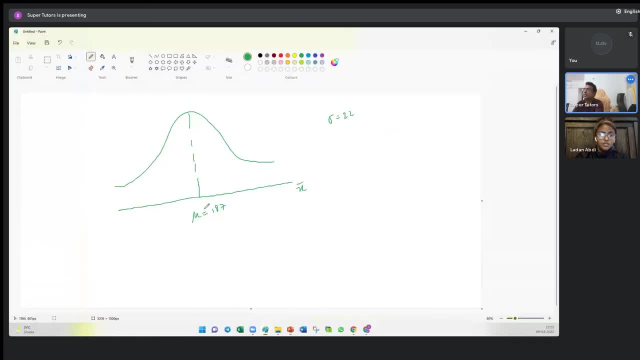 Blood pressures, The mean is 187. So if 187 is this number, 143 would be somewhere to the left of 187.. Yeah, The usual concept of number line where we say that the smaller number is always on the left of the larger number. 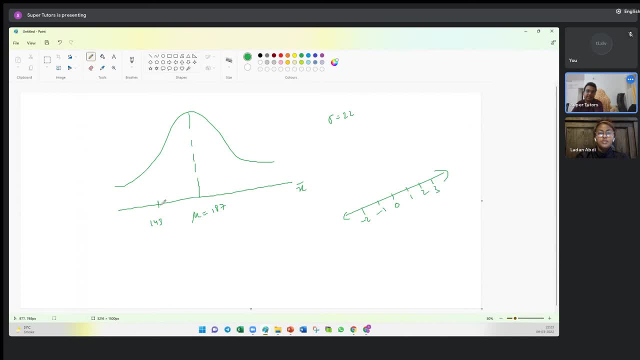 So if 187 is here, 143 would be somewhere on the left, maybe here. Maybe I can draw a dotted line also. Yeah, Yeah, And this is 143.. Mm, hmm, Similarly, what's the other number that we have? 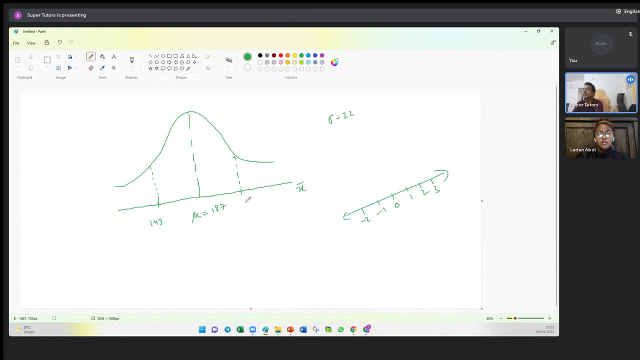 231.. So can I say that it would be somewhere here? Yes, Because it's positive. So you go that way. So I have to find what is the minimum value of the ratio of this green area to the total area under the curve. 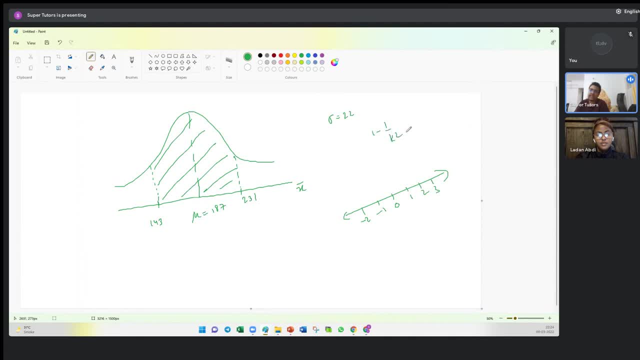 So basically I have to find 1 minus 1 by K square. So for that I need K. That's it, Yeah, Mm. hmm, So I want. this point is 187 and this point is 231.. So how many standard deviations am I going ahead? 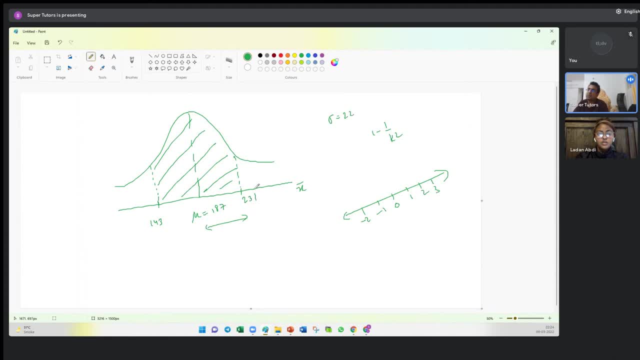 What do I multiply with my sigma to reach 231?. You subtract those two, Yeah, Yeah. So just use a simple formula. We know that this is represented as mu plus K sigma in the diagram. You remember that. So mu plus K times sigma is how much? 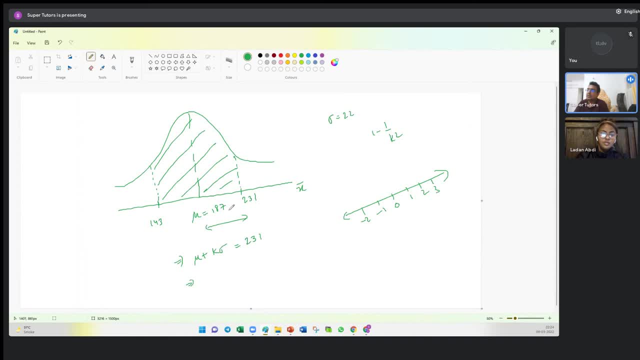 231.. Mm, hmm, What is the value of mu 187.. So 187 plus K multiplied with what is sigma 182.. Make sense, Mm, hmm. So can I say 22K is equal to 231 minus 187?. 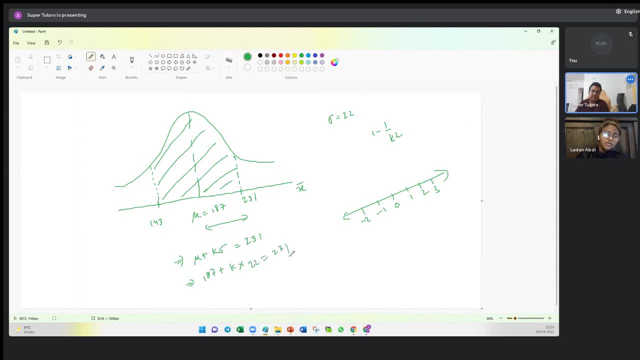 Just taking the 187 on the right hand side: Mm hmm. Yeah, It will come to 44 if you do the math. Mm hmm. So if you do the math, what is the value of mu 231.. Mm hmm. 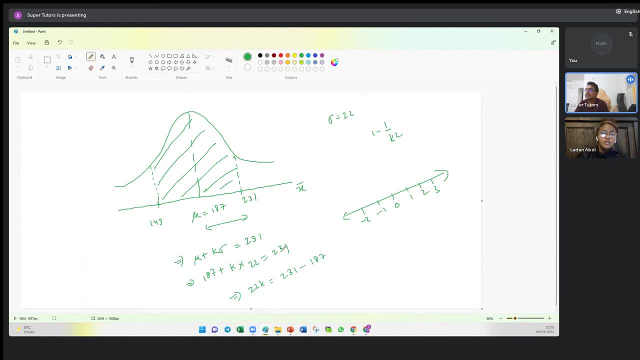 So what is the value of mu 231.. Mm, hmm, So what is the value of mu 231.. So what is the value of mu 231.. Mm, hmm, So what is the value of mu 231.? 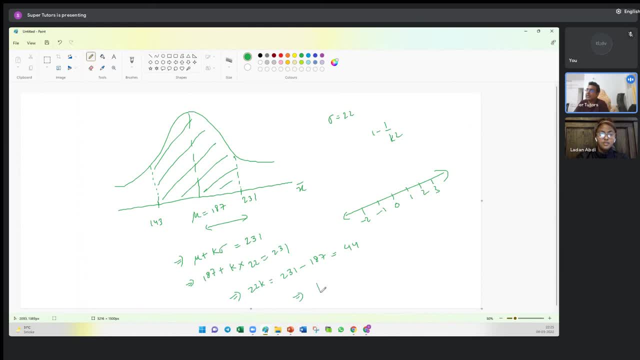 Mm, hmm, So if 22 times something is 44, then can I say that is nothing but 44 divided by 22? Something multiplied to something, when it comes on the right hand side, becomes division. Mm, hmm, What is that? 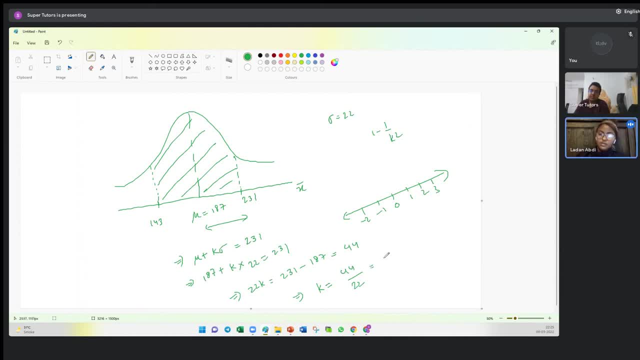 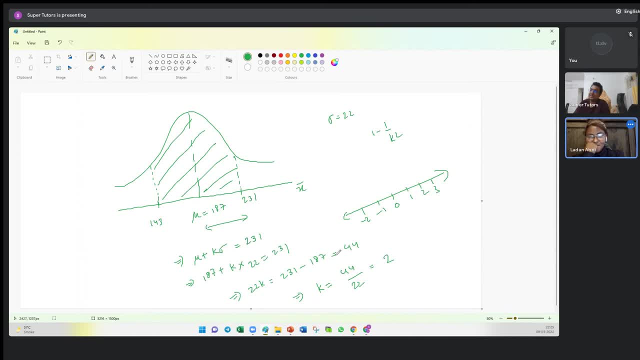 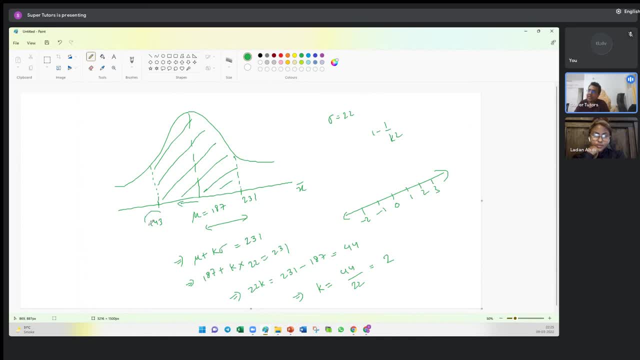 That's my rule for Chebyshev's Mm. hmm, So we need to verify for 143 also, Right, Yes, So 187,, which is mu minus two times of sigma, should give me 143.. Right, Where are you getting the two times from? 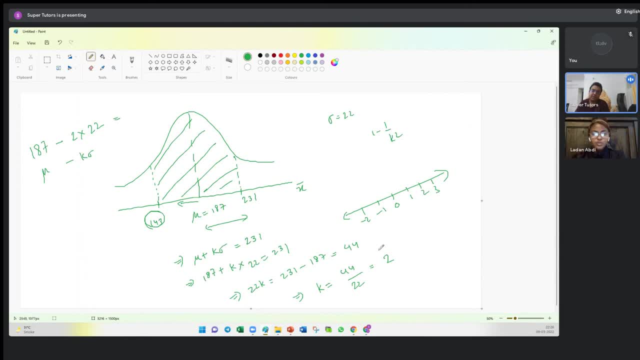 Right. Oh yeah, That's a. I am just verifying whether K is actually two or not. So the K is we just found here. This is nothing but mu minus K times sigma, Right, Mm? hmm. So for Chebyshev's to work, the value of K should remain consistent between this and. 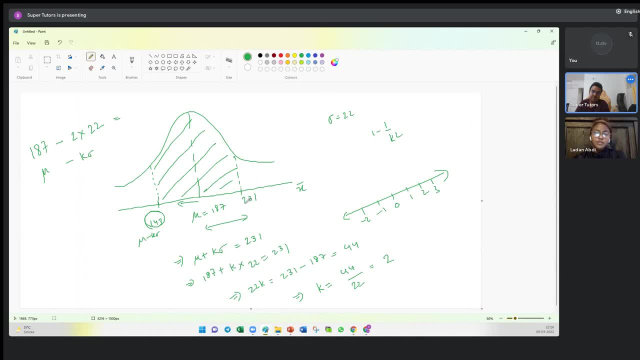 this Right: Mm. hmm. If you subtract K times the standard deviation from this number, you should get this number. Yeah, If you add K times the standard deviation, you should get this number: Mm. hmm. So we calculated K using this number. 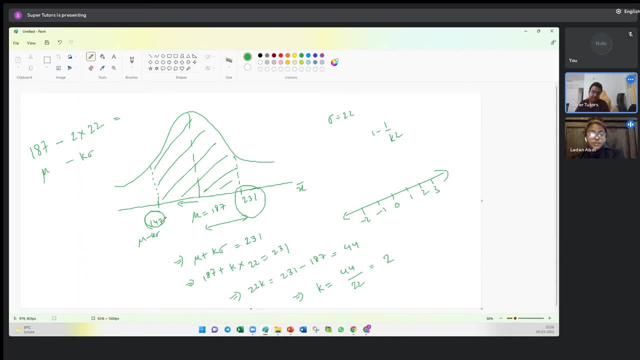 Now we're just checking whether this is also true, Mm. hmm, Okay, So 187 minus two times of sigma. Can you do the math? Tell me what it comes to? 44. Yeah, 44. No, no. 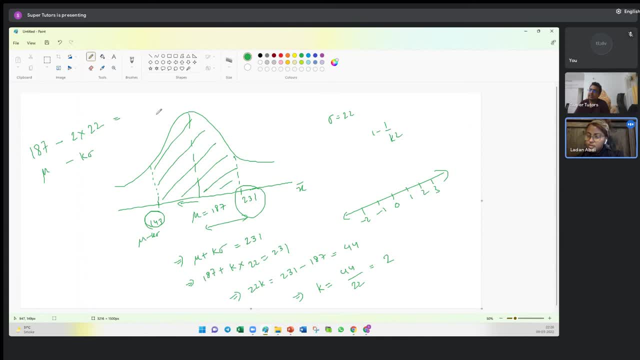 187 minus the whole thing, The whole thing. What does it come to? Oh, 187 minus 44.. 143.. Is that the number we have here? Yes, So now we have K minus 2.. Yes, So 187 minus 2 times of sigma. 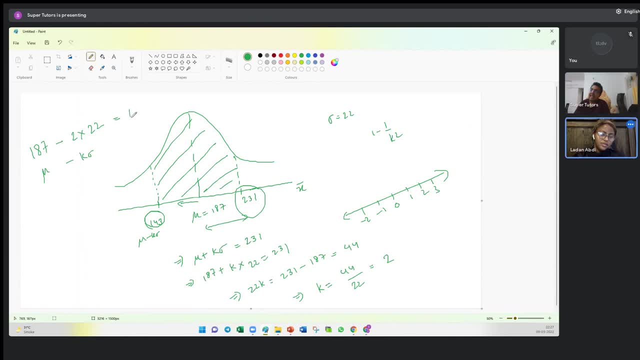 Right, Yes, So 187 minus 2 times of sigma, Right, Yeah, So 187 minus 2 times of sigma, Yeah, Yeah, That's right. So 187 minus 2 times of sigma, Yeah, Yeah, So now we are able to confirm that K is 2.. 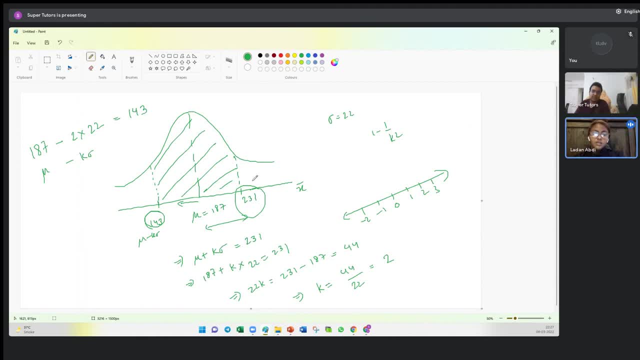 Yes or no? Yes, So 1 minus 1 by K square, 1 minus 1 by 2 square Mm, hmm, Which is nothing but 1 minus 1 upon 4, which is 3 fourth, or 0.75 or 75 percent. 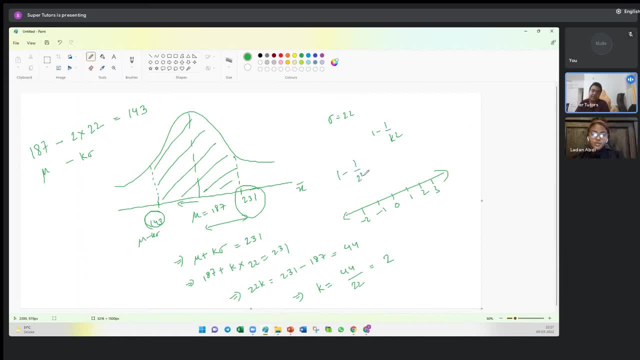 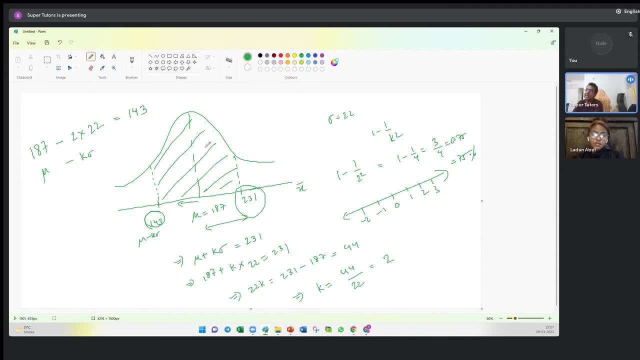 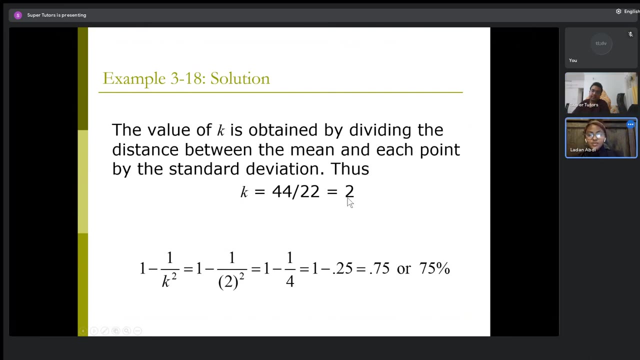 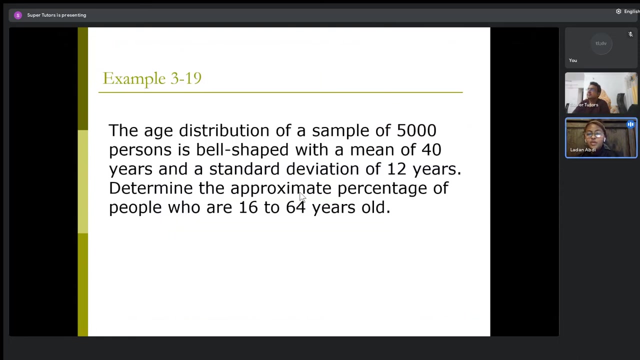 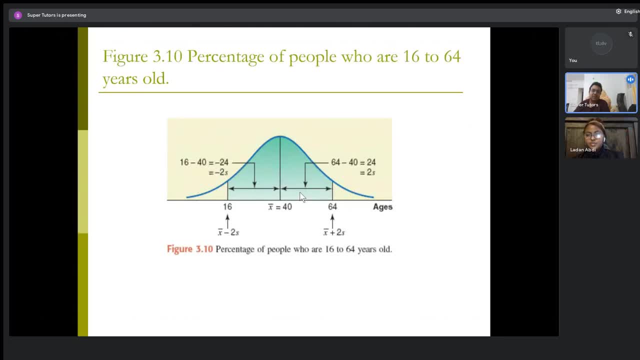 Okay, Okay, Yeah, Okay. When we deal with such using a variable in terms of 2 to infinity torment, we are using theнизArif value. in the만imal examples we have discussed Honestyri, Honestyri. So that is all to ChubbyShell. 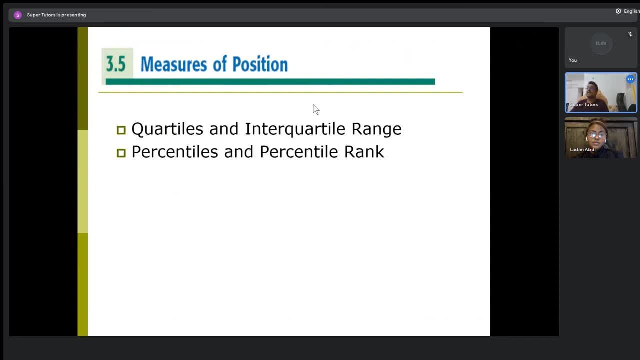 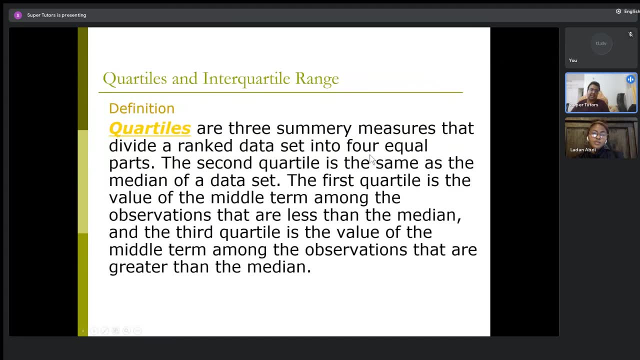 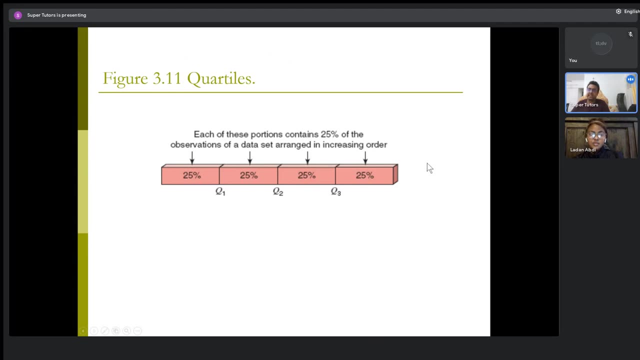 That's it. concepts in your chapter 3 talk about quartiles and percentiles. so quartiles essentially are summary measures to divide a rank data set into four equal parts. so if i have a rank data set just arranged in increasing order, i can divide it into four equal parts of 25. 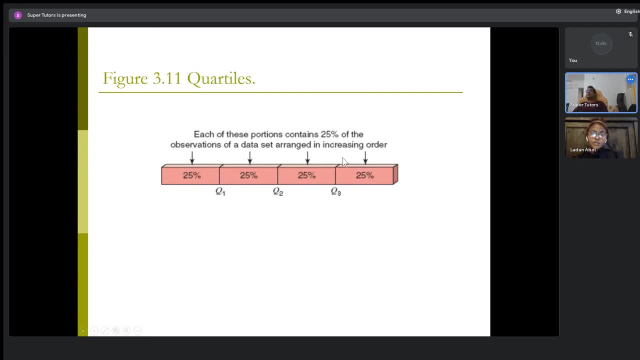 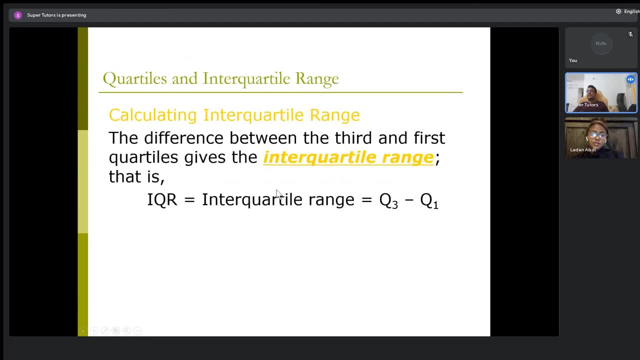 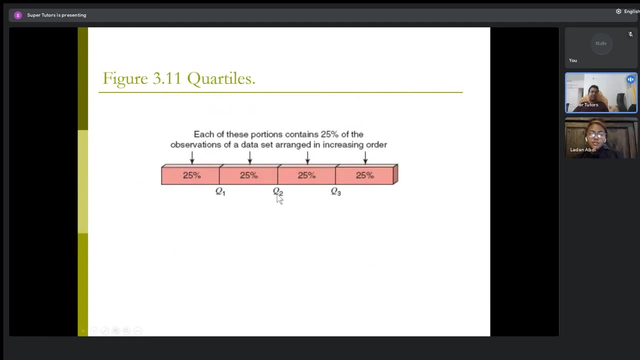 percent of data, each using three quartiles: q1, q2 and q3. that makes sense. so the second quartile is always the median right. yes, this is always the median, the same thing that we studied earlier in this chapter, and q1 and q3 are calculated as we will go. 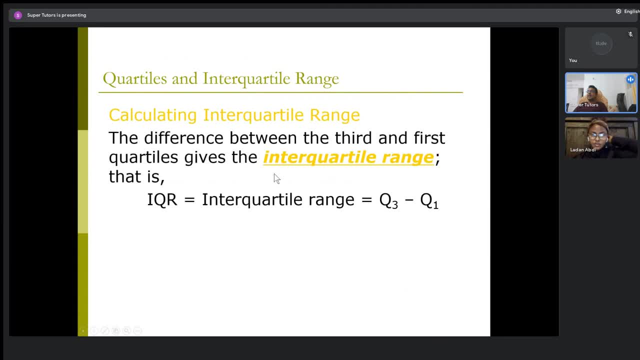 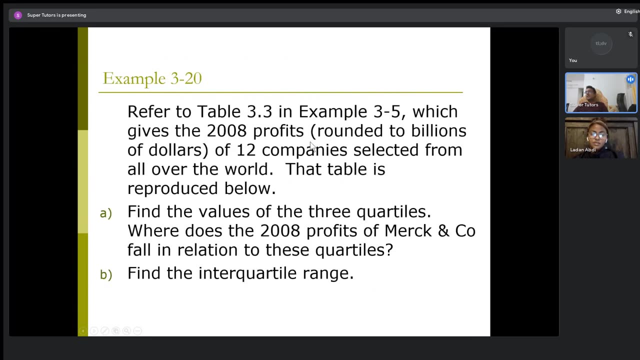 through in future slides. meanwhile, one intermittent concept for you is interquartile range iqr, and that is nothing but q3 minus q1. that's it. you find the two and you subtract q1 from q3. that's it. that's all you do. so let's see an example and try to understand how we calculate. 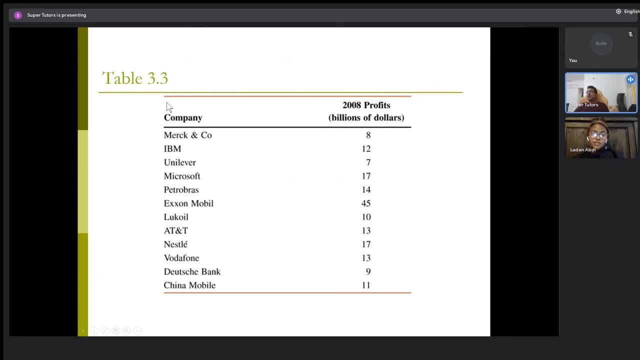 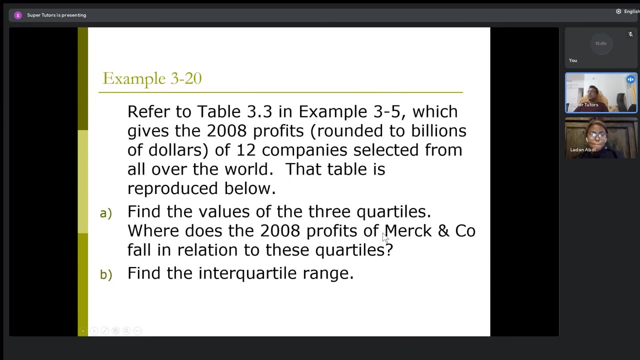 the three quartiles, right? do you remember this example we took earlier? 2008 profits of 12 different companies, right? the question is: first question: why the value of the three quartiles, right? where does the 2008 profit come from iqr and q3? why these profits of merk and co fall in relation to these quartiles, so how? 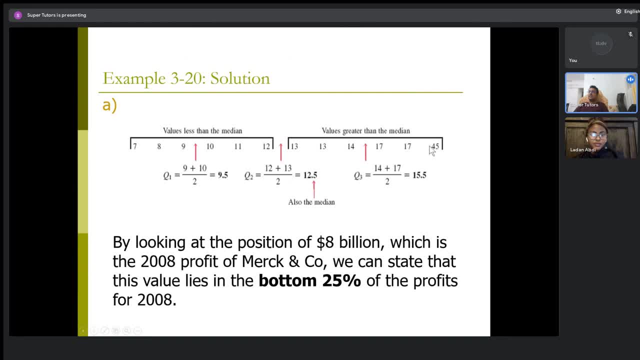 do you find the three quartiles very simple. first arrange them in increasing order. then the second quartile is the same thing as the median, as i told you. so, if you remember, median was middle, two values averaged, because there are 12 values here, so even number of value. 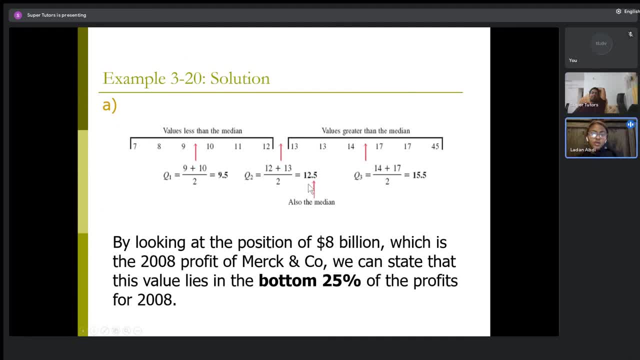 so what is 12 plus 13 divided by 2, 12.5 absolutely? and then you are after the example, you get earthquake come in and you have the hayat amount, right, right. so what is 12 plus 13 divided by 2, 12.5 absolutely? and then you are able to calculate in different ways the average. 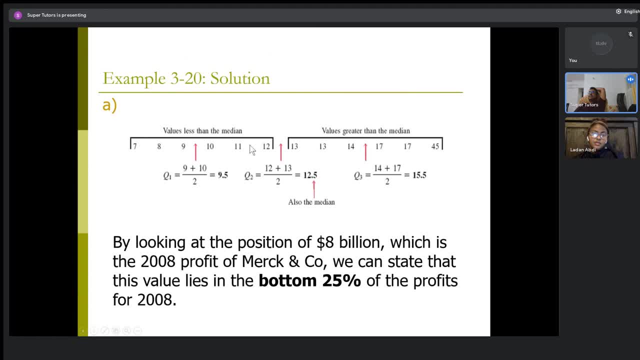 quantity of the quartile and the median, the average quantity of the quartile. okay, so this left with six values on this side and six values on this side. so out of these six, also you average the third and fourth, which is 14, and 17 out of this. 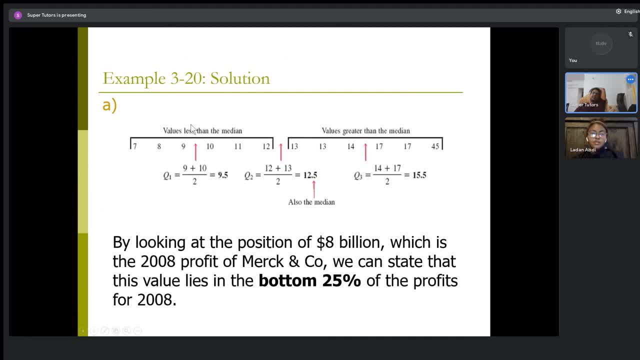 six. you average the middle two, which is nine and ten, if that makes sense. so by looking at the position of eight billion dollars, which is the 2008 profits of Merck & Co, we can state that this values lie in the bottom 25 percent of the. 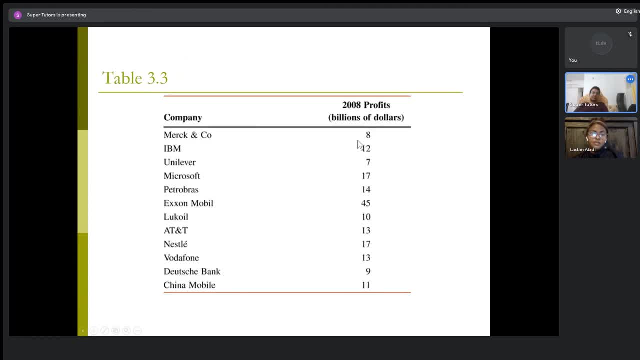 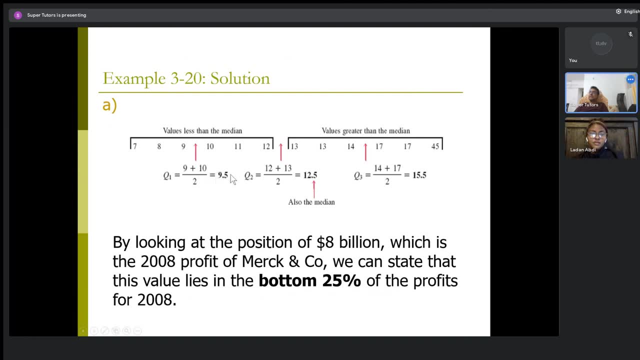 profits. so Merck & Co is eight, so it is below nine, point five: yes, because if you notice, q1, q2 and q3 are arranged in increasing order, always because these are the medians for a ranked dataset. so if q1 is nine, point five: if you look at 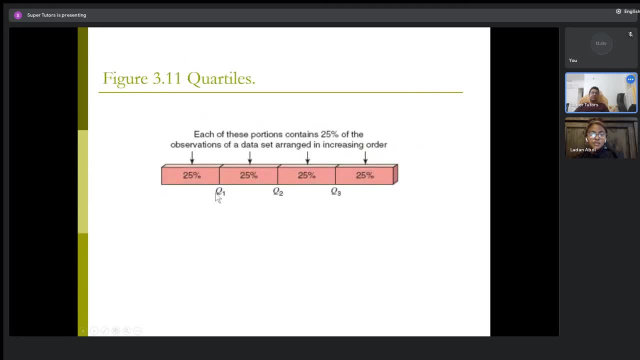 this diagram here is 9.5, then 8 would fall somewhere here. so that's bottom 25. yeah, if something falls here, then you say it falls between q1 and q2. you don't say top 25 or something like that. this is bottom 25, between q1 and q2, between q2 and q3. top 25. 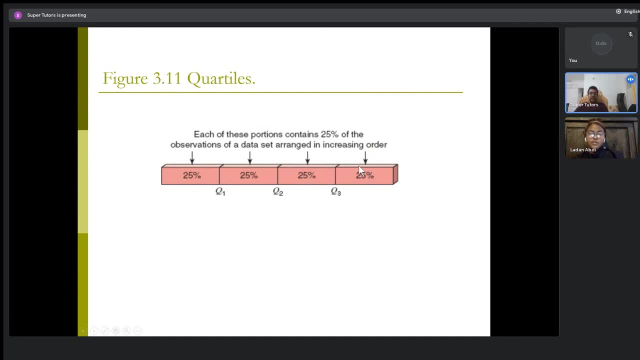 percent. that's how you speak in terms of cortex. so this one is top 25. this one is top 25, this one, okay, top 25, bottom 25. between q2 and q3. you clearly see q2 on one side and q3 on the other. so this is between q2 and q3, this is between q1 and q2 and this is bottom 25. 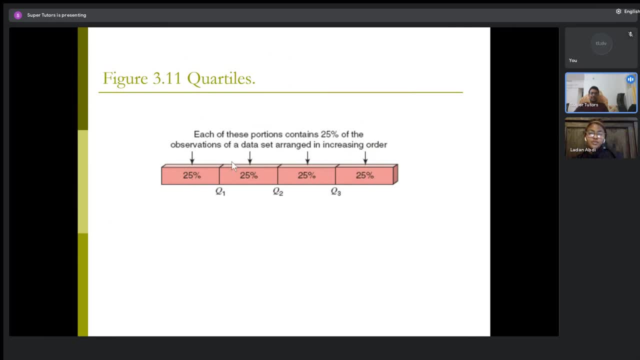 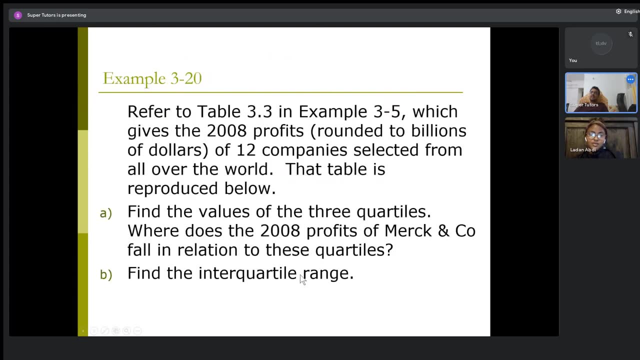 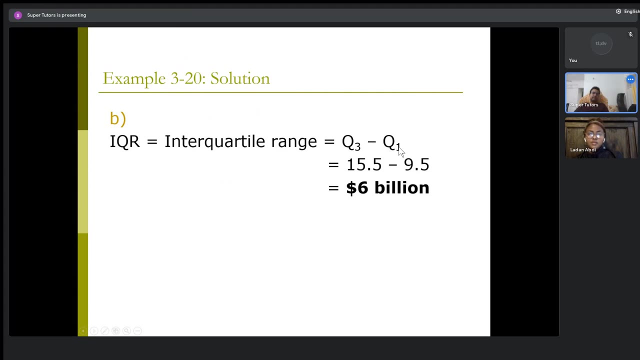 any questions. does it make sense? yes, absolutely yes, very clear, perfect. and last question is the simplest: find the interquartile range. so all you have to do is q3 minus q1, right? yes, percentiles and percentile rank. now, each of these portions contains one percent of the observations. 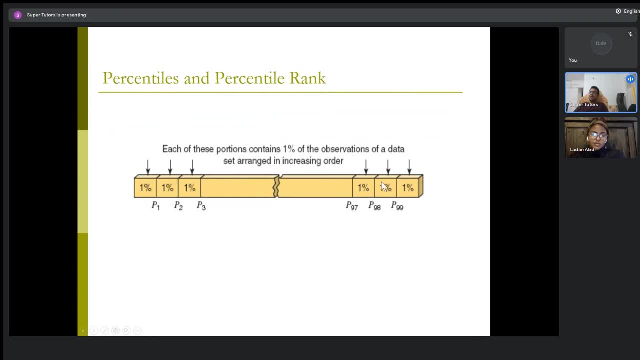 of a data set. similarly, in case of percentiles, we divide the data into 100 equal parts. quartiles. four equal parts: 25 percent each. percentiles. 100 equal parts: one percent each- the first part. so in order to cut a cake into 100 parts, you need 99 cuts. 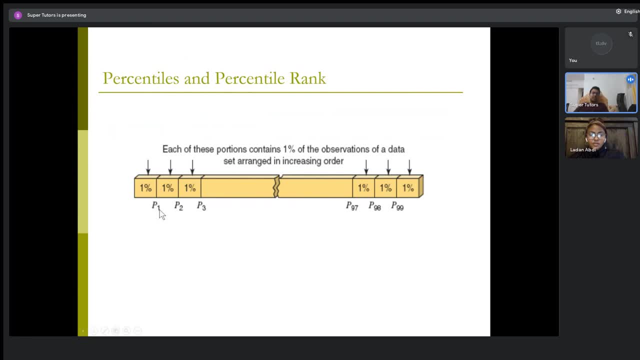 yeah, so the first cut is p1, percentile one percentile number one, p2, and hence the last one is p99. similarly, to cut a cake into four equal parts, you need three cuts: first cut q1. second cut q2. third cut q3. you understand the correlation between quartiles and percentiles. 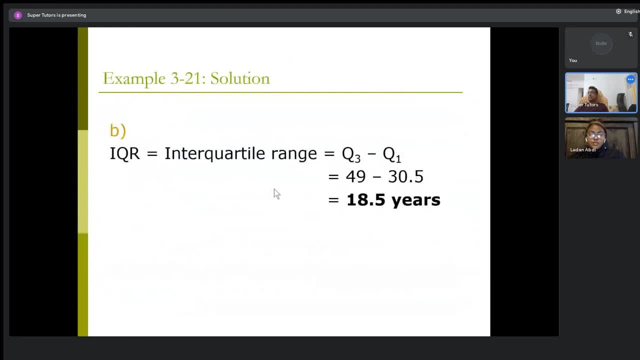 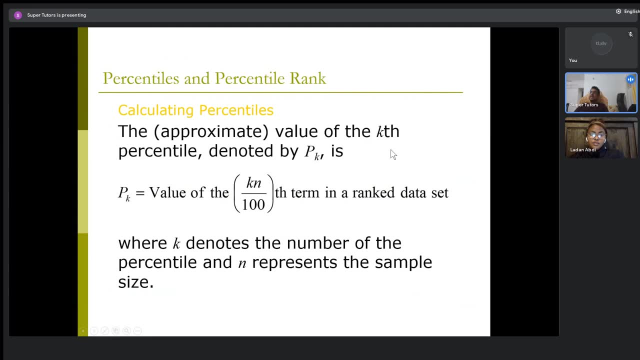 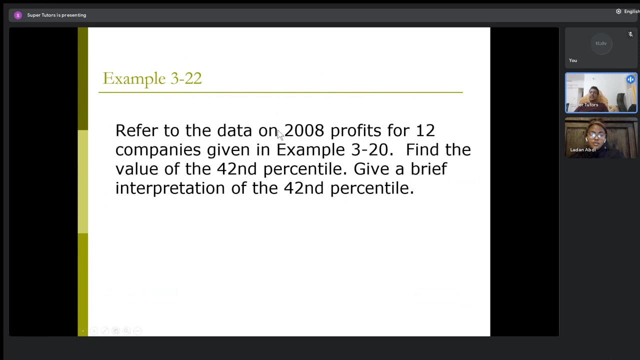 perfect. so how do you calculate the kth percentile? you simply grab the value of the kn upon hundredth term in a rank data set where k denotes the number of the percentile and n represents the sample size. right? so let's see an example. looking at the same data set, 2008 profits- find the value of the 42nd. 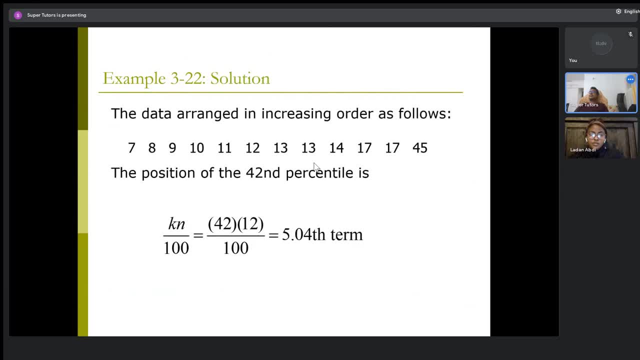 percentile. how do we do that? we first arrange it in increasing order and then i have to grab the kn upon hundredths term. where k is 42. it stands for what sorry the n is done for what n is the sample size? i was just coming to that. 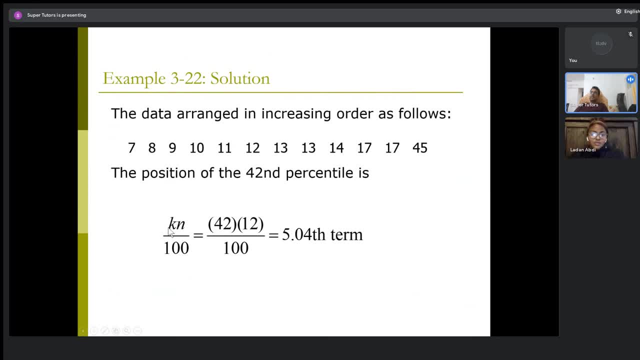 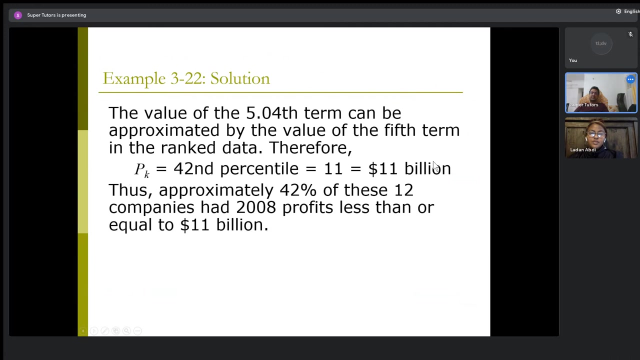 oh okay, sorry. yeah, so 42nd percentile is what i'm looking for. so k is 42 times the 12 values here. so 42 times 12 divided by 100, equal to fifth term. what's the fifth term in this data set? the 12 number, 12, 11.. fifth term: right, one, two. oh yeah, so 11 is my 42nd percentile. 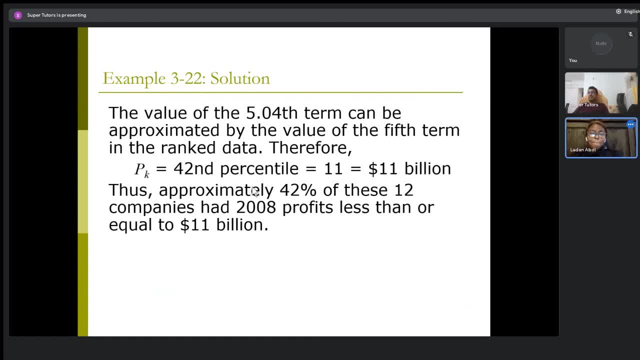 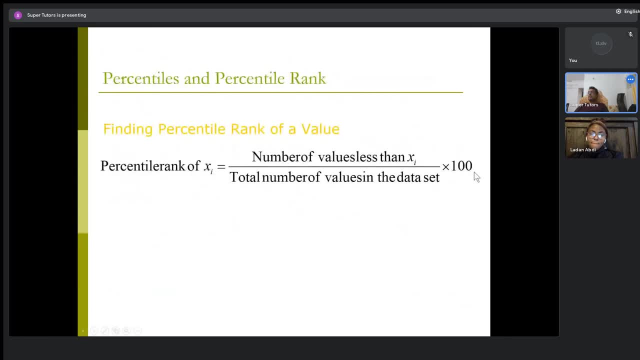 make sense. yes, it's pretty good too. yeah, and then we have something called percentile rank. so percentile rank is nothing but number of values less than x. percentile rank of x is nothing but number of values less than x upon total number of values in the data set times 100. 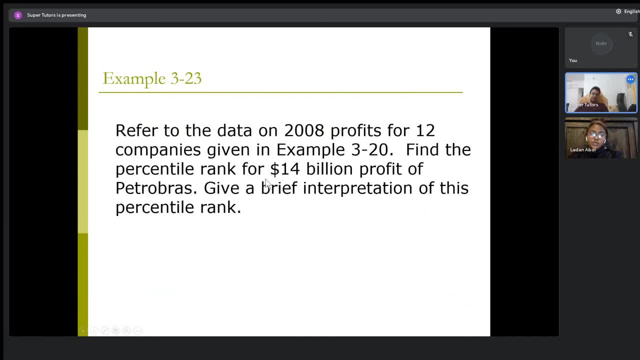 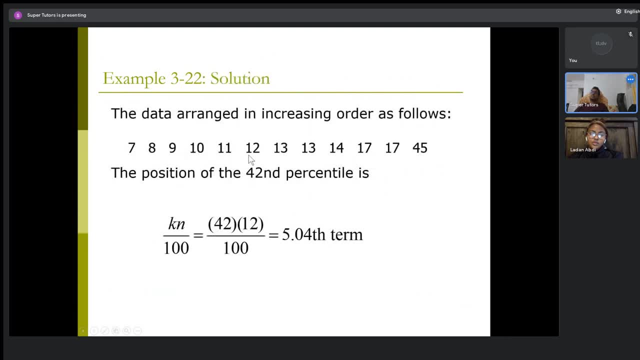 so find the rank of 14 billion dollar. mmhmm, so how many values should be there for f? and then find the rank of 14 billion dollar. so how many values it gets. let me show you this one: values. do you see less than 14? all of these values, if you count carefully. how many do you see here? 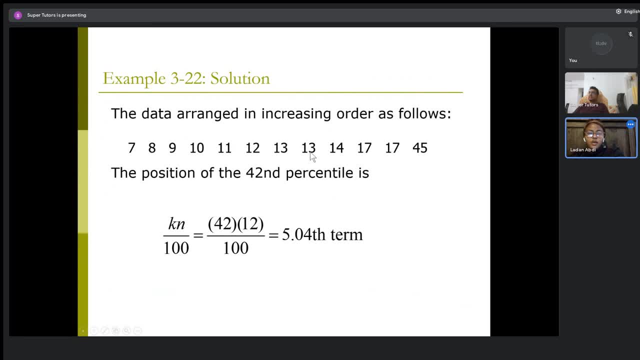 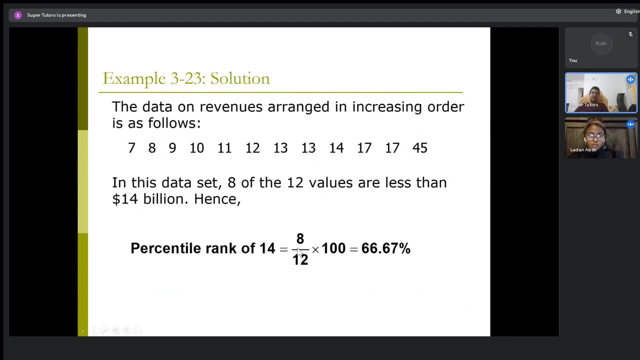 from 7 to this: 13, 8, 8. so number of values less than 14 is 8 divided by total number of values, which is how much 12 multiplied with 100. so 66.67 percent is the percentile rank of this 14. 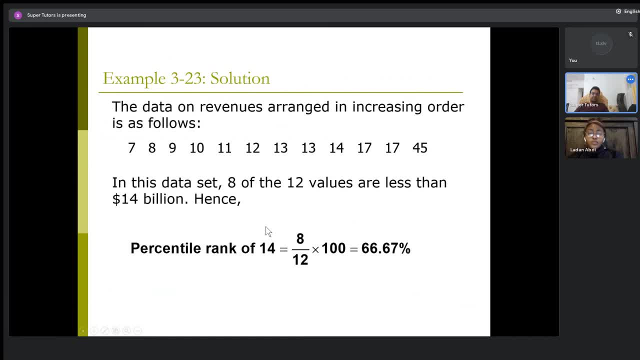 oh, okay, straightforward. that's the reason that i always say chapter one, two, three is free marks for everybody. and the good news is, from chapters one, two, three alone, you will have 40 percent of the questions. 40 percent, 40 percent of the questions from the exam, just for chapters one. 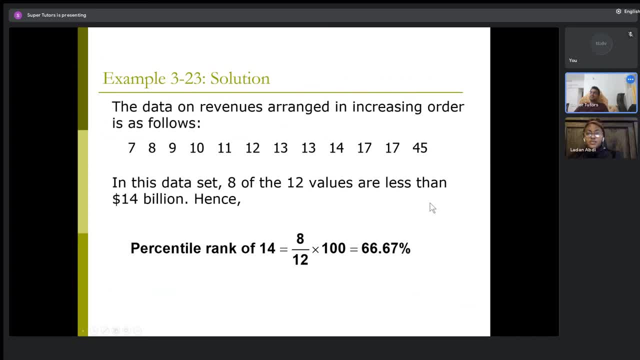 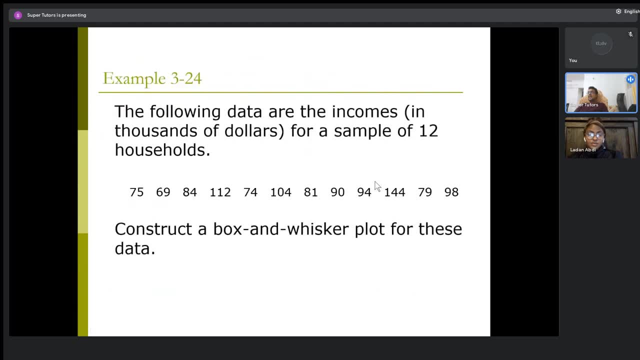 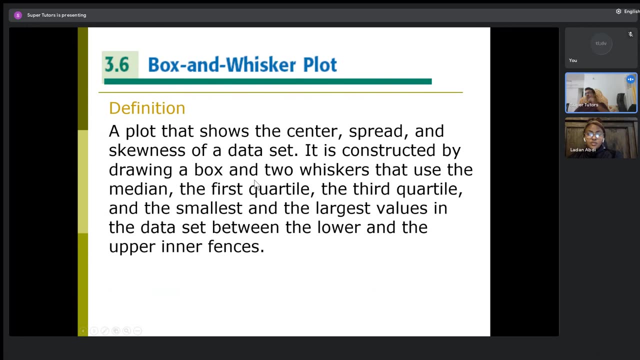 two, three. that's amazing, right? so this is how you find the percentile rank: mm-hmm. and the last one is about a box and whisker plot. now, you might not get the construction of it in the exam, because that is of course not possible, but you might have one or two questions from here. 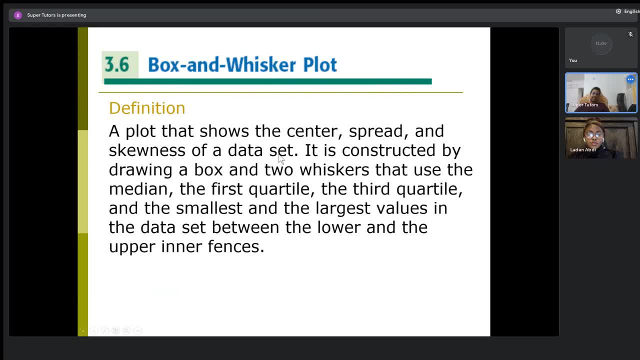 so this is a plot that shows the center, spread and skewness of a data set. it is, as the name suggests, box and whisker. so you construct a box, you draw two whiskers that use the median, the first quartile, the third quartile and the smallest and largest values. 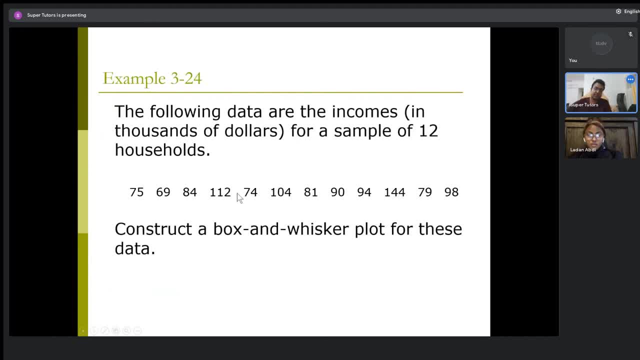 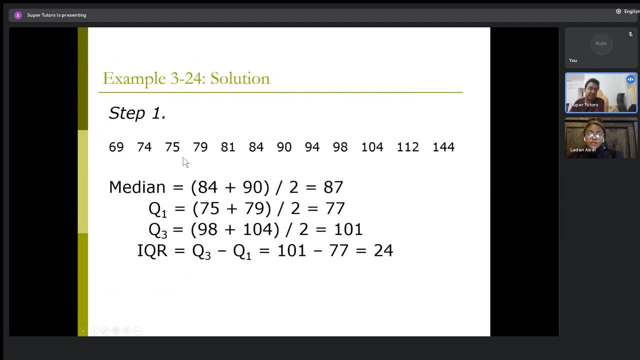 and then go from there, simple construct a box and whisker plot for this data. you have all of this data here, right? yes, how do you construct it? you first arrange it in increasing order. then you find all of these numbers: median. you know how to find median by now. yeah, q1, q3, iqr. 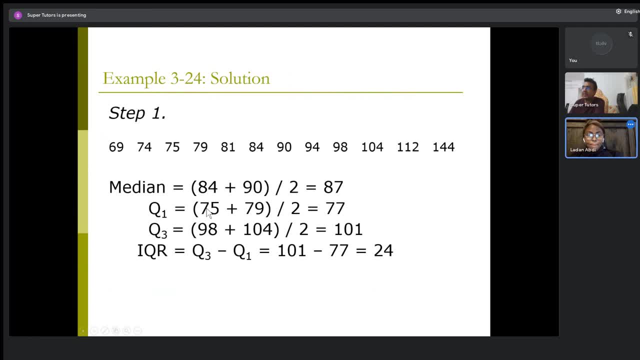 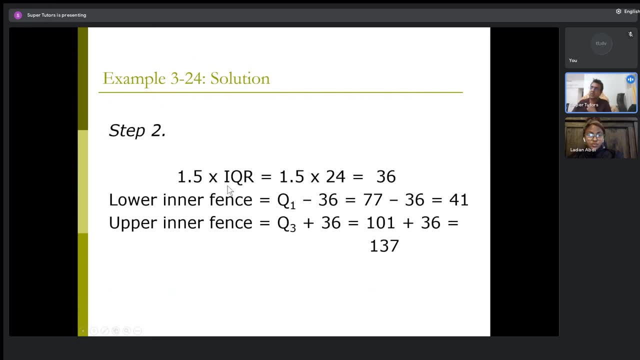 clear: yeah, just go on. yeah, yeah, yeah. and then you go from there, and then you go from there, and then you go from there, and then you find these three quantities based off of the previous ones. so we find a special quantity which is nothing but 1.5 times your iqr. so our iqr came out to be 224. so 1.5 times that 24 gives us 36. 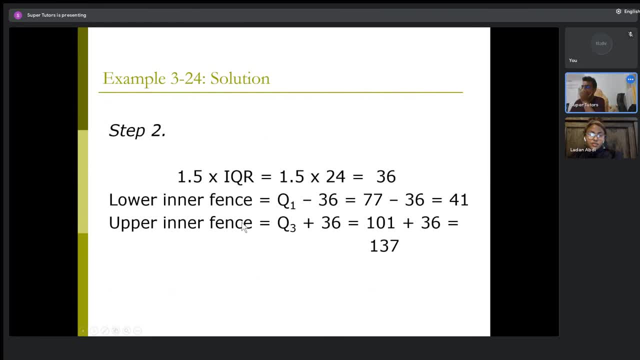 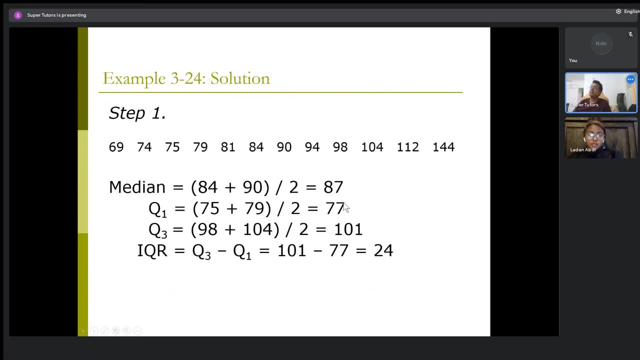 and then we calculate lower inner fence and upper interface. so lower in our fence is nothing but your q1, or your first quartile minus this number. okay, so what was your first quartile? coming to 77, 77 minus 36 gives us 41. upper inner fence means q3 plus this number. so q3 plus 36, which? 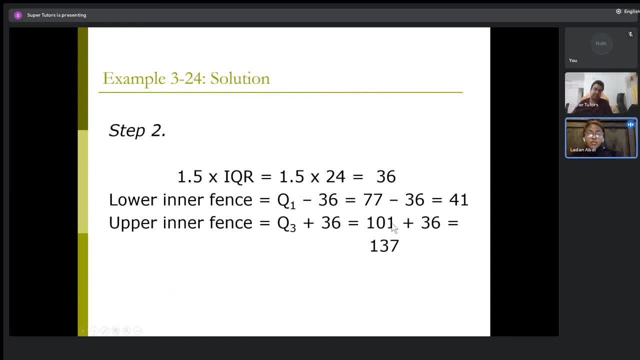 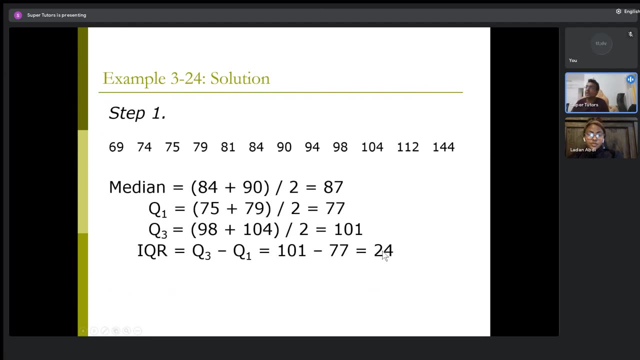 gives us 137, if that makes sense. yeah right, so smallest value within the two inner fences: 69. largest value within two inner fences: 1, 1, 12.. so what you do is these two fences, 41 and 137. now you look at the data and find the largest and smallest values within that range. 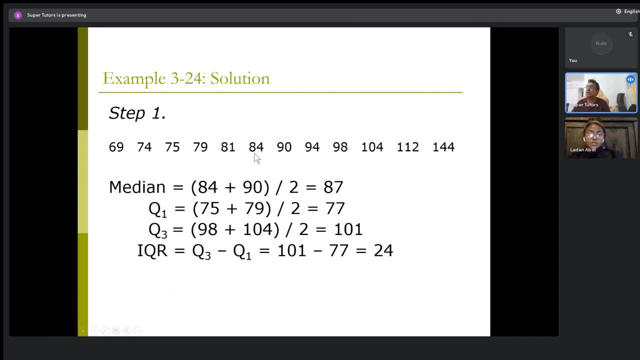 so if i get the rank data set for you, which is the smallest number between 41 and 137, 69 make sense, so i say that again. so just remember these two numbers: 41 and 137. yes, okay, between 41 and 137. out of the numbers that you see here, what is the smallest number within that range? 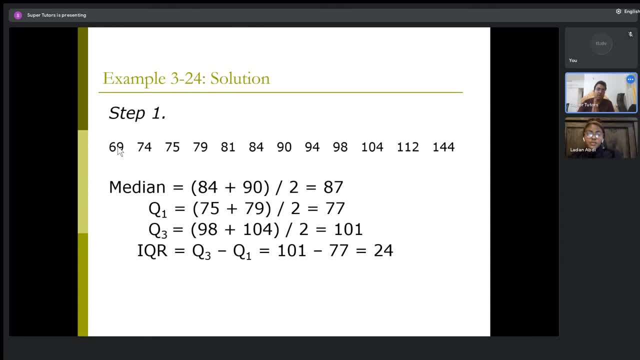 oh uh, 69, 69 within 41 and 137. what is the largest number on this slide? 144 is 144 between 41 and 137. no 112.. 112.. so largest value within the two inner fences. these numbers are referred to as inner fences.